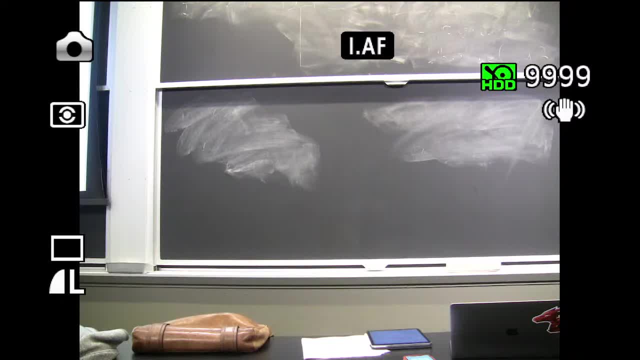 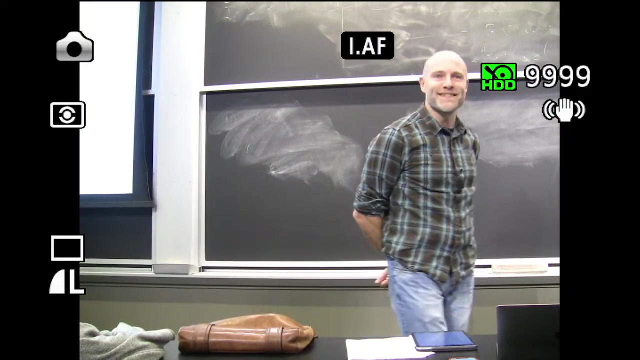 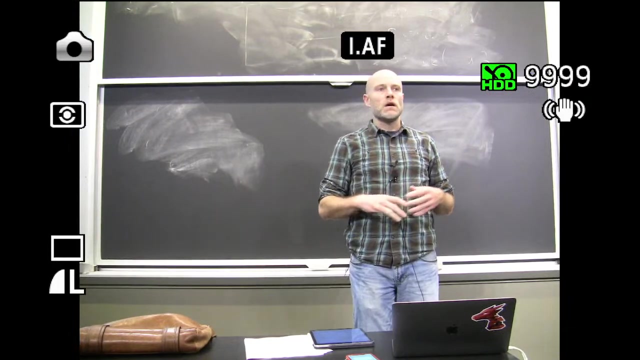 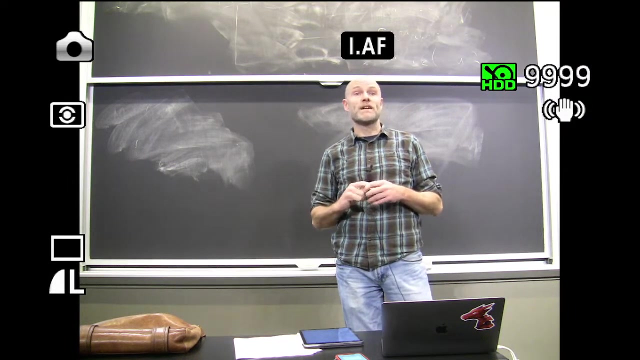 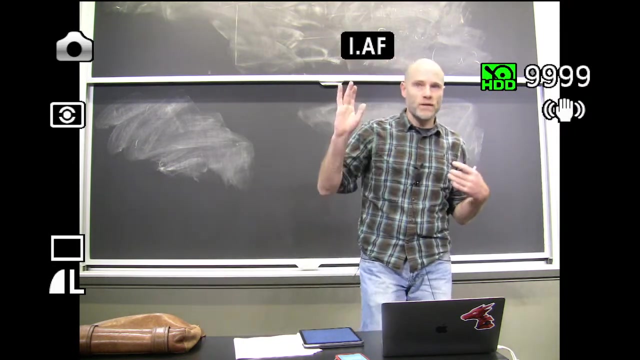 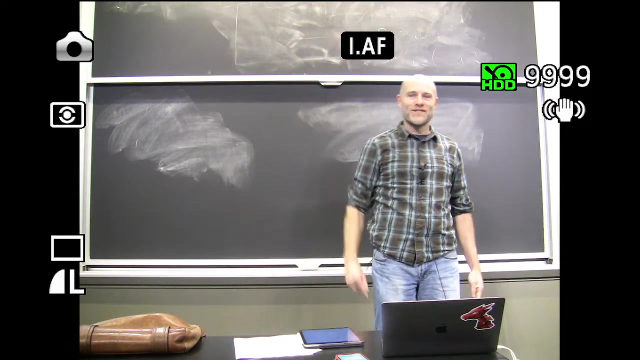 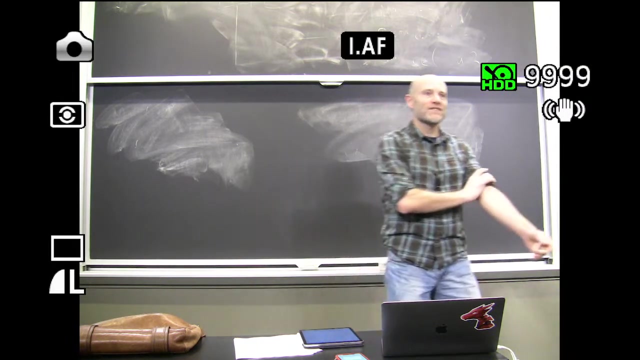 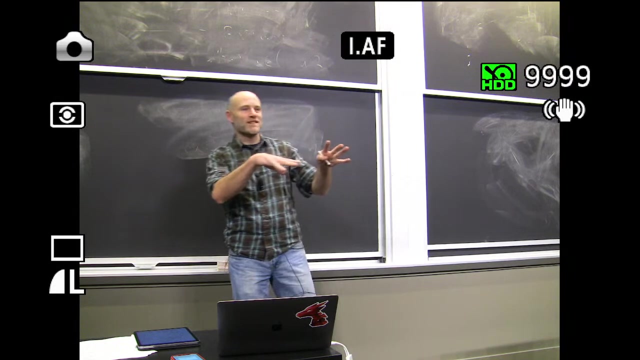 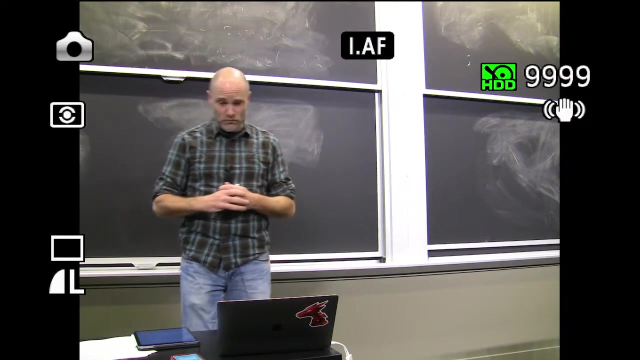 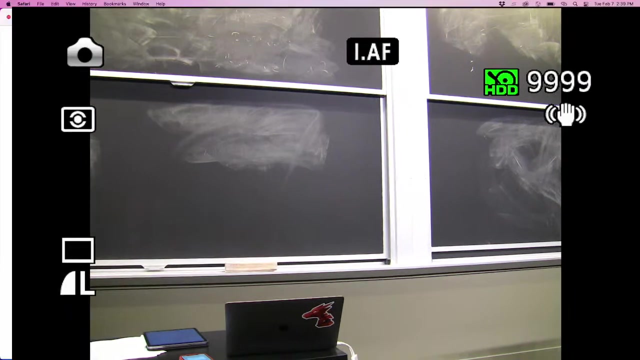 You good? Okay. All right. Hi, everybody. Good to see you. It's nice to see a nice full room. That's good. Yeah, so welcome to underactuated robotics. If you don't know what that word means, that's okay. We'll understand that by the end of the day today. But I think it's pretty clear we're going to try to make robots do things like that on the slide. So I'm going to try to do a couple things today. I want to give you some high-level motivation, but I also want to give you some of the initial derivations and definitions just to at least start thinking about robot dynamics, which is going to be a big theme throughout the course. So let me introduce quickly myself. So I'm Russ. I've been a professor here for a while now. The TAs here. So Richard, can you stand up and wave? Yeah. Richard Minnell is right here getting us on YouTube here. And Sun Bo-Chen is here. We have excellent TAs with a good diversity of experience, by the way. We have a couple people that are sort of RL experts, a couple people that are really experts in the model-based side of the world. I think it'll be a great term. So everything, all the course materials are going to be on the web. So there's no handouts. The grading policy, the collaboration policy, everything is on the web for you to... 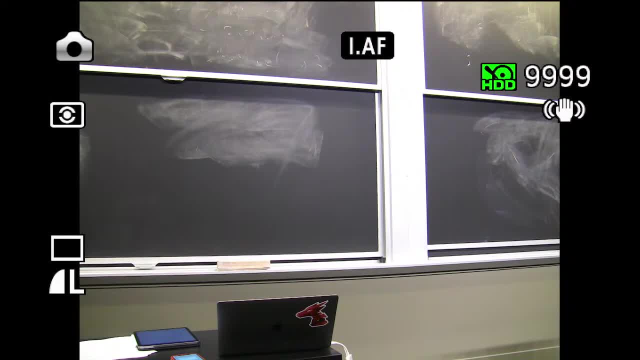 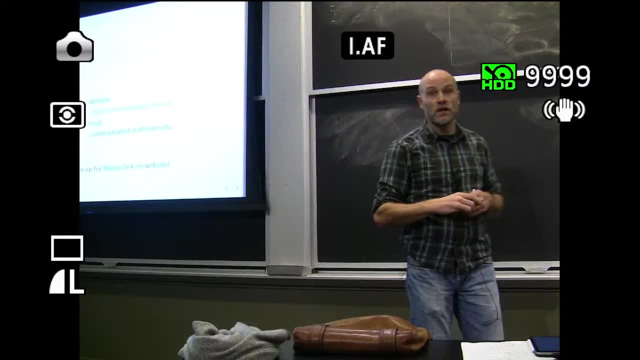 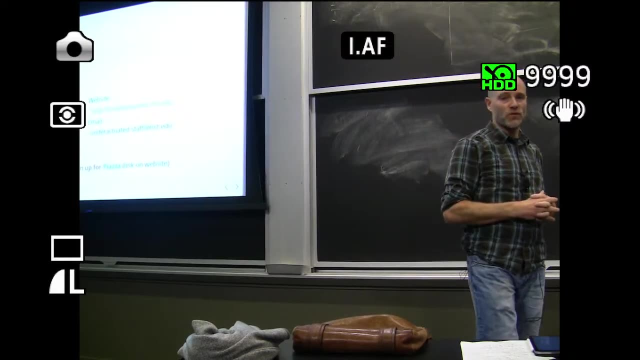 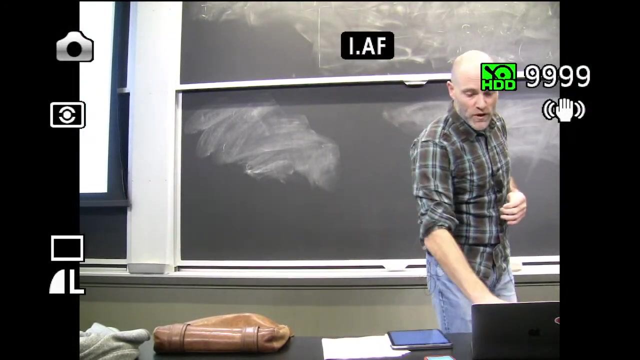 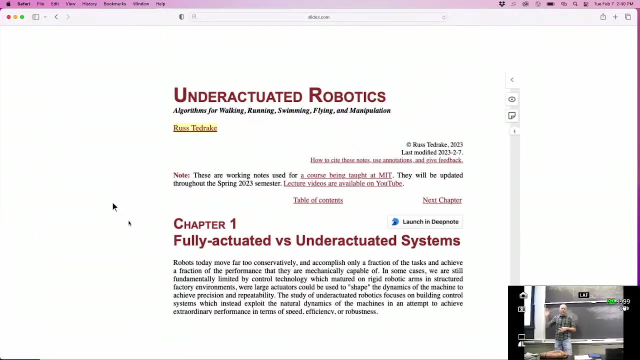 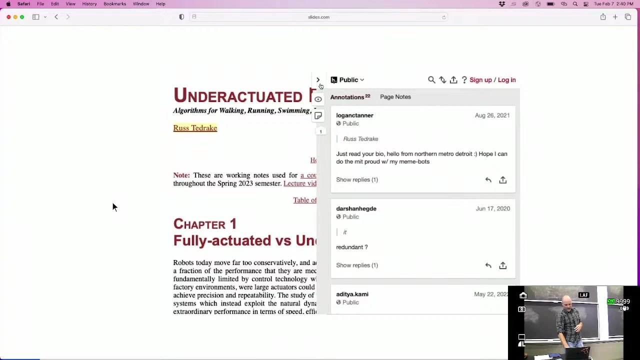 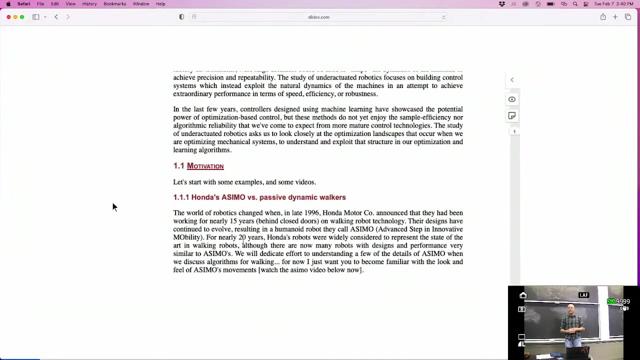 Find there. You can contact us with the email. And the one action item here for you is please go ahead and sign up for Piazza. There's a link on the main class website. And then hopefully your MIT credentials will just get you right through. If you have any trouble, email the staff and we'll make sure we approve your Piazza. When you go to underactuated.mit, what you'll see is actually the course notes, right? So I've been trying to... Write notes now in raw HTML because then I can put in all kinds of dynamic content. You'll see simulations and other links to code that are right in the notes. So I prefer that to PDF these days. Although some people prefer PDF if you... I make it available at the end of every term. So there's a last semester's version is locked in as a PDF, but I'm gonna keep updating the notes online. And please consider using the dynamic version. You can also comment. We can have a little discussion on the dynamic version. People ask questions about like where I grew up and stuff, which was just because that's the first page. But if you have technical questions or whatever, you can highlight, you can make notes to yourself, or you can make public notes and I'll try to answer there too. 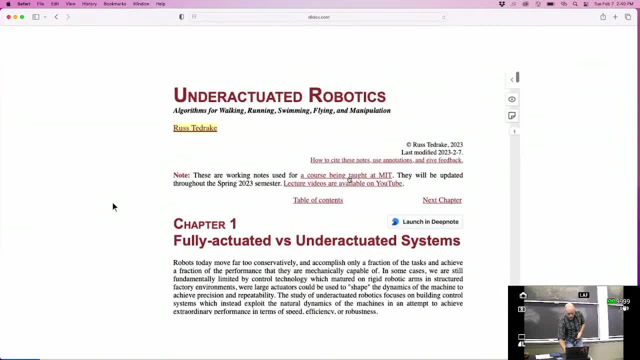 And it's a nice way to have a discussion. If you do click on the course being taught, that'll take you to the semester's course website, which has the calendar and everything like that. 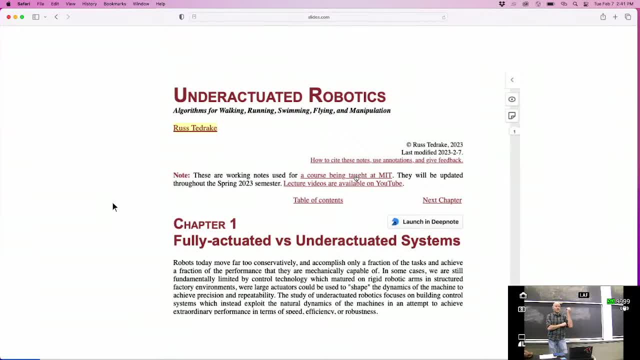 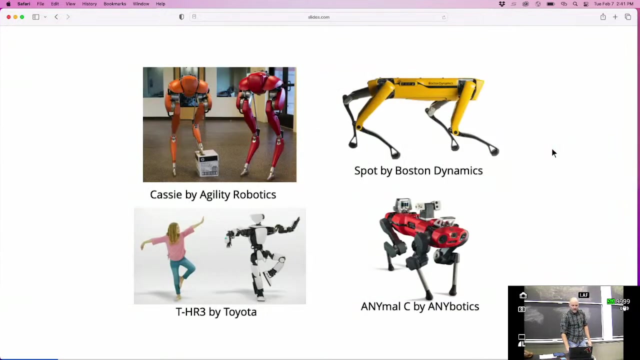 Okay. So let's talk about robots. You guys realize I guess you're here because, you know, we're kind of in the golden age of robotics. Things got really, really good. You guys are so well-timed. You're so lucky to be like in the field, coming into the field right now. Things happened dramatically over the last few years. There's never been a better time, right? We have... What we've seen actually, it's the result of many different things. Certainly people know about the machine learning revolution and how that has enabled computer vision, which makes our robotics applications dramatically more ambitious, right? We now, we have large language models. You can ask chat GPT what your robot should be doing. That's huge. That is, we've never had something like that that could give us somehow a common sense backend for robotics. The things we can do with robots now because of those kinds of technologies are fantastic. The other thing that's been happening behind the scenes is that there's been a significant increase in the number of robots that have been sustained funding of robotic hardware over the last, you know, two decades even that have gotten our hardware just better and better and better until they just broke out of the lab. And the 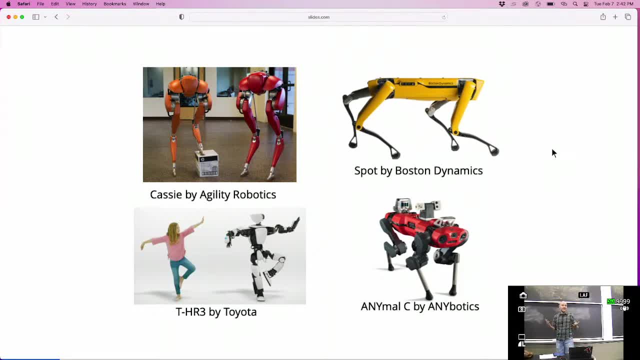 robots you see here are some of the most fun examples of that where we see now bipeds or quadrupeds. You might have seen them running around campus. You can buy a quadruped, a very 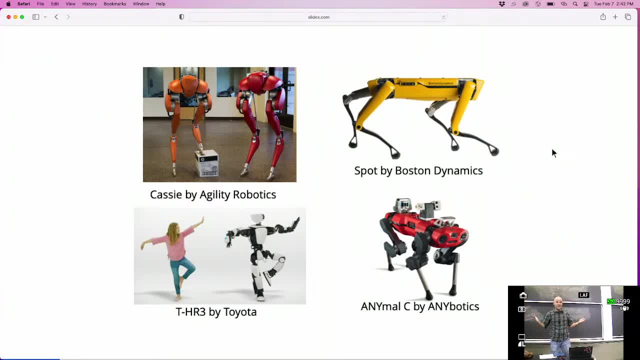 capable quadruped for two grand now with a GPU inside. That's insane, right? 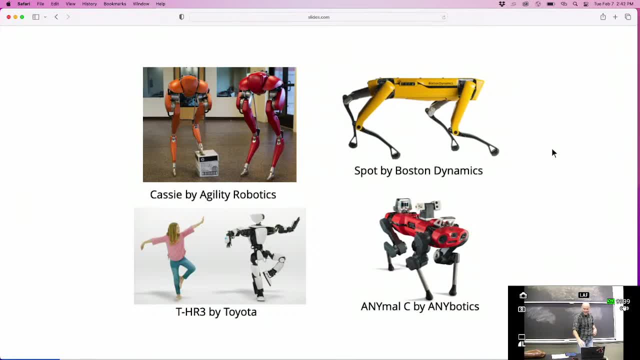 And there's extremely high-end robots like one of my favorites, right? If you want dancing robots. 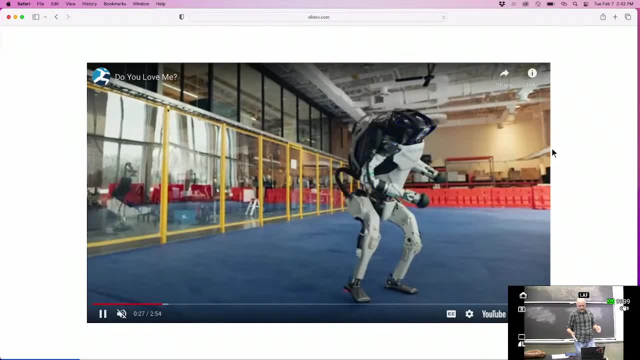 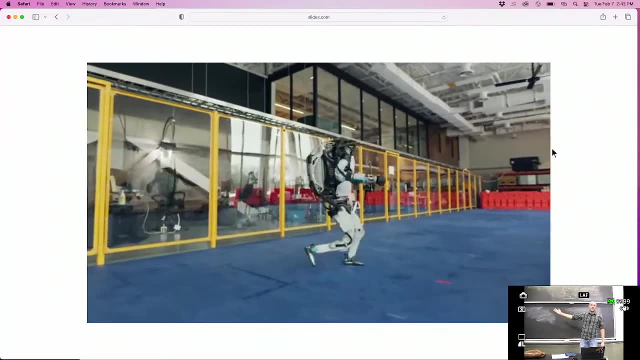 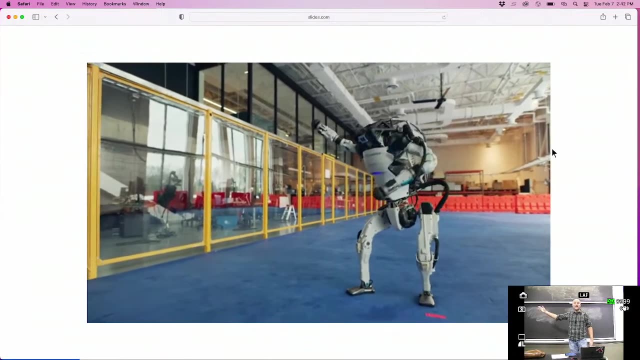 Oh, by the way, the network in here turns out is bad, so I'm powering this off my phone, which is awesome. But yeah, so this kind of hardware just didn't exist a few years ago. I had an early version, I do have an early version of this robot in my lab, but it weighed 400 pounds and it could not do this. Continued investment in hardware and some really, really talented hardware 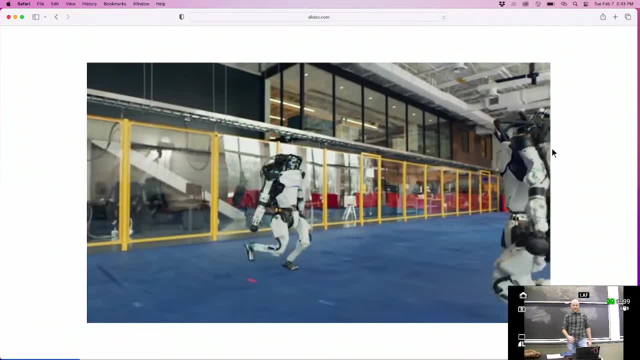 engineers. Gives us robots that can do this and backflips and all the other things you've seen. 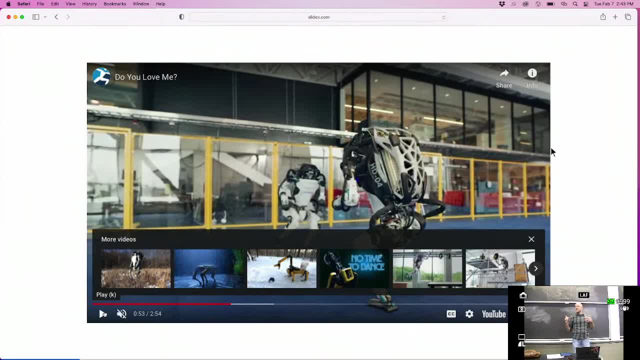 Right? So all these things have combined to be this just amazing time to be doing robotics. 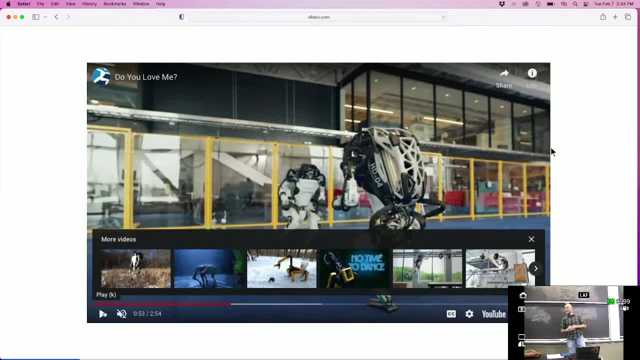 So when I talk about underactuated robotics, which we'll define carefully in a few minutes, what we're talking about really is of all these different components of intelligence, perception is one component with computer vision. The large language models is sort of another component. What I'm talking about in underactuated robotics is kind of is what Mark Raybert, who you'll see in these videos, for instance, calls athletic intelligence, right? So this is about the dynamics and control of our robots. And we'll touch base on some fundamental ideas from dynamics, dynamical systems theory from control. I'll go through some of the background in a second. So think about being in this course to learn about how to make the control system, the athletic intelligence that can power robots like this. 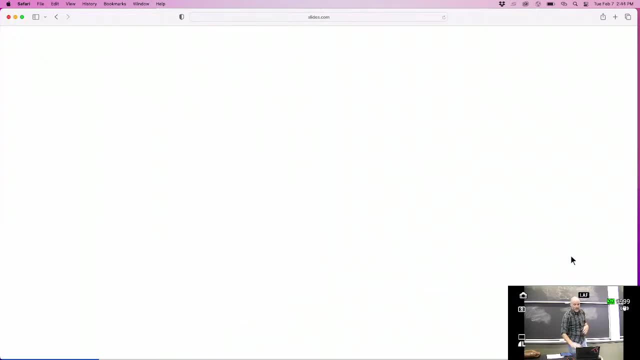 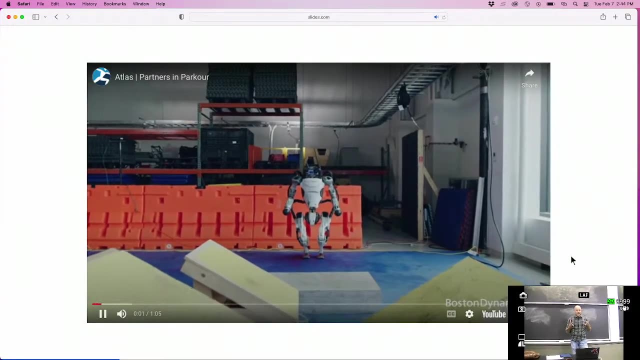 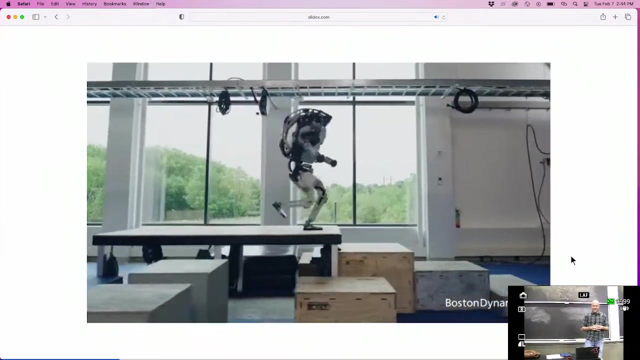 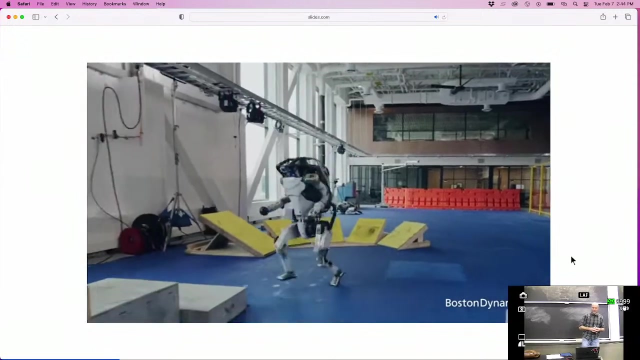 So there's a few great examples of, I think, underactuated robotics. So that's maybe I'll first define it just by examples, right? So of course, Atlas doing stuff like this. This is athletic intelligence, you know, embodied, right? The parkour course or the Ninja Warrior, I guess, is that first, right? This is just awesome. I know you've all seen it, but it's so good that I'm going to make you watch it just one more time here, right? It's just absolutely insane. 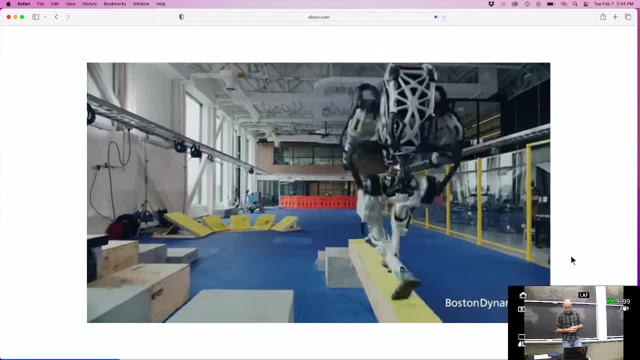 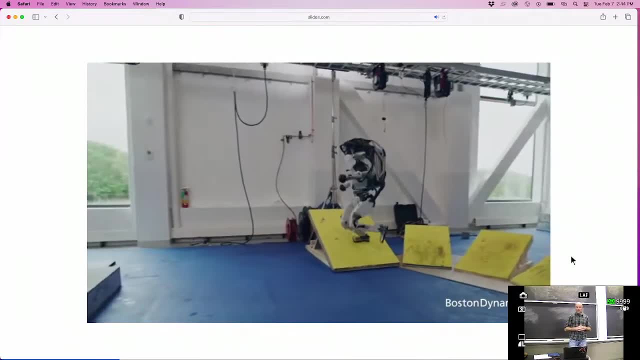 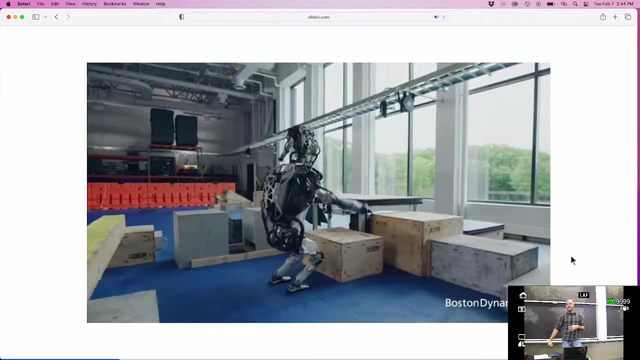 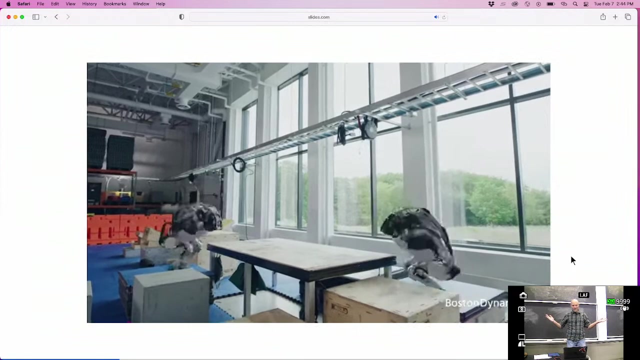 How well this works, how well the hardware works. If you were to stop by Boston Dynamics, now they would run this demo with no problem. It's not a one-off in any way, shape, or form. That hand contact, that was a big deal. We tried to do that back in lab and it was very hard. They were very proud to do that. And then the backflip, oh, so good. 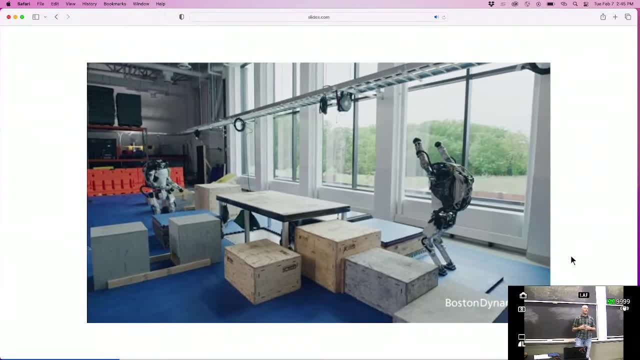 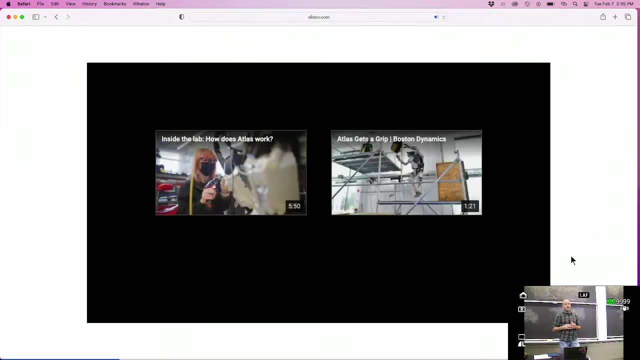 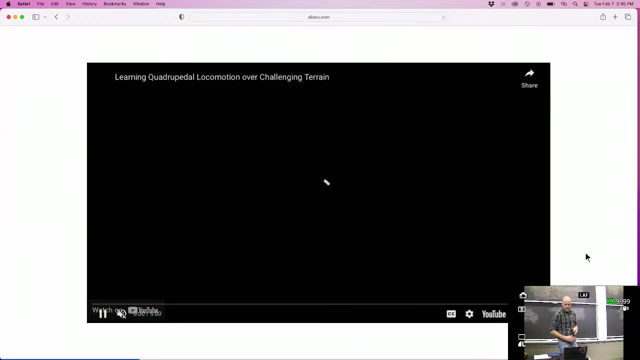 Okay, so we're roughly going to spend the semester, making sure we understand how that kind of stuff works and how new advances in machine learning should change the way that we build control systems like that. And we're going to try to dig in deep to that kind of technology. So that's one of my favorite examples, the Atlas, right? 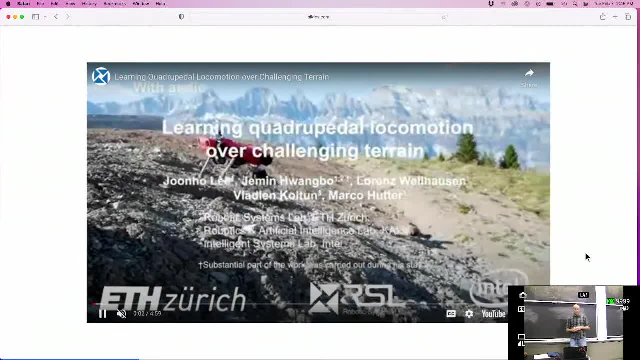 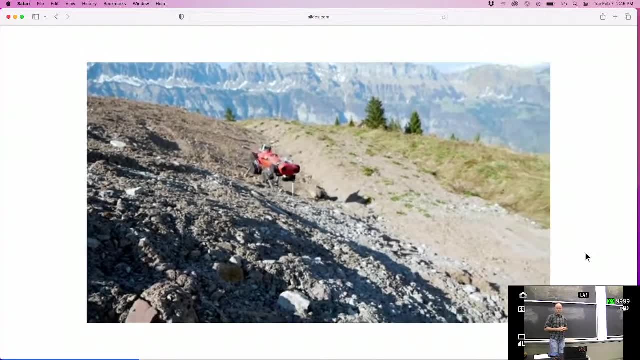 Here's another fantastic example. This is a quadruped walking, but you can see from the title slide there that this is a reinforcement learning-based approach to doing quadrupeds. And that's big. That's new. That's... 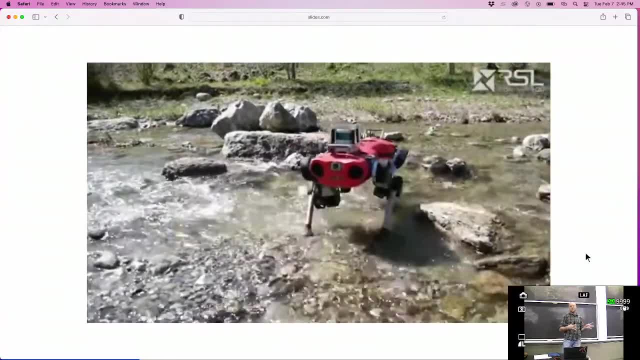 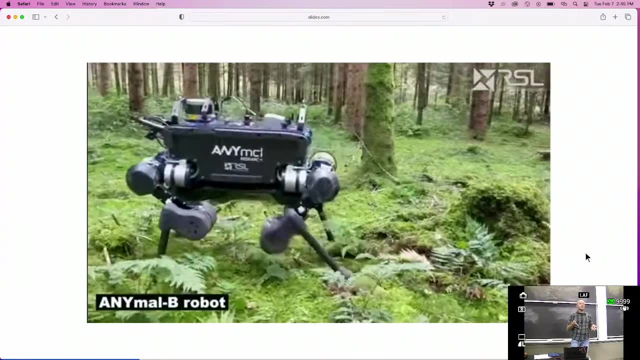 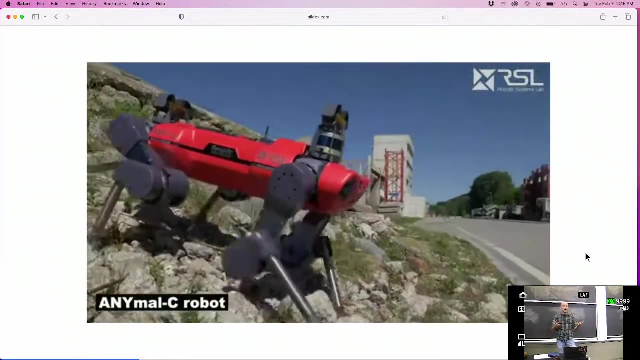 You wouldn't have said even a year and a half ago or something that reinforcement learning could compete with some of the other control approaches, but it's starting to happen, right? And we're seeing some of the controllers that people would really field being powered by machine learning 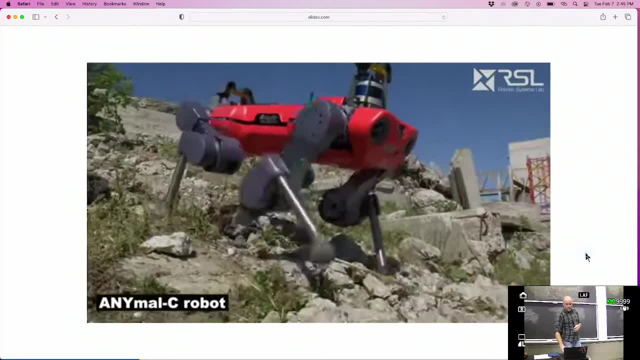 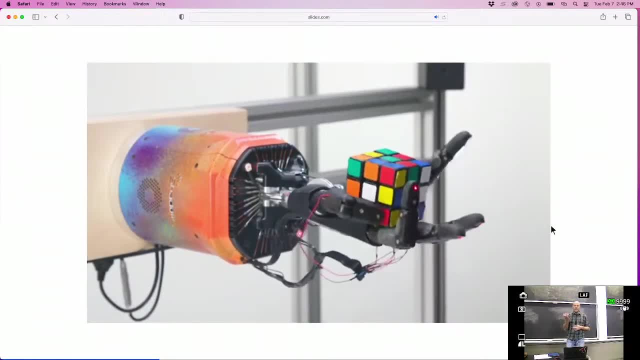 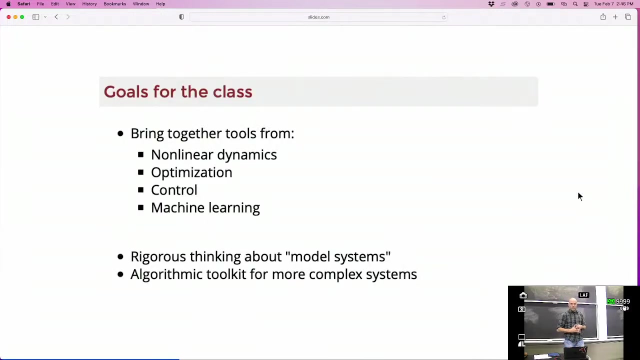 Really interesting dynamics task with lots of rich contact interactions. So you'll appreciate by the end of the class how rich the problem of contact mechanics becomes in a setting like this. And we're seeing more and more advances of more and more capable robots in this direction. Okay, so the background, the the tools that we're going to bring together to try to understand those kind of systems and not just kind of just be able to approach the problem. I'd like us to try to deeply understand the problem, right? We're going to try to bring together tools from nonlinear dynamics which is similar to mechanics but a little different. I want to focus not on where we get the equations of motion but how to think about the time evolution of equations of motion once we get them. We're going to use a lot of tools from optimization, linear programming, quadratic programming, semi-definite programming, things like this. We'll talk 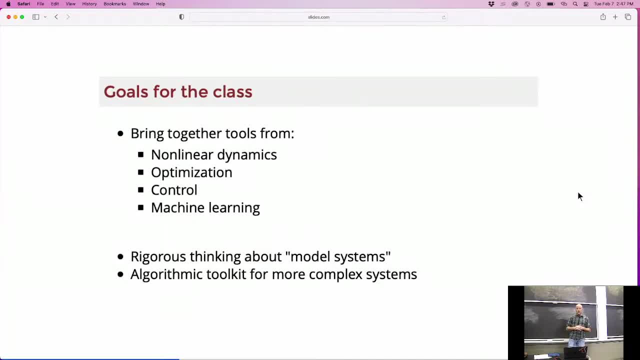 about control theory and we'll talk about machine learning and how all these play together. And the way that we're going to go through that material is by trying to come up with simple examples of the system. I'm always a huge advocate of trying to find the simplest possible robot, for instance, the simplest possible model that captures the essence of the dynamics problem we're trying to solve. And we try to understand that, you know, as well as we possibly can. And then we'll slowly build up to more and more complicated systems. Okay. And what you'll come out with, I hope, is an algorithmic toolkit. You will know how to use some of the RL algorithms but also some of the model-based algorithms and we'll have a suite of tools. 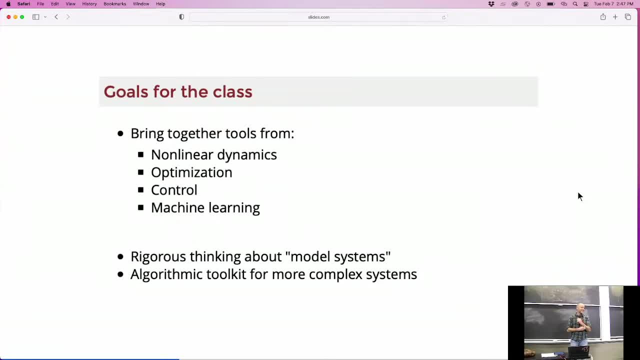 Okay. That you'll be able to apply to your robots. If you happen to have a super strong humanoid robot at home, or maybe even the $2,000 quadruped at home, then hopefully we'll give you a bunch of good tools for that. 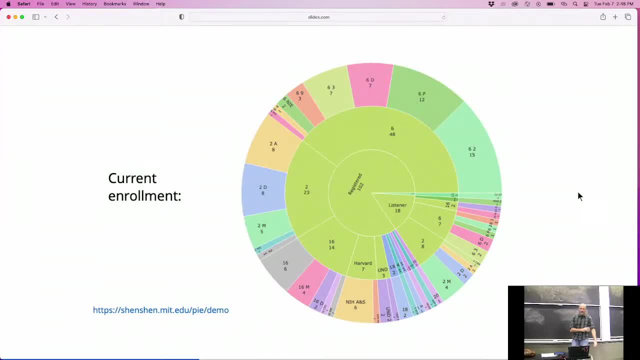 It's actually interesting. So one of the roles that this class was originally set out to play was to bring together people from a lot of different fields. And it still plays that. So I actually... Shen, who's in the back there. Shen, who's in the back there. 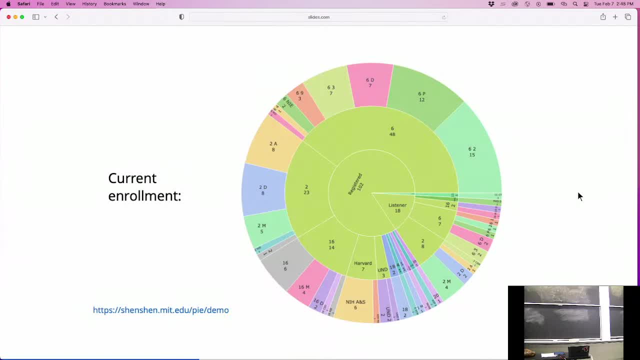 She's our instructor in course six. She made this little tool where we can take the class 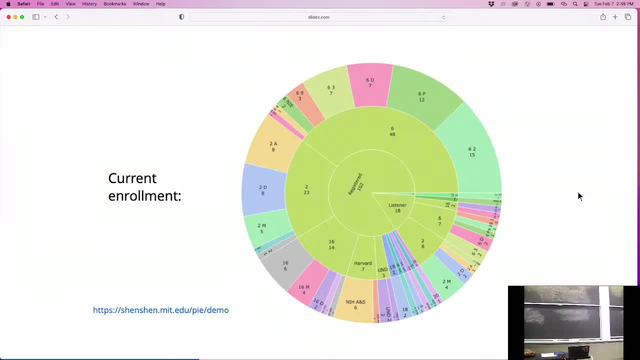 and make a pie chart of where people come from in terms of departments and things like 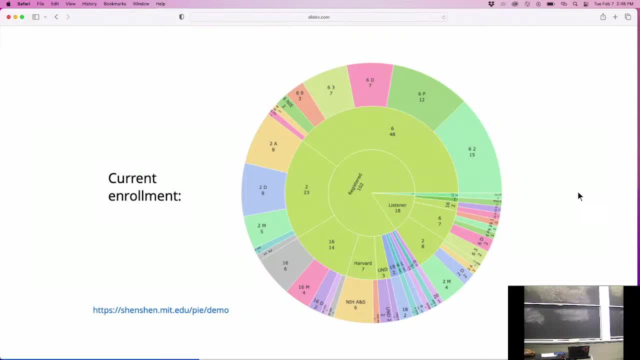 this. And this is course six here. There's 48 of you from course six. There's 23 of you from course two, from course 16, from Harvard. There's some listeners. But the point is there's 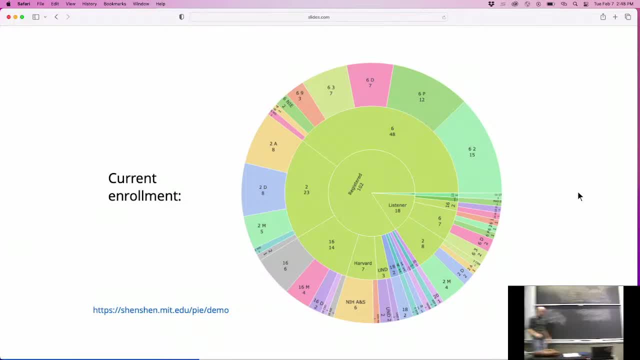 a lot of colors here. Okay. And although we're covering all those different topics to some extent, my goal is to... I don't expect anybody to come in understanding this course. They're those four areas right and I'm trying to for computer scientists maybe they think 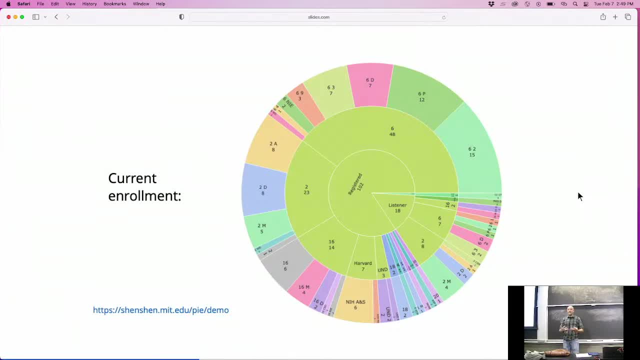 a lot about machine learning I want to this to be the class where you think about dynamics and how the dynamics should impact your thinking about learning maybe you've thought a lot about dynamics but you haven't thought as much about planning and control or learning you know so that this would be the class that will bring those two worlds together okay so that's always my goal in this class but also my challenge in this class to try to bring those 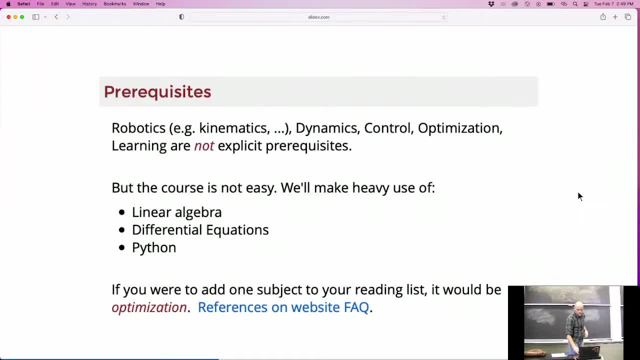 different communities together I often get asked about prereqs right so I do not assume you know you've taken as a basic robotics course actually so if you 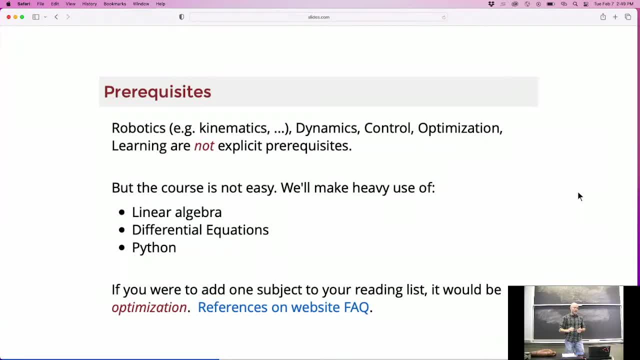 if you've never designed you know sort of done by hand robot kinematics or dynamics that's okay we're normally just going to use the software to generate those for us you don't need that as a prerequisite even dynamics and control and optimization I'm because we're coming from so many different areas I'm going to try to introduce the core ideas of course if you have more expertise in those then I will hopefully complement your expertise and give you different aspects of that but I'm going to try to introduce the basic concepts and give references if you want to go a little deeper on any one of those ideas that does not mean that the course is easy I think the place where we're sometimes people get surprised by the by the requirements is is just the way that we're going to throw around linear algebra algebra and differential equations so we're going to write matrix differential equations I'll show you some this lecture partly just so you get to see 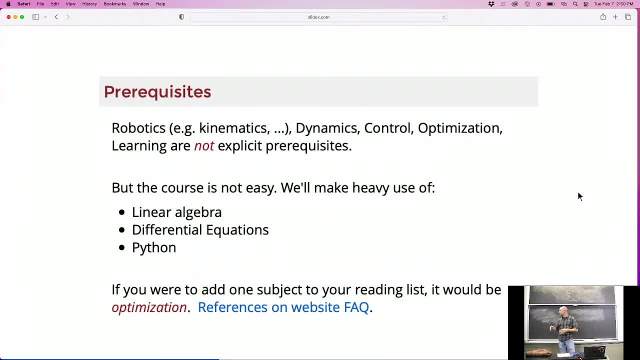 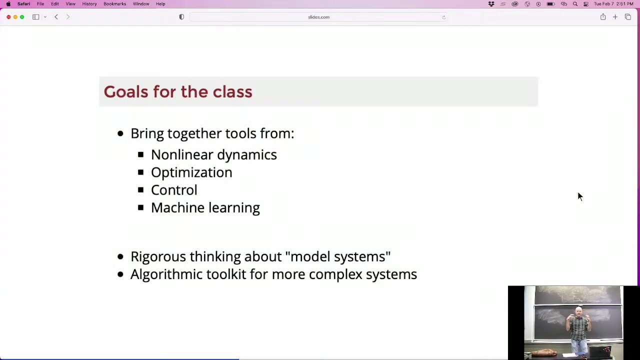 what you're up against there I think 1803 1806 those kind of classes will prepare you for this and if you can run along okay but I consider those the more important prerequisites than having expertise in in any of the back of the big topics we do use Python pretty heavily so comfort in Python helps a lot I would say the one thing that you know I think a lot of the dynamics a lot of the control we can introduce the core concepts I will introduce the core concepts from optimization but if I were to say well there's one area that if you'd feel not super comfortable and you want to do extra reading as we go along I would say optimization and there's a there's two really great references on the website for that the void convex optimization book or the no-suit all and write optimization books are just really great references if you want to think about that but I'm going to go ahead and fill out I always feel you know I wish I could spend a few more lectures on that background material okay so again the we're talking about sort of the 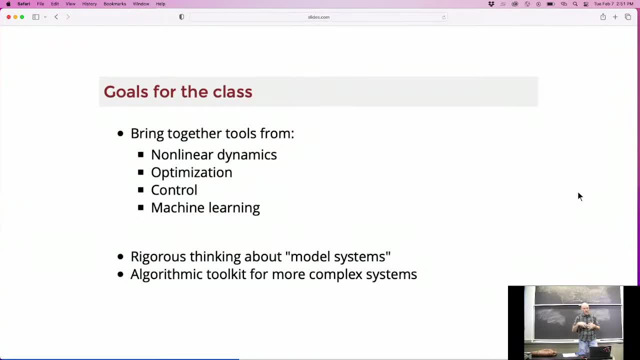 confluence of a handful of different topics optimization machine learning 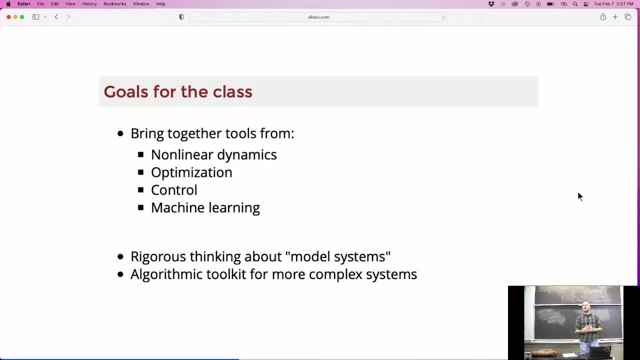 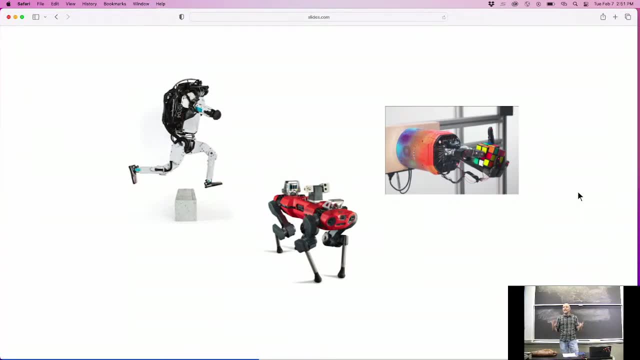 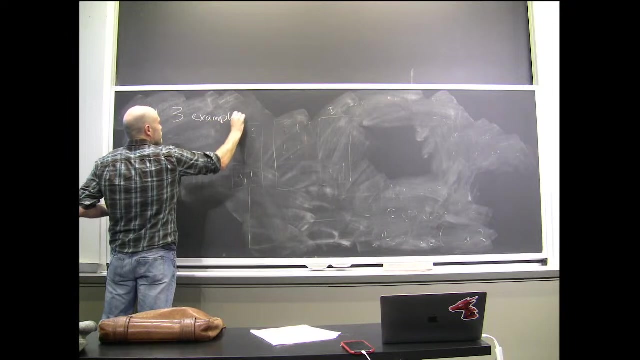 they're deeply connected deeply related okay and I think an interesting way to think about that is is when you put these three systems that I chose up on the right hand side of the screen and you can see that there's a bunch of board together okay so one of the questions that I know the Boston Dynamics folks that the Atlas robot the humanoid always get asked is does it use machine learning right and the simplest answer is no that doesn't really use machine learning if you were to ask animal or the open AI folks does it use machine learning the simplest answer is yes those use machine learning okay and you know what's and then people will say well that's too bad Atlas maybe next year you'll use machine learning and you'll be but I I want to dig a little deeper about that in this class I mean even just to say a few words about it today right so you know the simplest answer of Atlas is no but I would say all three of those examples there's a they're more similar than they are different right all three examples start the work started by building a detailed 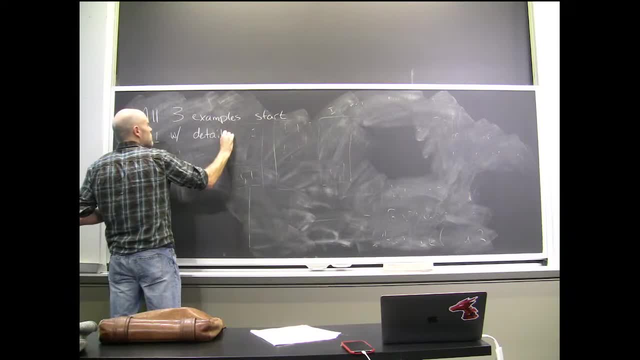 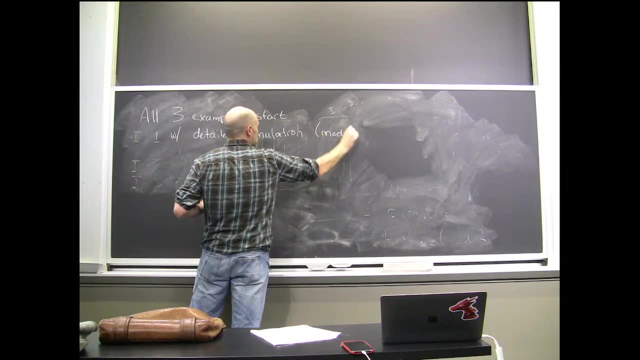 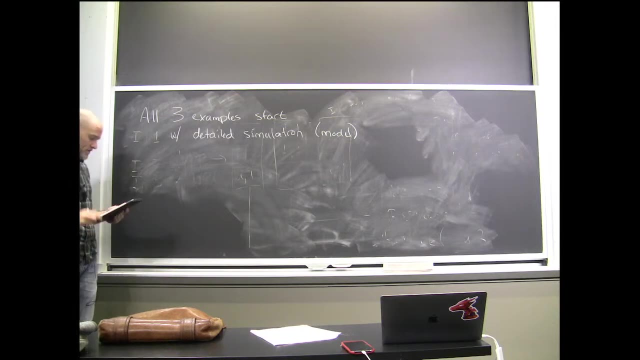 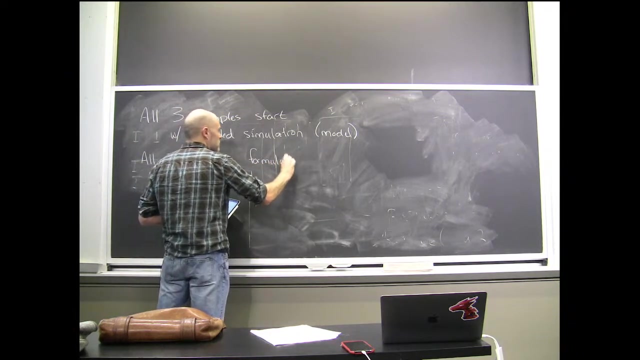 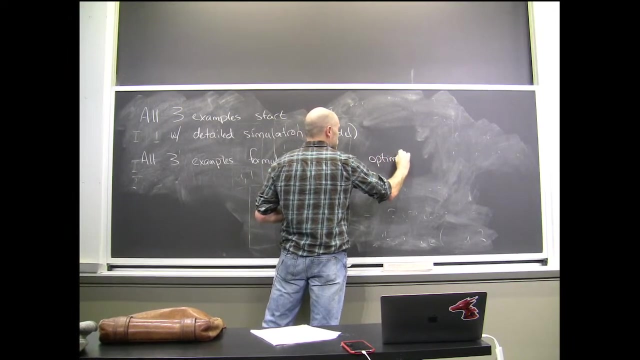 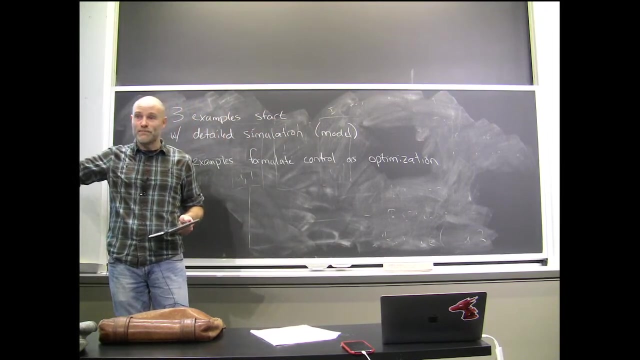 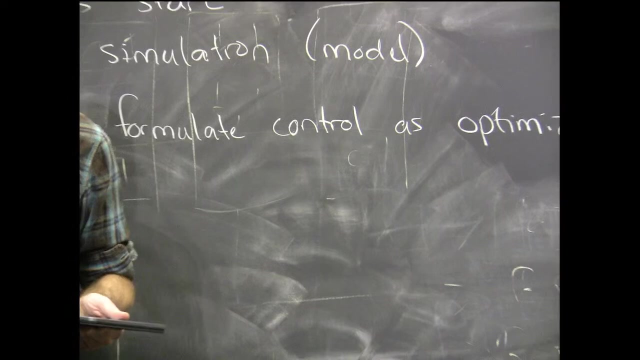 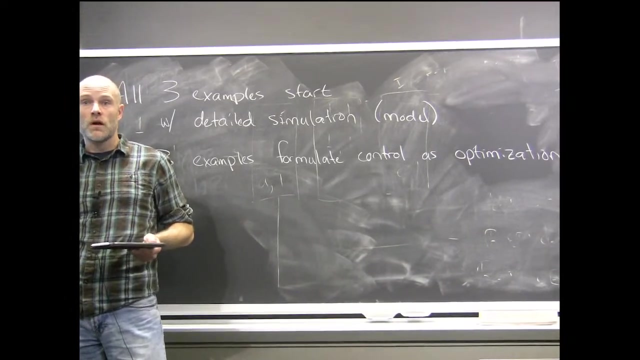 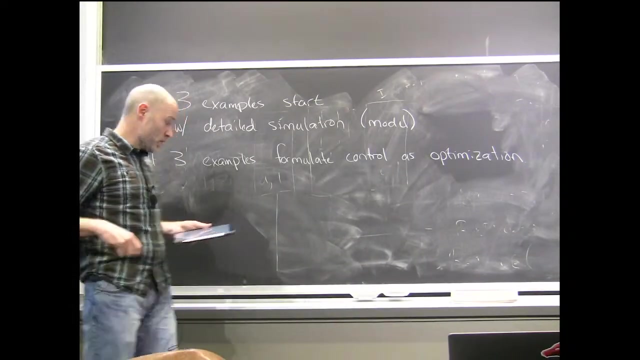 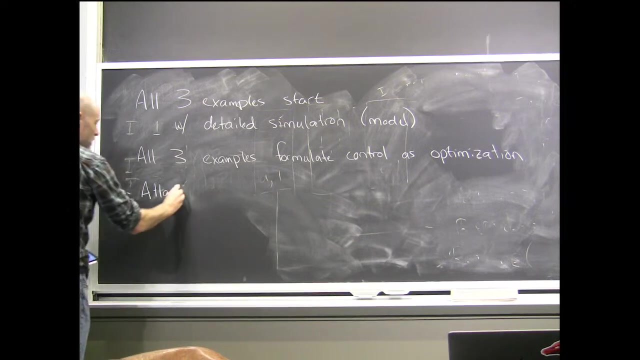 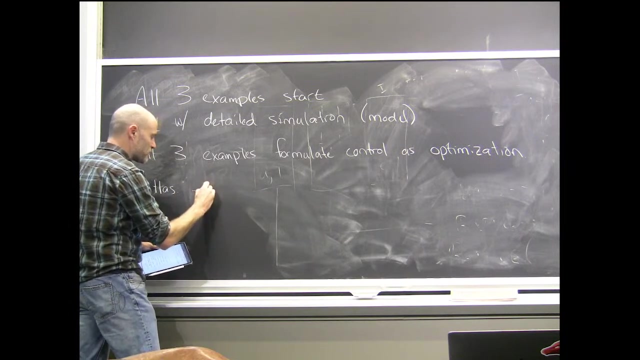 simulation let's call it a model a dynamics model okay so we you know all three of those the the simulator was a big part of the of the work right and so all three I've got some lines that were hard to get some stains I guess from the previous lecture right all three examples formulate control with as an optimization right we'll talk about the specific formulations and the but roughly, you know, you get points if Atlas doesn't fall on its face, you get points if it does a backflip, right? And the way that we talk about what the controller should do is as an as a cost function, as an objective function. Same thing for any model, same thing for the hand, right? We're writing optimization based controllers for all three of them. The difference, right, for Atlas, which is the Boston Dynamics one, right? The search, the optimization, we're going to get into all the details of these as we go through, but just to foreshadow, right? The optimization is over the parameters of a trajectory, okay? 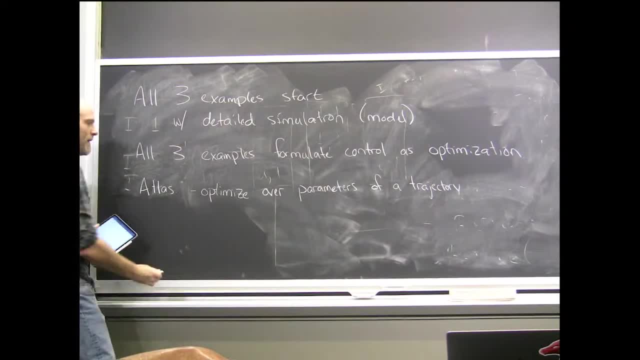 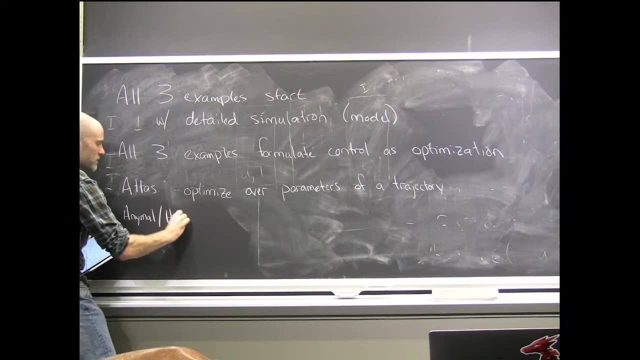 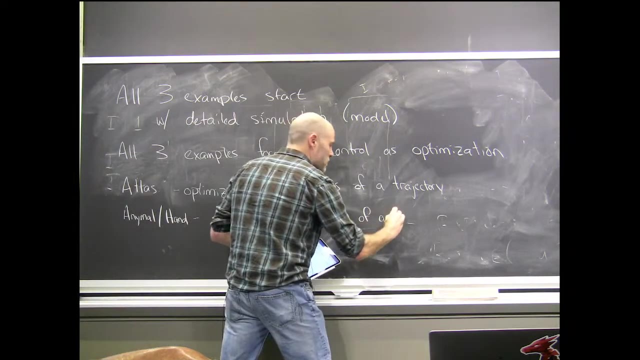 Okay, and for the other two, I'll say, any model on the hand here, they're optimizing over parameters of a neural network. 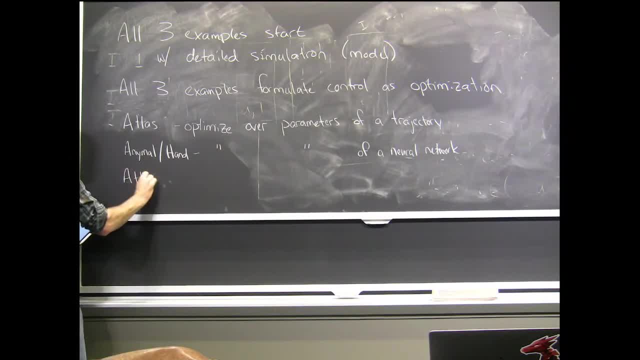 Okay, for Atlas, the optimization is over the parameters of a neural network. Optimization uses gradients, so it asks for a differentiable simulator, right? If you will. 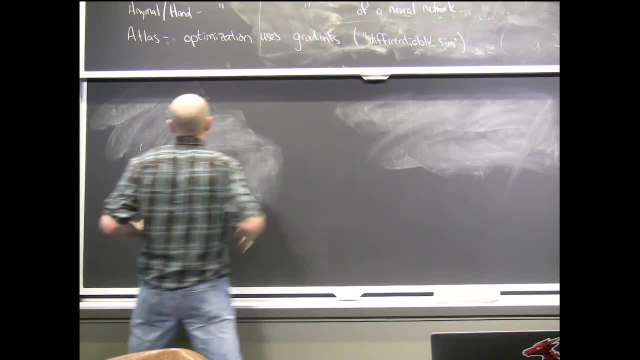 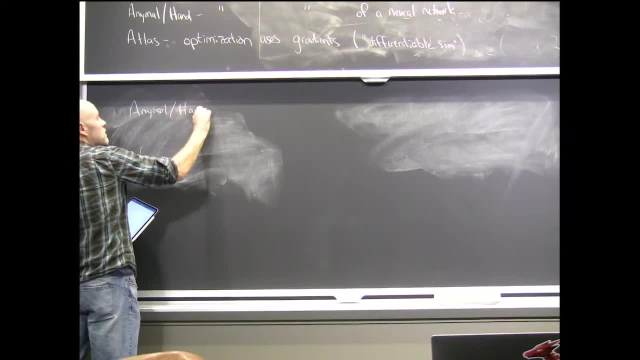 It's not quite that, but it's almost that. Okay, any model in the hand, just use a black box optimization, we'll call it. 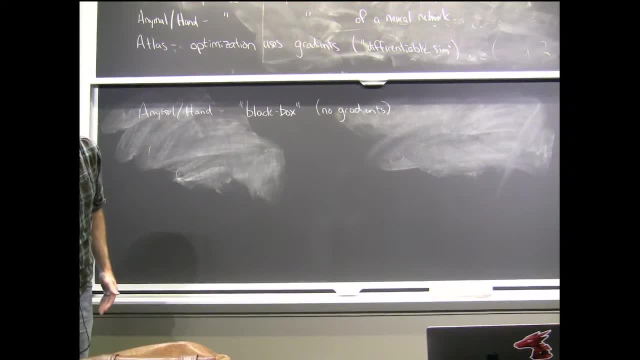 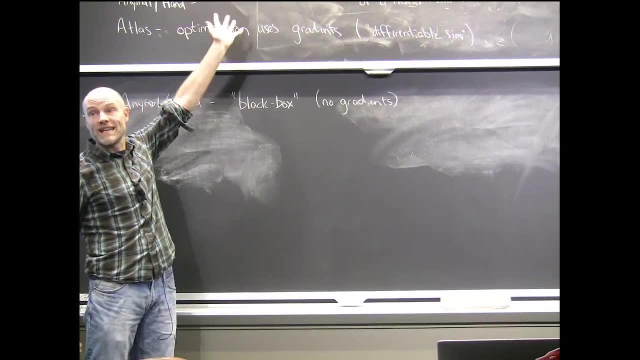 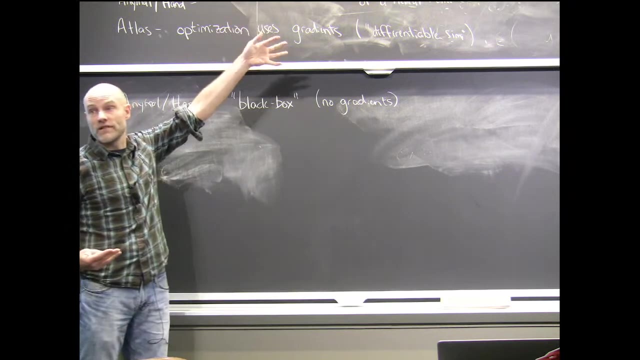 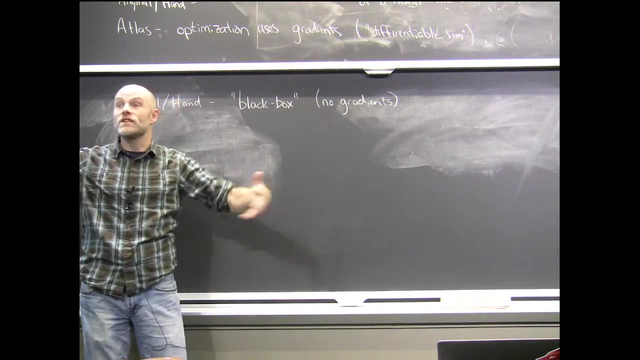 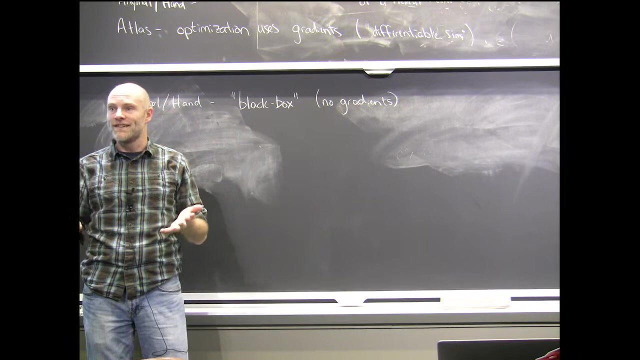 Okay, but really, they're not, they're more similar than they are different, right? There's a few other differences. Atlas is able to do the optimization so fast that it runs online, right? They're constantly, as they're running, re-optimizing that trajectory, which is why they can get away with only parameterizing a trajectory. And the AnyMall case is training a neural network once offline and then using that neural network on the fly. But the differences here are more about the optimization landscape because of the way we've chosen the parameterization that we're going to optimize over. 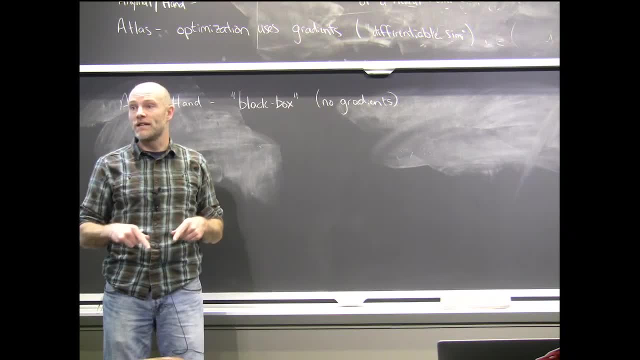 And the optimization algorithm, one of them is doing straight-up gradient descent or sequential quadratic programming. We'll talk about all these things. 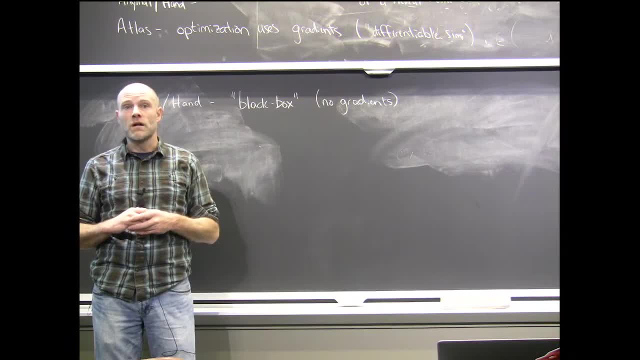 And one of them is doing a more randomized search. But they're more similar than they are different. 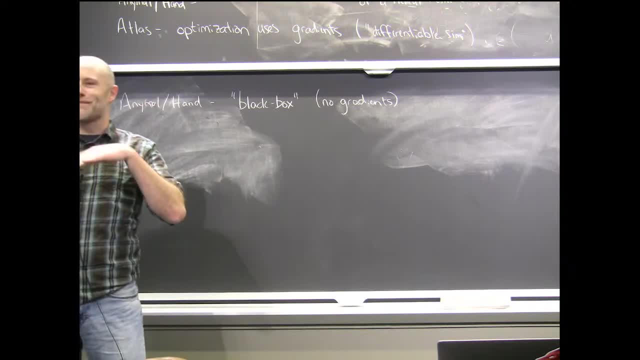 Okay? So I don't think either of those approaches has some glass ceiling. You don't have to feel bad for Atlas because it's not learning, right? 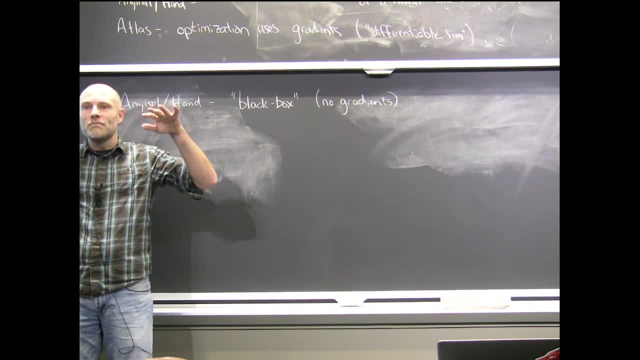 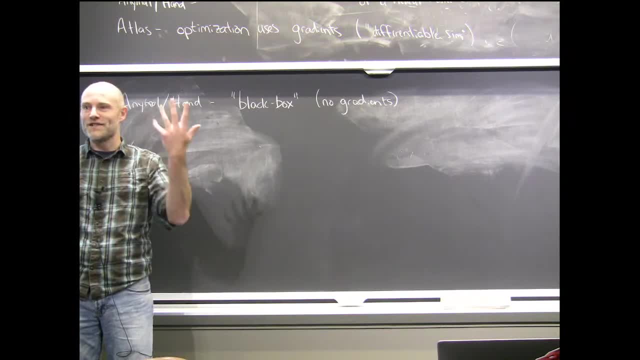 That will, as we understand things better and see that they're just multiple sides of the same, you know, big problem, then we'll understand how to put the best of all this together. 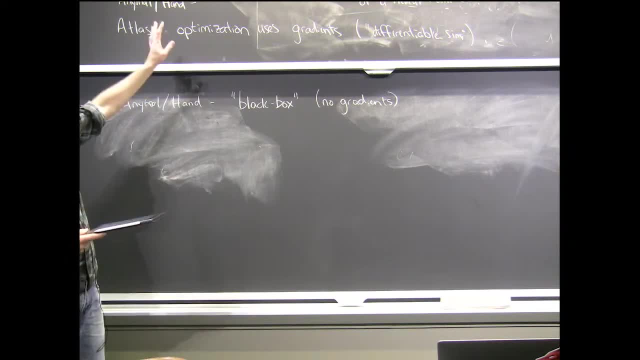 So we'll try to understand all those ideas, you know, specific algorithms, but also the concepts of what does it mean to think about the way the optimization landscape changed and what are good optimization landscapes and the like. That's the kind of thing we want to talk about in the course to try to understand more deeply. 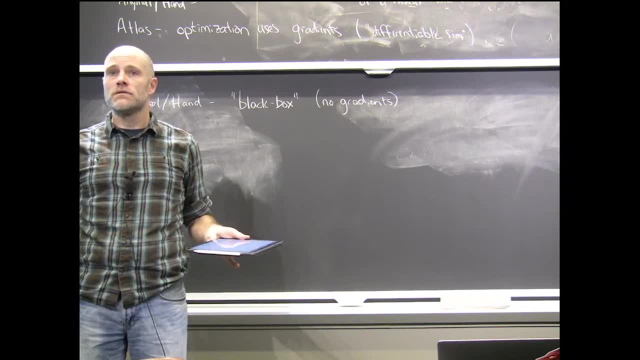 Any questions at a high level? I love questions, by the way. Ask questions. You have them. Anybody sad that Atlas doesn't use learning? Okay. I'll try to encourage questions as we go. Of course. Great. Okay. Yeah. How do you, like, how do you, like, 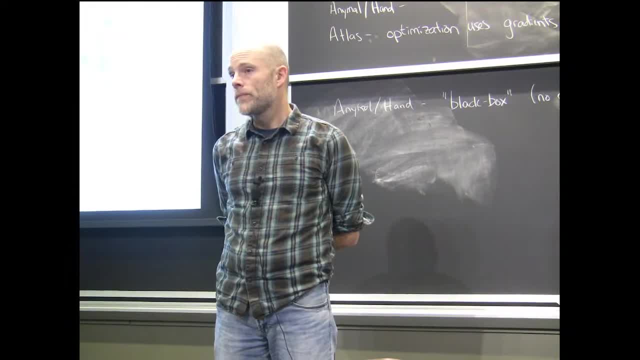 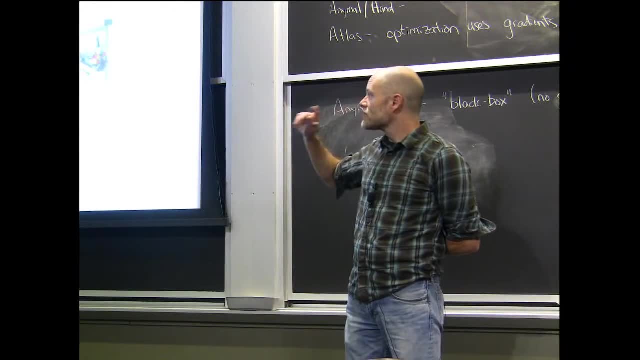 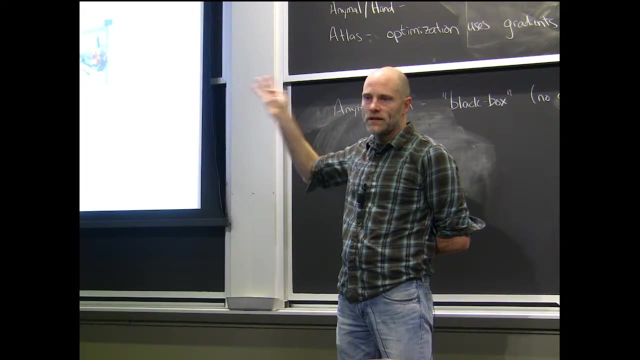 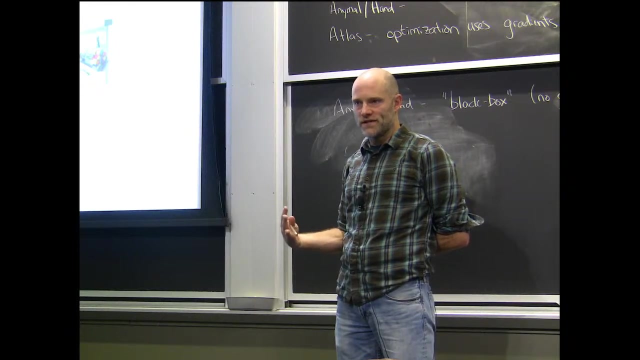 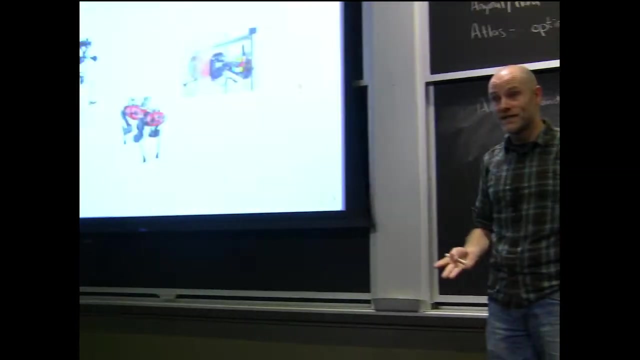 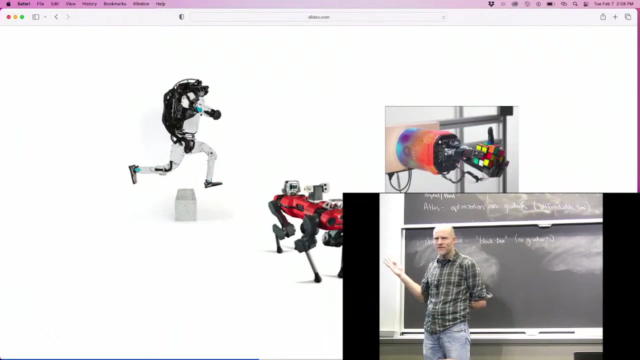 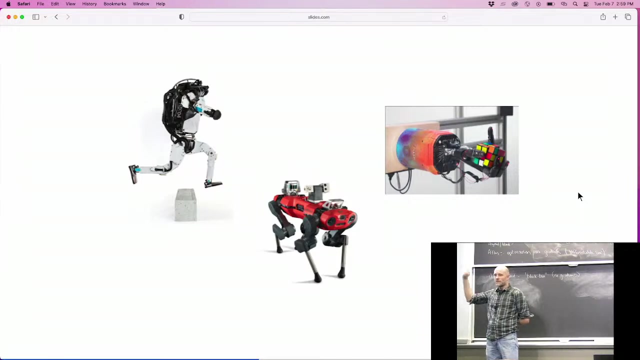 versus animal how do they differ in terms of the onboard processing hardware that they need yeah that's a great question so the question is about onboard processing hardware so i think um i think both of them could carry sufficient compute for this uh i think i don't know that atlas is doing it online i actually don't know the details the version of atlas that we had had sufficient compute in its belly to do all of the processing we needed and we had to run off you know off the grid and stuff like this the newer version of atlas has been trimmed down it's got much more emphasis on minimizing weight and stuff like that i i've seen it run outside i'm sure they have enough compute to do all the algorithms on board and similarly even the the inexpensive quadrupeds are carrying uh gpu uh hardware acceleration you know in their in their bellies now so i think that affects their battery life but the carrying capacity seems to not be you know the problem of 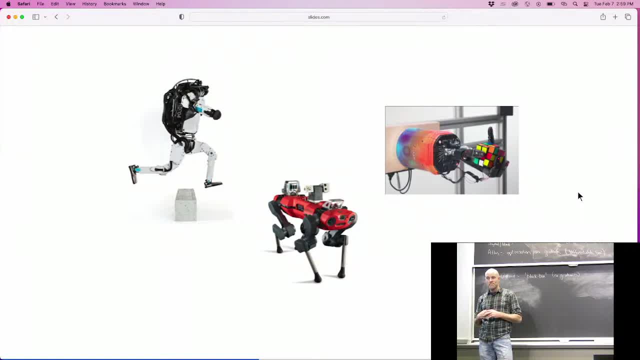 carrying the computers seems to not be what it used to be great yeah actually that's a part of what's happened with hardware is just that you know batteries got better compute got lighter right we used to be that if you had to carry enough compute your dynamics got worse because of the weight of the the computer yes that's a good question yeah so if the if the world is 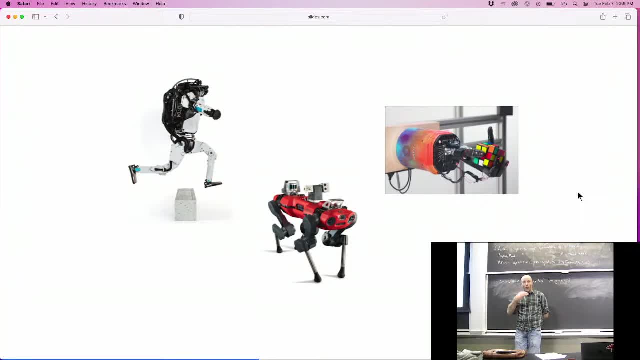 changing or the dynamics are changing i'm going to give it a little bit of 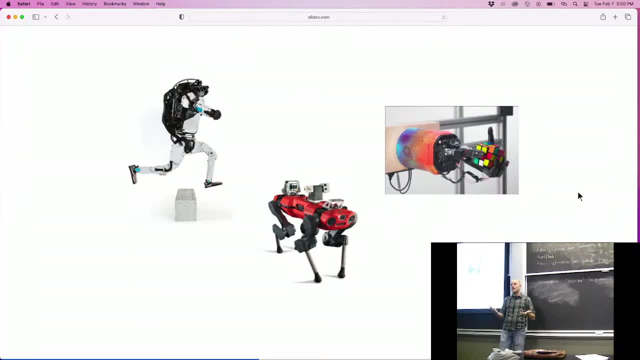 well there um It's more of a robust strategy where it needs to be exposed in simulation to the types of things that we'll see in reality. 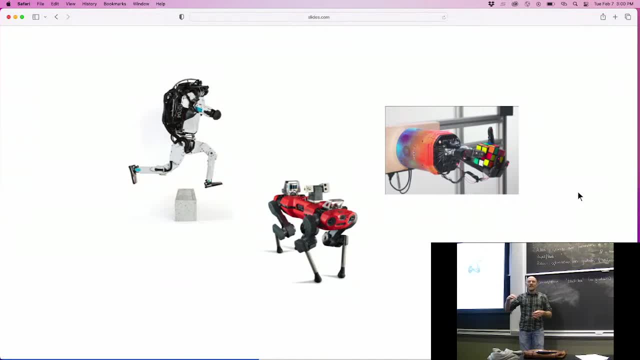 And one of the amazing success stories of that is that exposing it to relatively simple sandbox of different environments in simulation was enough to do what looks like much more complicated things in the real world. So if you're robust to stairs and just a handful of things, then you're robust to walking up a mountain, which is awesome. But that's a story that control has given us often throughout the years. Thank you for the questions. 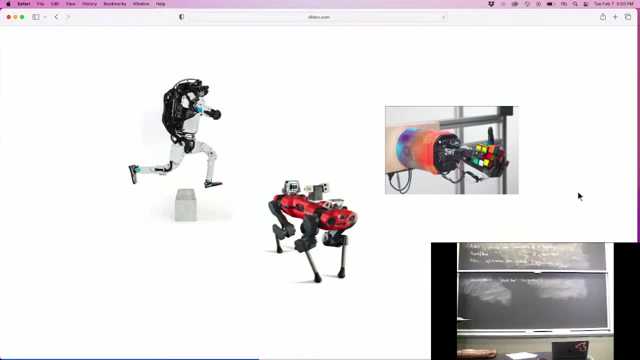 Okay, so let's give a couple definitions. I want to get a little bit more specific. That was, I think, good at the high level. 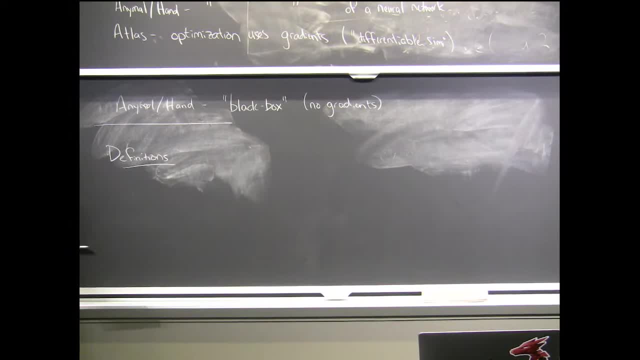 So the beginning of every reinforcement learning talk or book, or something like this, starts with a diagram that goes something like this. 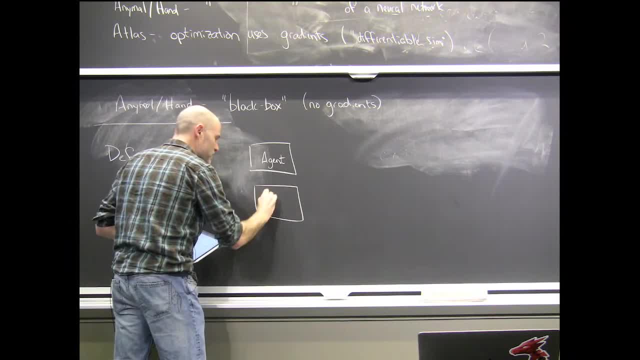 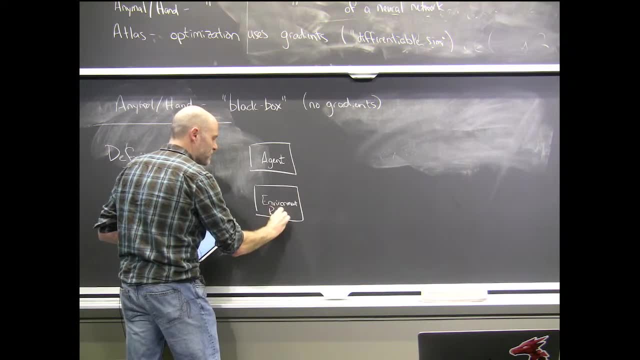 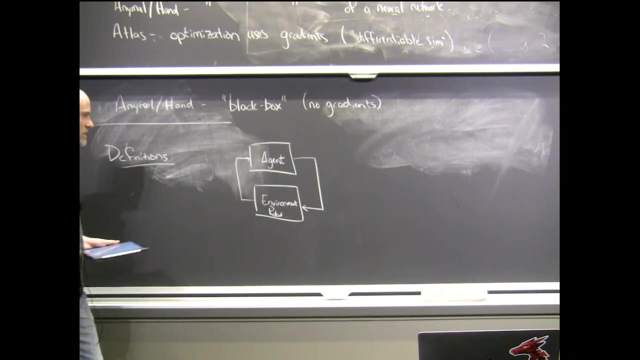 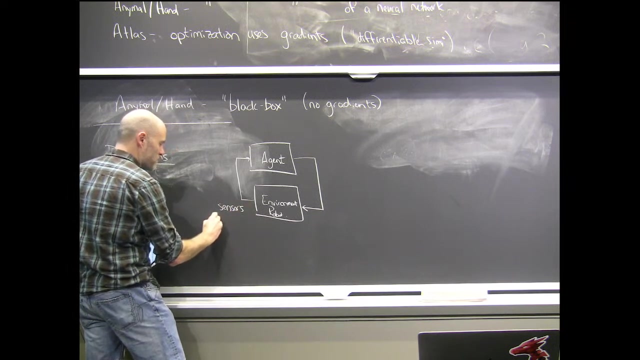 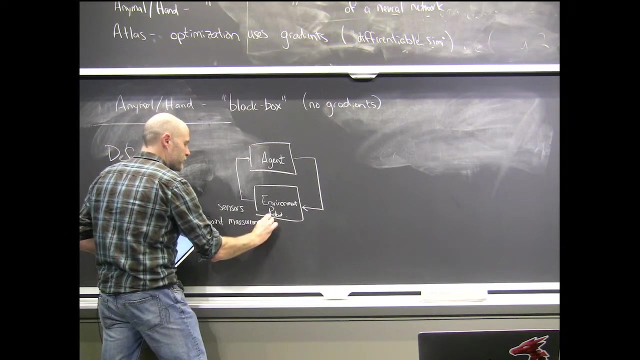 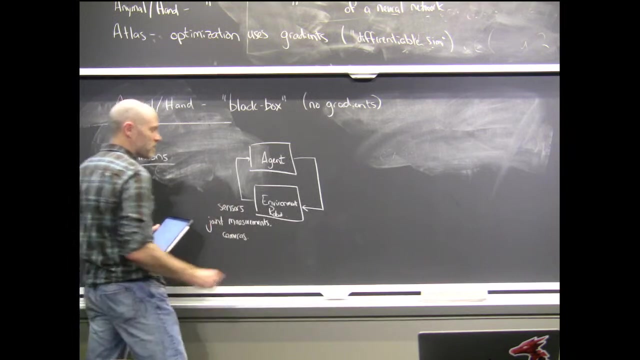 I have an agent, and I have an environment, where this might be a physical robot, for instance, and this is the brain of the robot, for instance. Okay, and I have a feedback loop that connects the two. So the environment, his output is the sensors, which might be, the joint measurements, cameras, you name it, okay, on some list of sensors, and the inputs are going to be the motor commands. 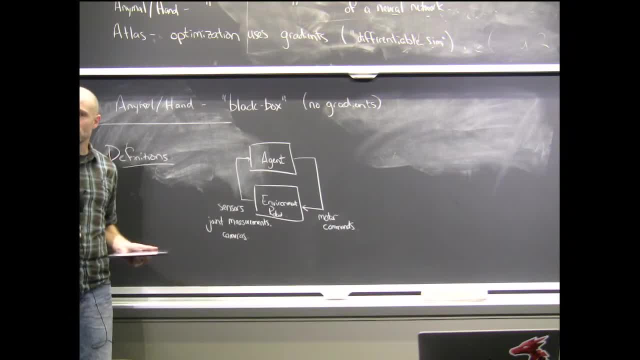 So I'll often use the term actuator instead of motor. Motor is a specific type of actuator. Typically, I like to call it an actuator. An electric motor, for instance, right, and an actuator could include hydraulics, or pneumatics, or other things. 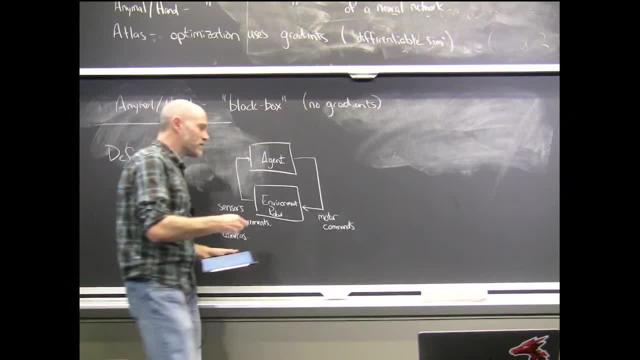 So actuator is the broader term, but if you haven't heard the term actuator, I will often use that, and you can almost substitute it for motor if that's your preference. 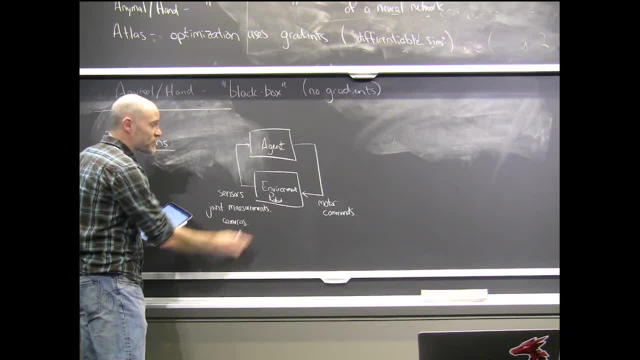 Okay, so this is the same, this is the control problem. There's nothing wrong with that. 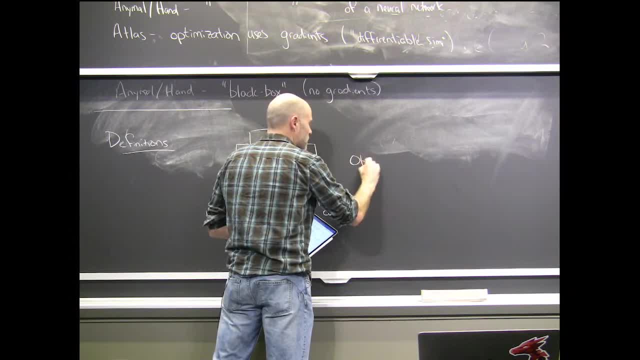 The other thing we have here is that we have some objective, or some cost function, or reward function. 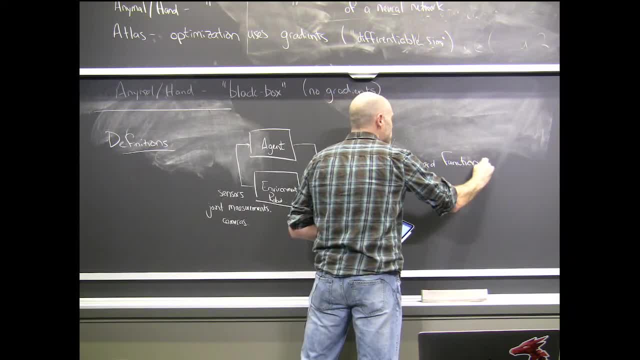 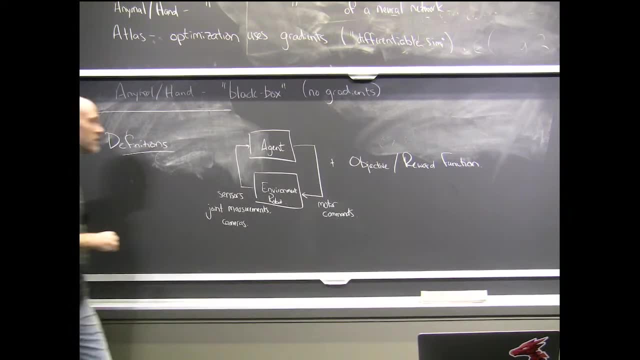 This is how we define an optimal control problem, or a reinforcement learning problem. In control, we tend to call, or even, you know, another word for this part of it is to call this the policy, 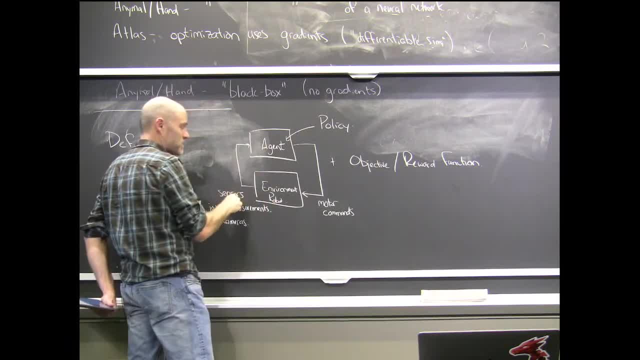 which takes sensors, histories of observations, possibly, and produces motor commands. 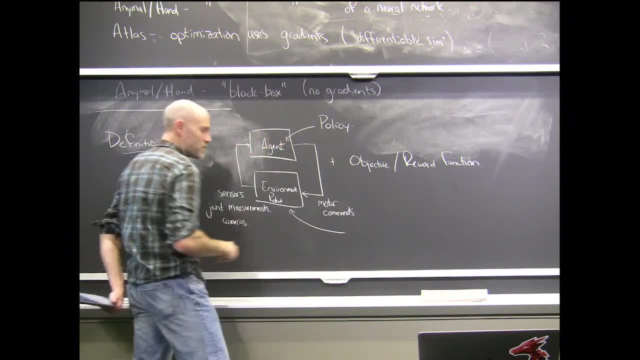 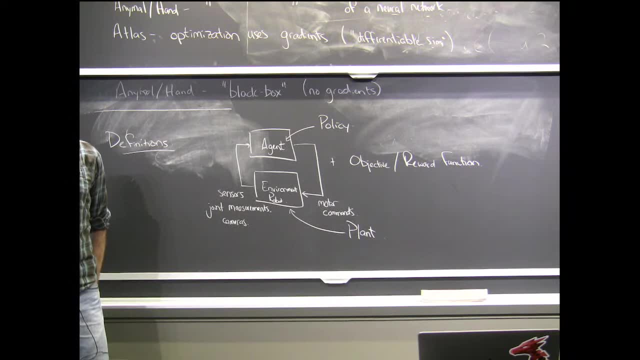 Okay, and then the control theorists will call this part the plant. Right, which sounds totally out of date, but it's baked in hard. Like, I will never be able to call it anything else. 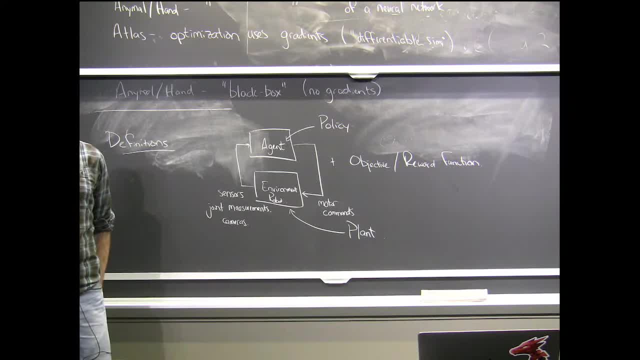 It started from, you know, because a lot of the interesting control worked in chemical plants first, okay? But the thing you're trying to control is the plant, and I think it's okay. 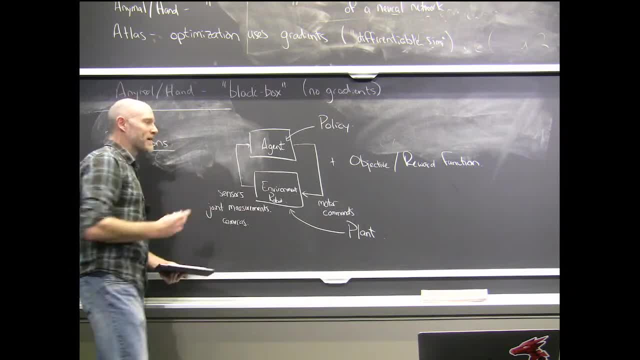 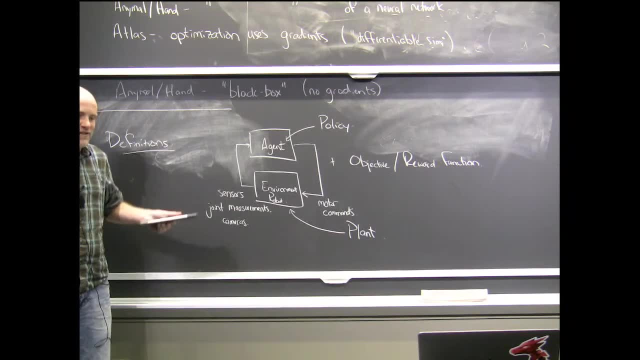 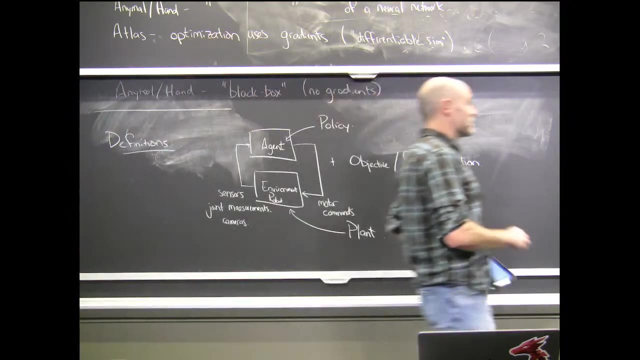 So, all right, so given this very broad perspective, I think it's interesting. I think you guys should give me feedback, but I think the general, the general understanding of machine learning has just, you know, it's just so much more pervasive that I think I can say some of these things, you know, even before giving all the specific definitions. 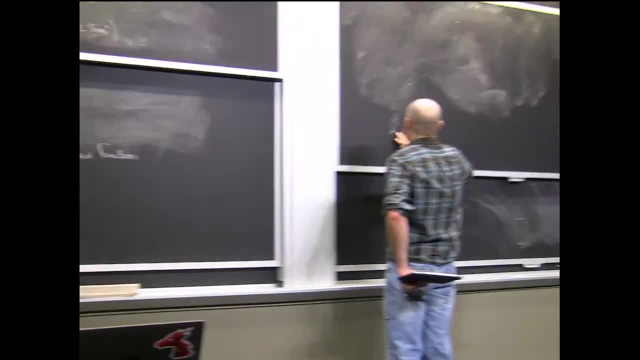 Because I think people have heard, you know, basic things about what makes reinforcement learning hard, or machine learning hard, and I'll try to build on that. 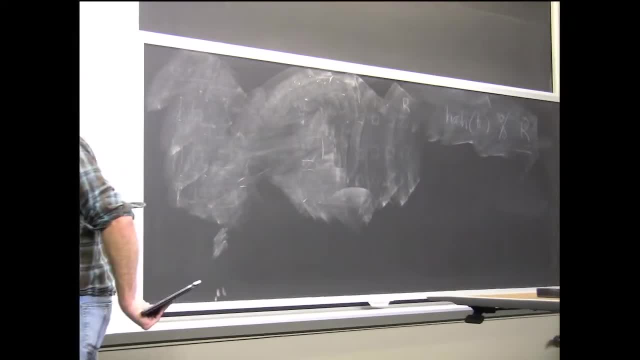 But we'll, of course, circle back and make it all very concrete and specific as we get into the details of the course. Okay, so what makes control hard? Okay. Okay. 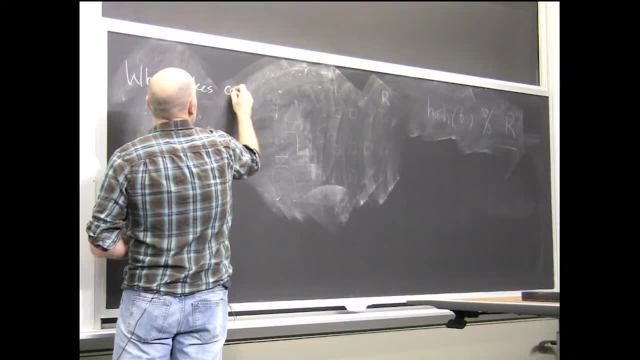 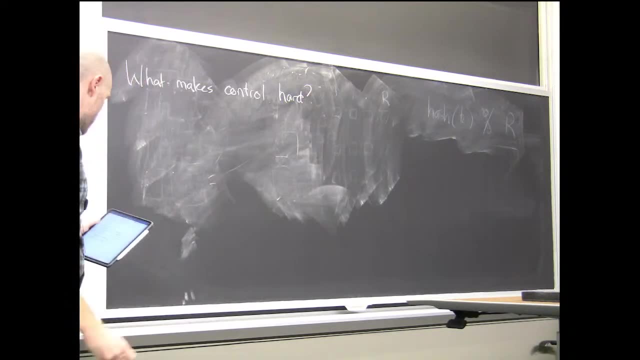 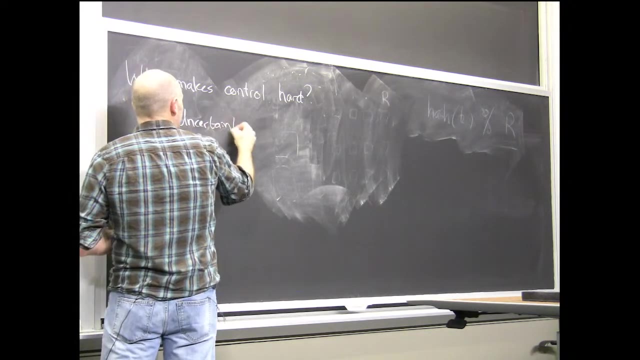 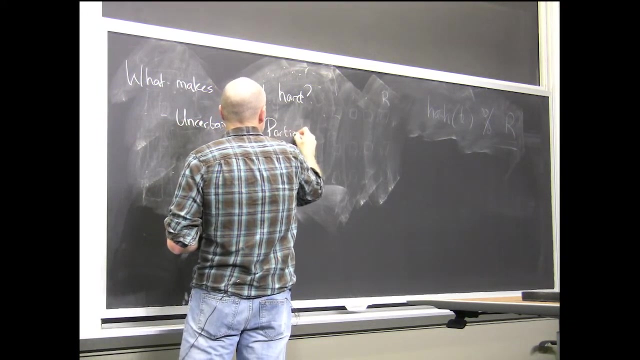 There's potentially a long list. I'll just highlight a few of them here, right? So one of the big ones is if you have uncertainty, you don't know what the world's going to look like, the world's changing dynamically possibly, or if you have something called partial observability. 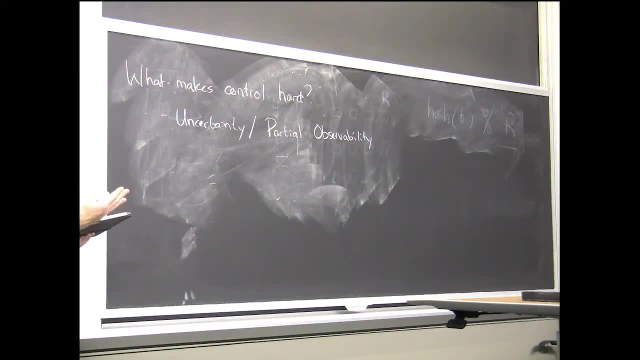 Where looking out your sensors right now can't tell you everything that's happening in the world. You have to somehow accumulate understanding of the world through long histories of observations and infer something about maybe what you can't possibly know. 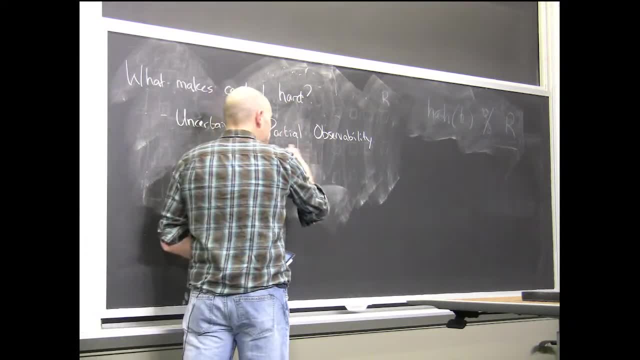 These are big issues, but they're not the primary ones that we're going to focus on for the big part of the class. 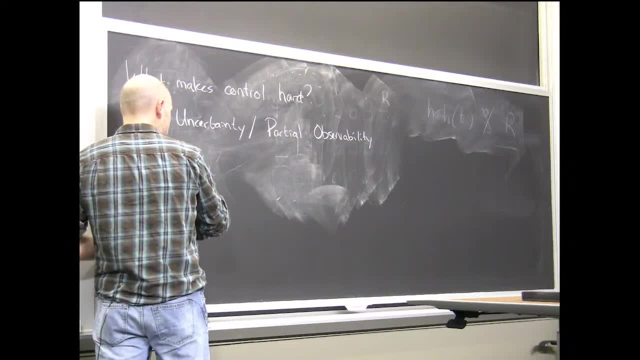 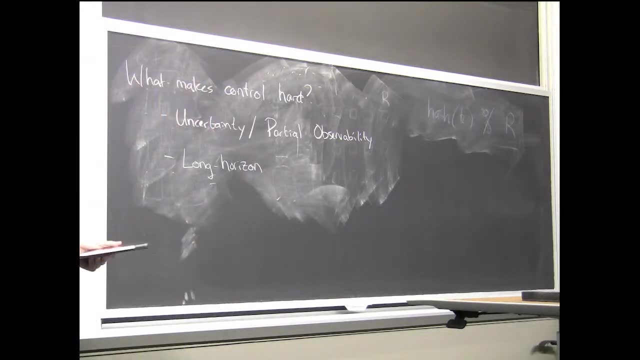 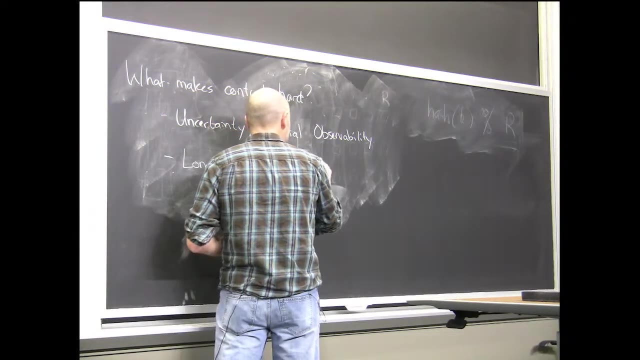 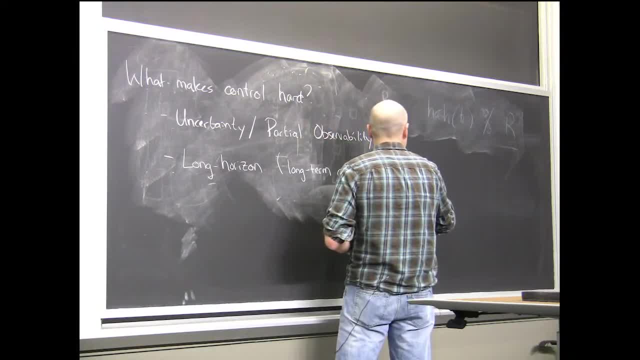 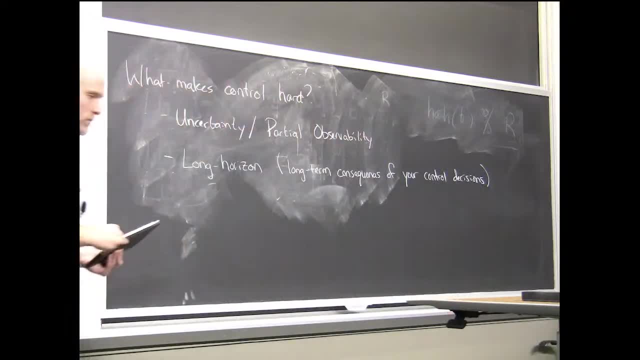 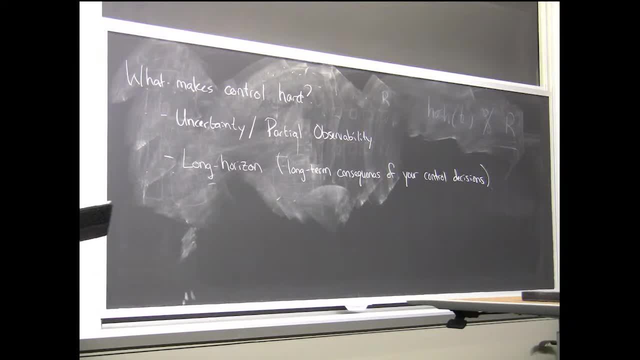 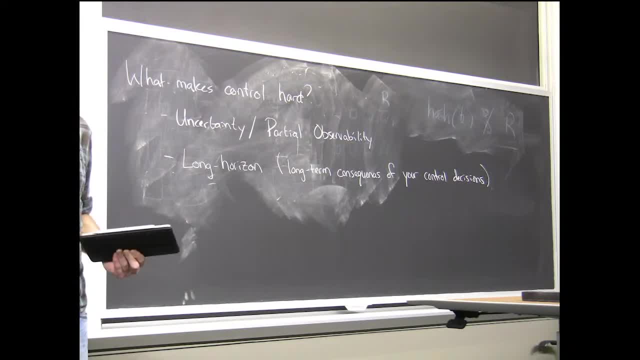 Okay. 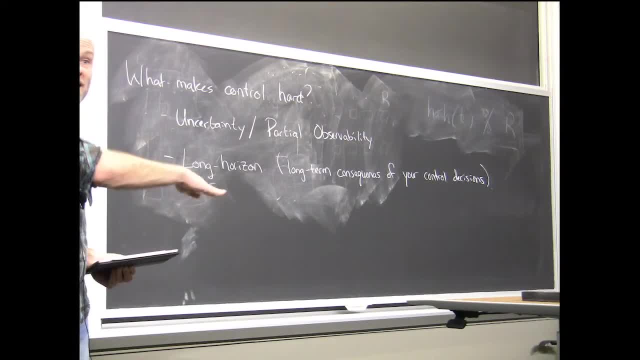 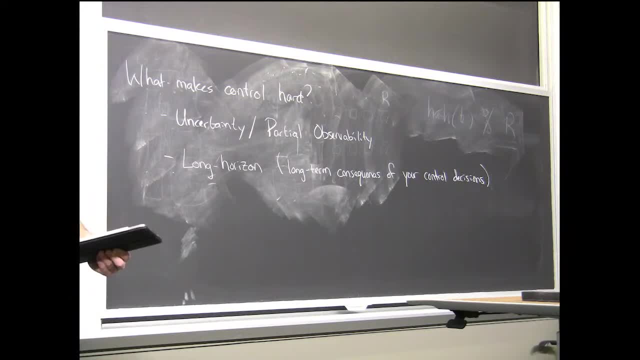 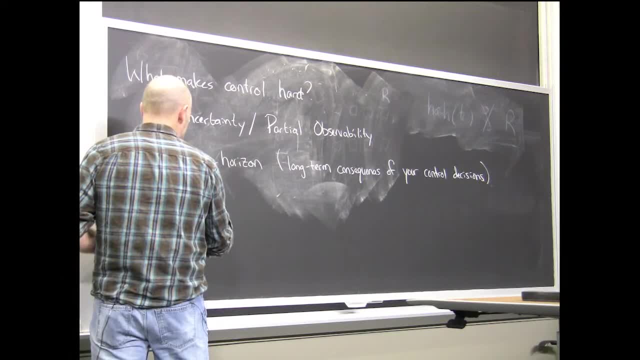 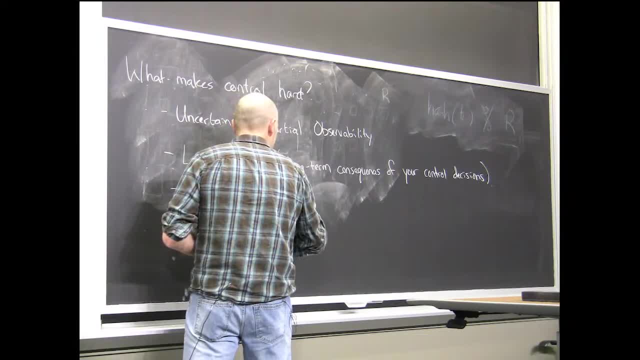 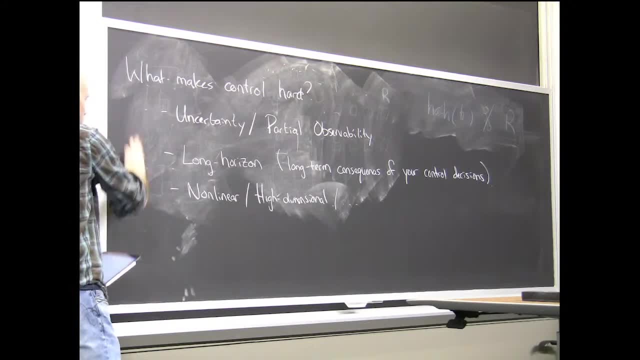 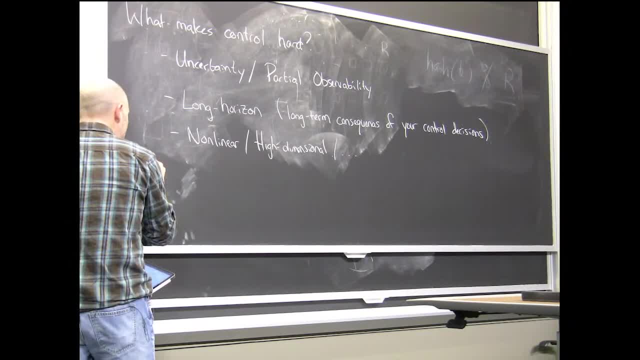 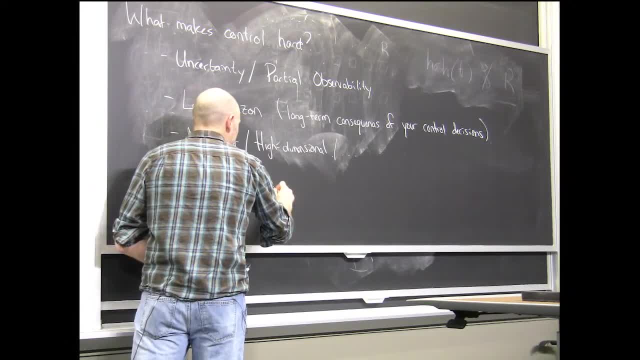 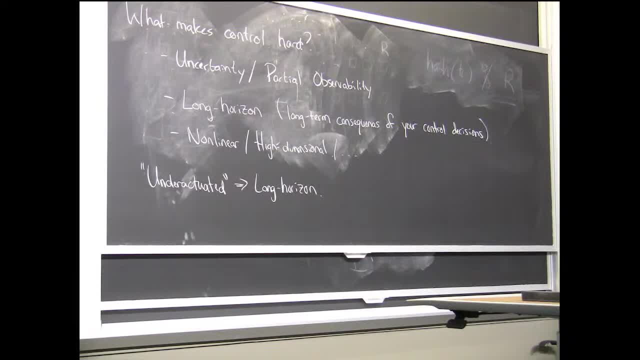 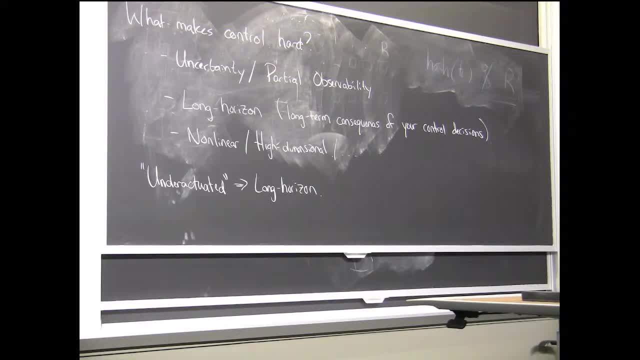 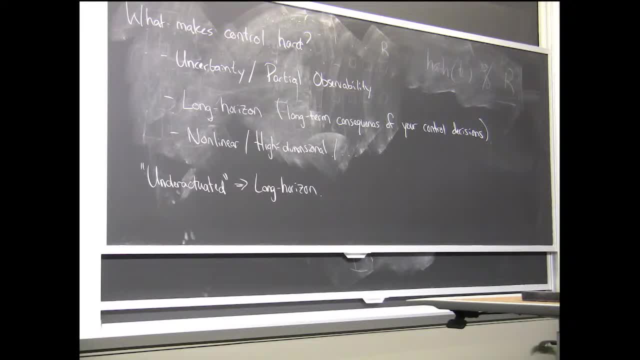 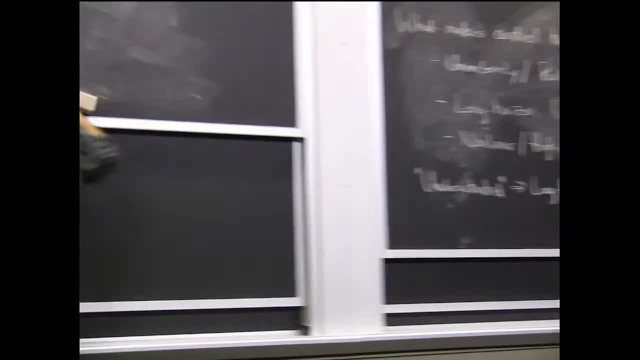 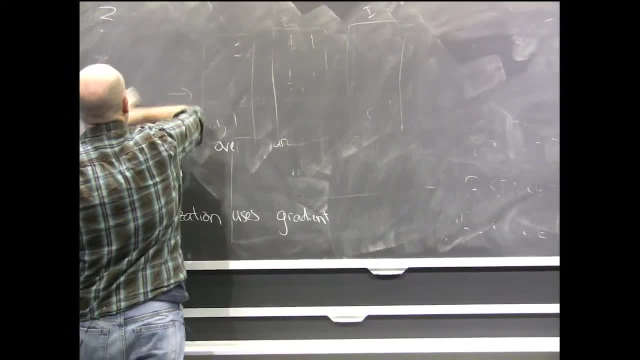 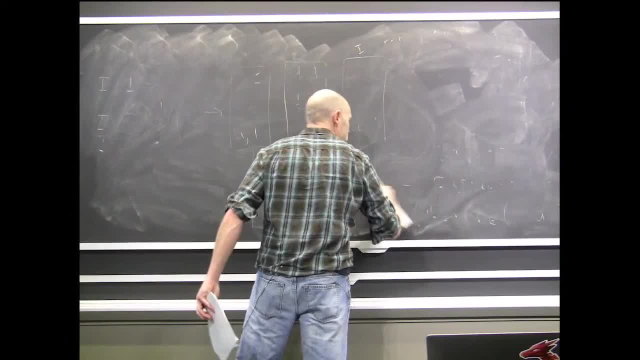 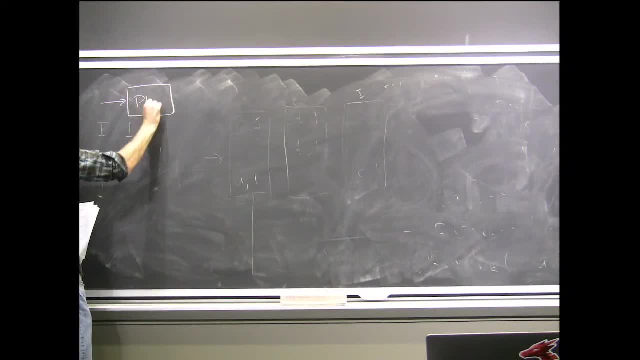 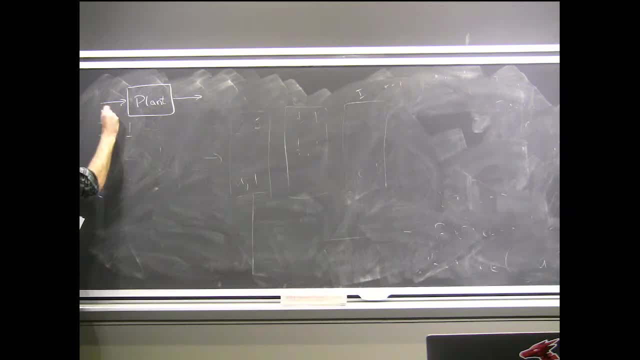 Okay. Okay. Okay. Okay. 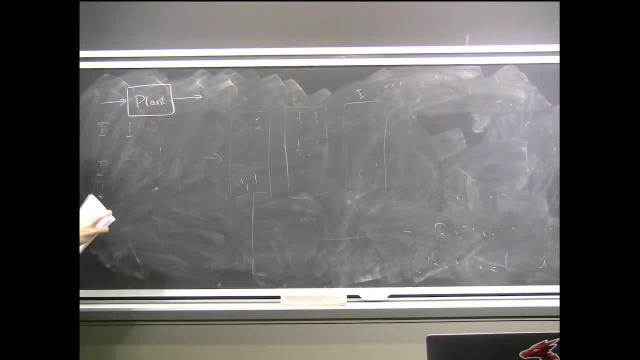 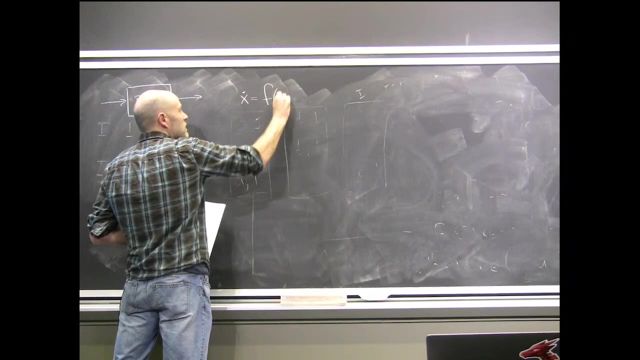 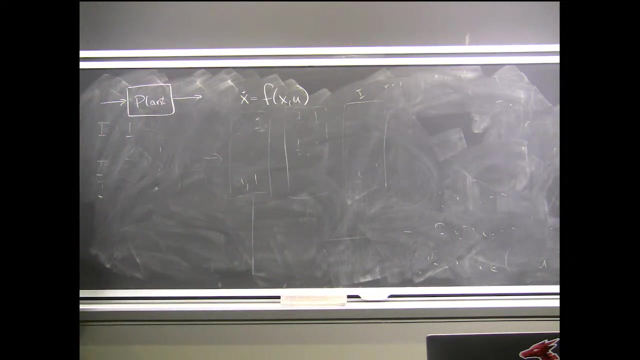 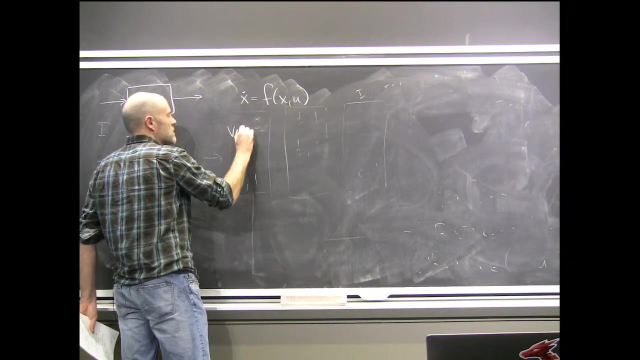 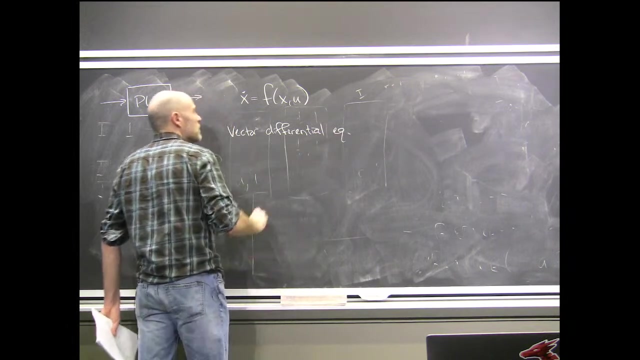 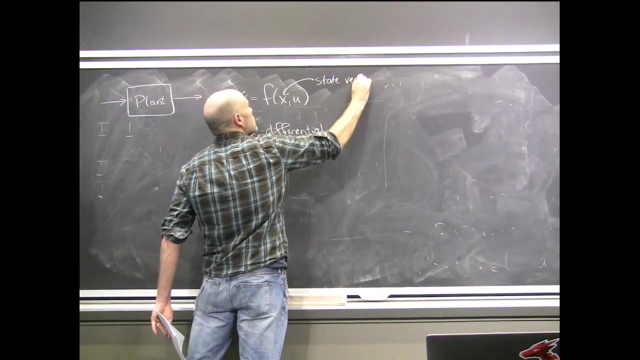 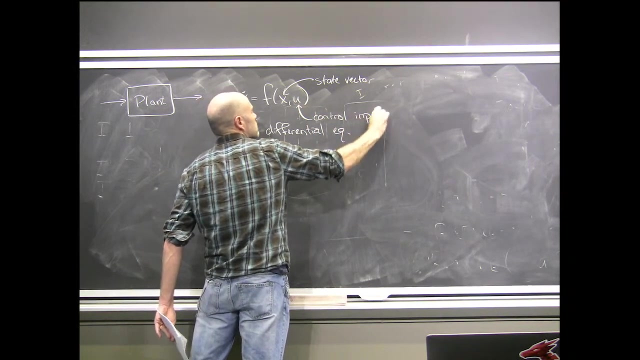 or actuator commands and output sensors okay but our modeling language for that type of system is going to be the language of difference or differential equations okay so I'll do the differential the continuous time version of it too you'll see me commonly writing equations that look like this form or slightly expanded versions of this form okay now this is a this is a vector differential equation right where this X here is called the state vector this here is our control inputs okay this is X dot . 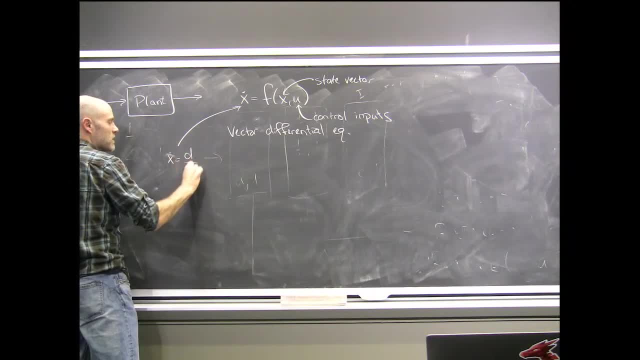 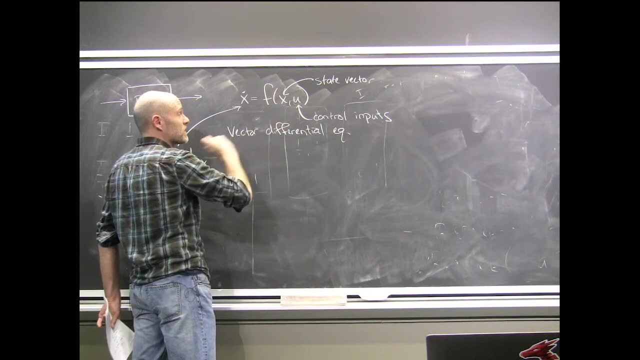 That is the time derivative. It's just dx dt of x, which makes this a vector-valued, potentially nonlinear function. It takes vectors in. It outputs an entire vector of time derivatives. 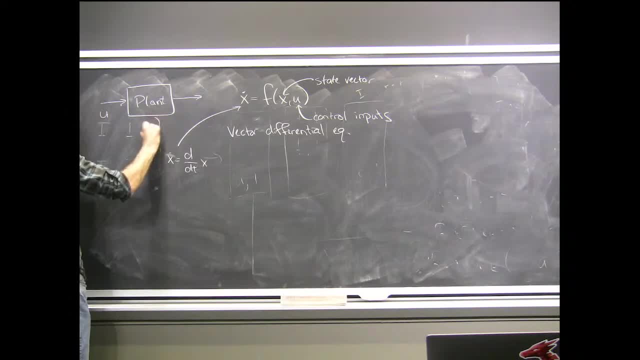 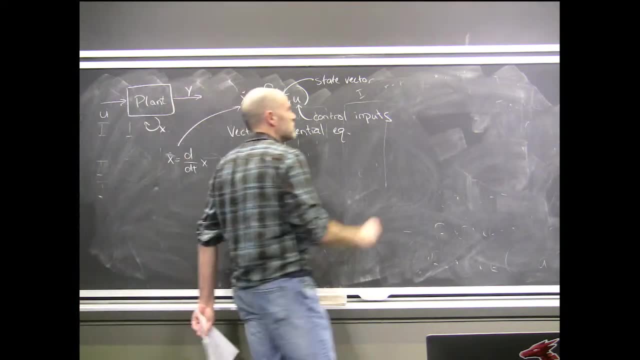 So this is u coming in. I'll often draw a little x in here, the state evolving. And then I'll tend to call the sensors y, which is some other vector-valued function here. These are the outputs. 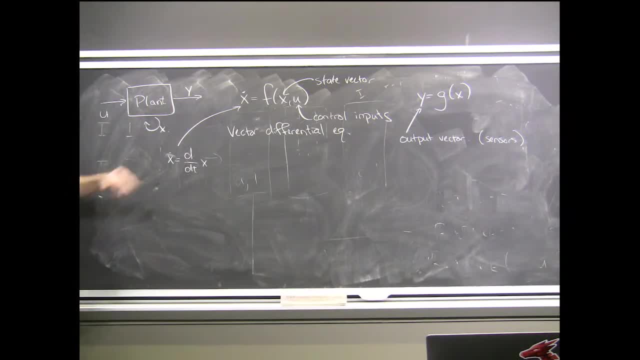 Actually, the controller, the other half of the diagram, we could use exactly the same machinery to talk about the controller too. But I want to focus today on the plant. Think about our robot dynamics. 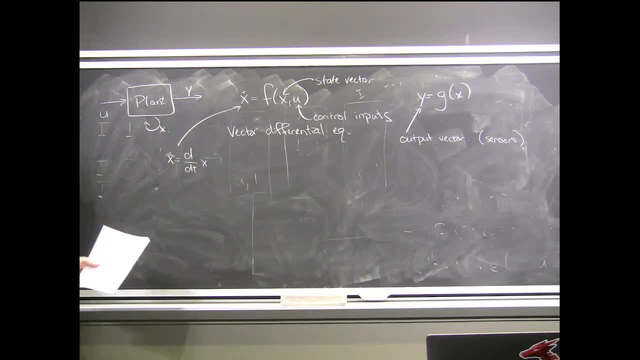 So there's one view of control, which is I should be able to control sort of any f. But that's too generic. 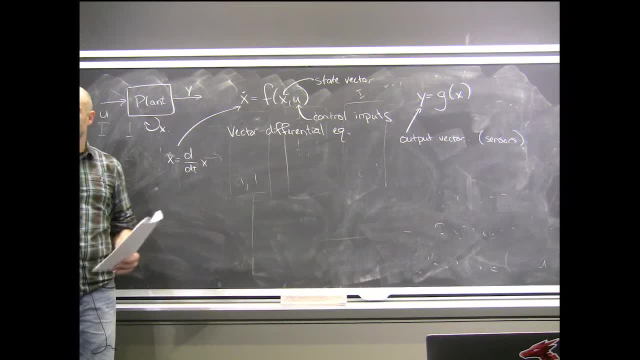 That's a very hard problem. The more structure we can add to f to sort of understand what's in there, the more strength our optimization will have, and the more our understanding will penetrate about what the problem looks like. 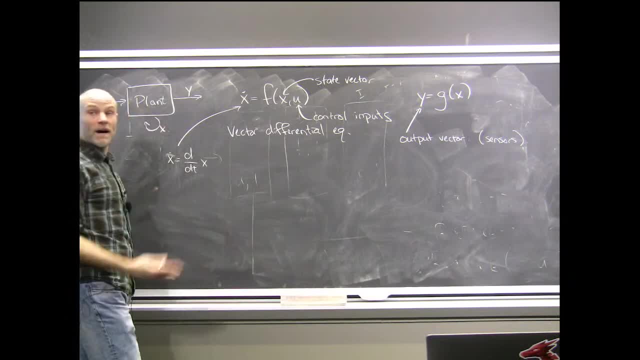 So it turns out that for most of us, we're going to be able to do this. So it turns out that for most of us, we're going to be able to do this. But for most of the robots we care about, we can do a little bit better. 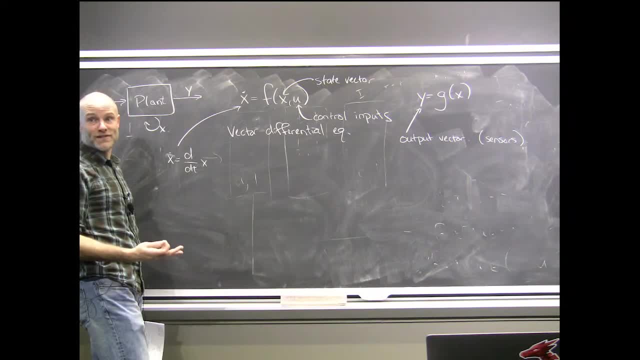 So most robots are governed by mechanics, Lagrangian mechanics. And so they tend to be second order systems. 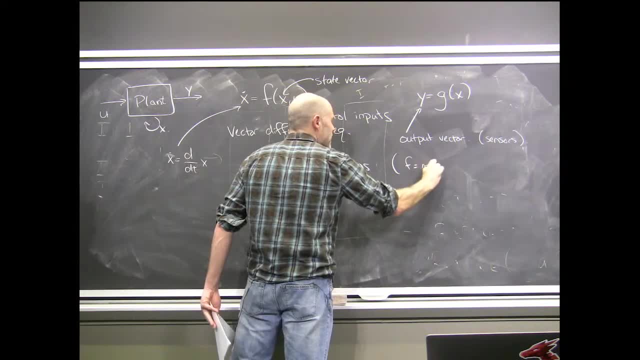 All right, fundamentally, we have f equals m a governing our systems. So how am I going to write that in this form? Oh, please, yeah. 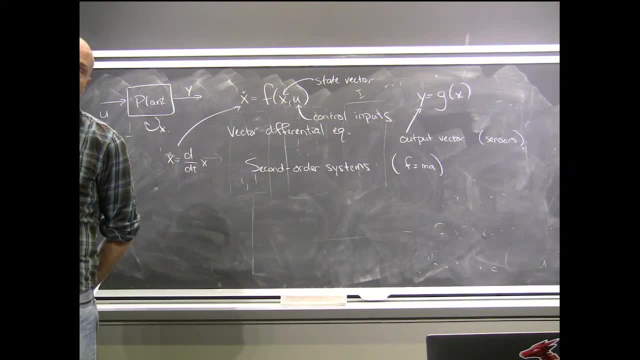 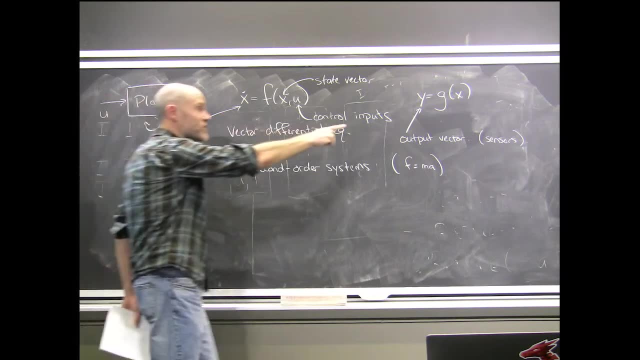 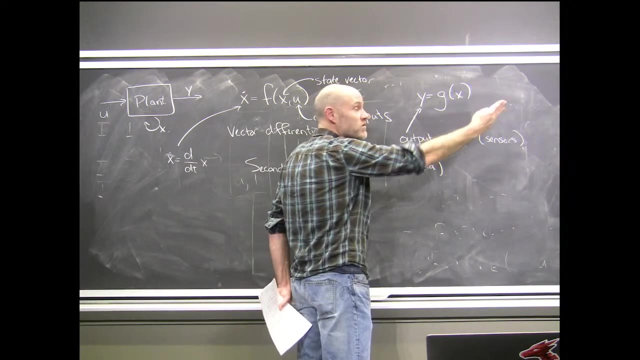 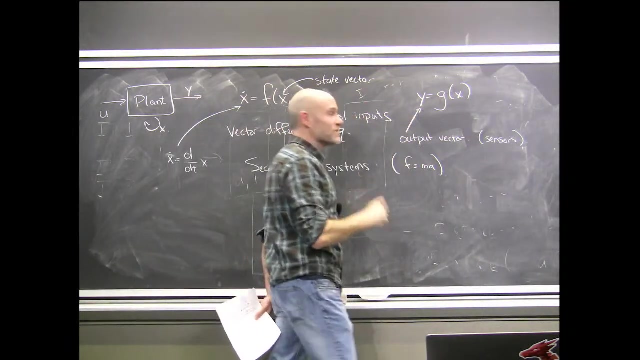 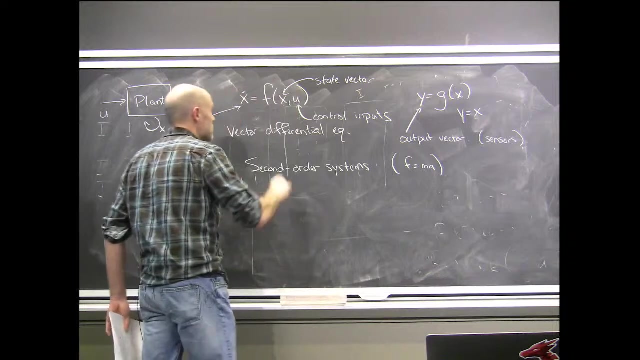 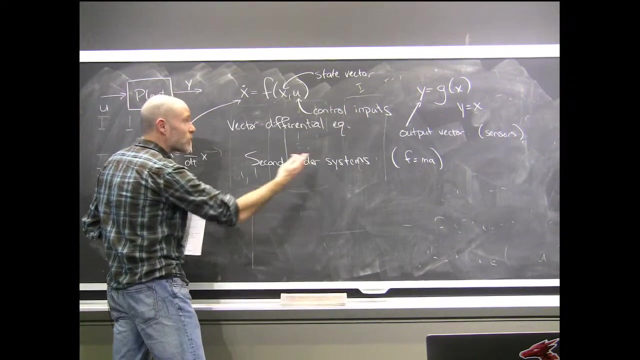 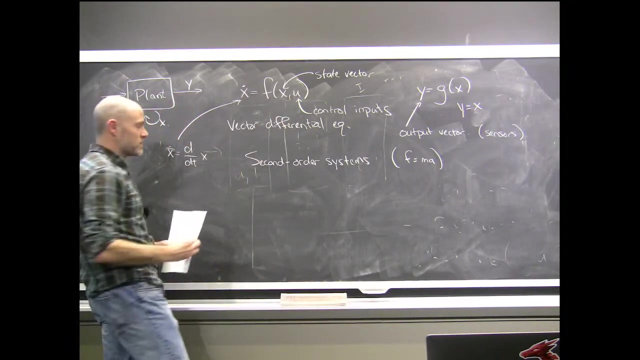 X is sort of hidden here. Good. So that's a good question. So that's right. So depending on what we assume for G, that's if G hides X, if it's not invertible, for instance, then that's where you get into the partially observable settings. And we will address that. But we're going to start by thinking about, let's just say G is even, you know, just for today, let's think about Y equals X. And then it's not hidden at all. Great question. But let's dig in first to this. Good. Okay. For second order systems, we're going to break it down and actually break the state down into positions and velocities explicitly. So we're going 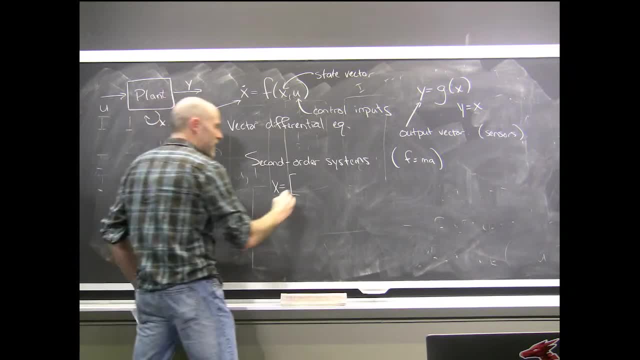 to say that the state of the system is completely defined by, I'll use Q as my notation. So this will be a vector of positions. 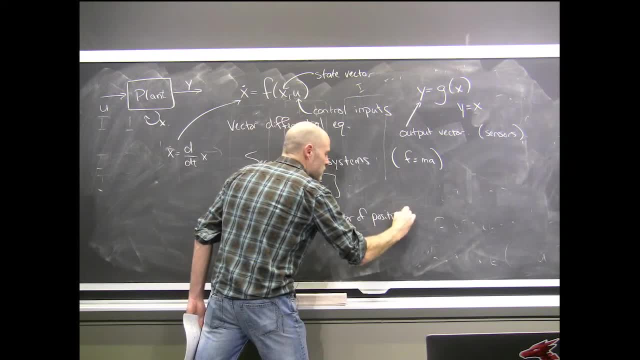 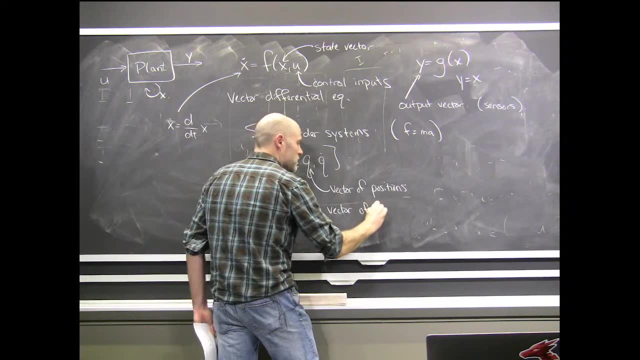 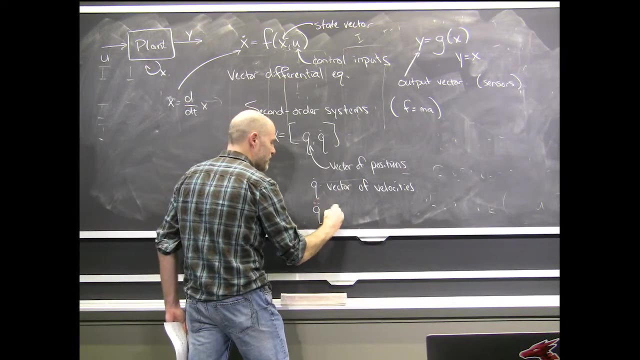 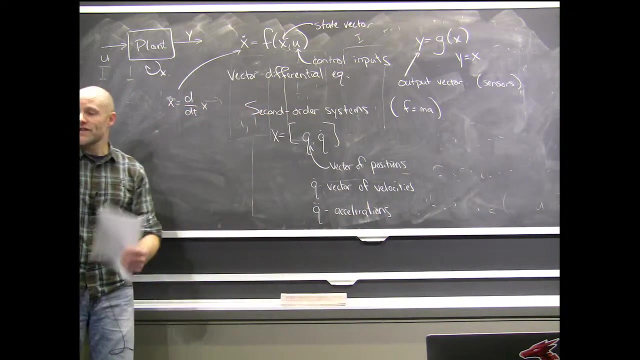 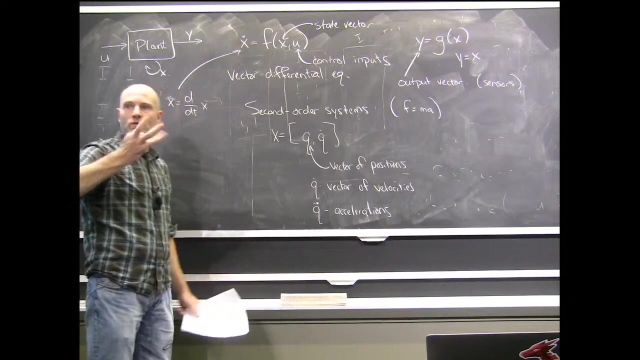 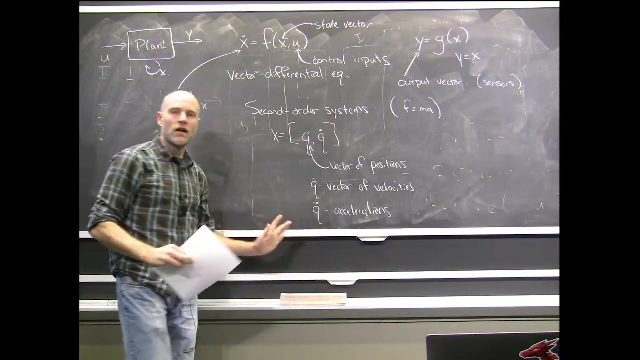 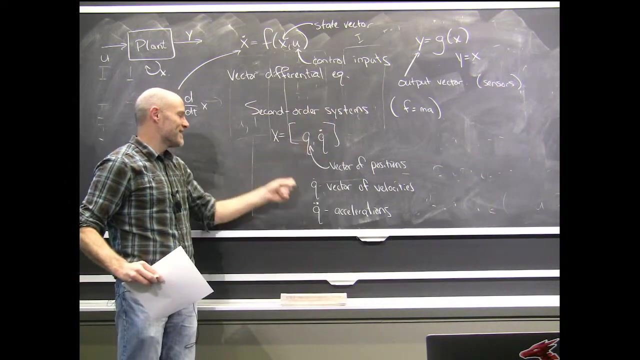 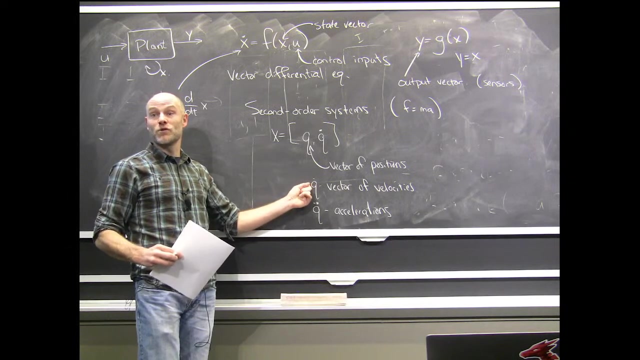 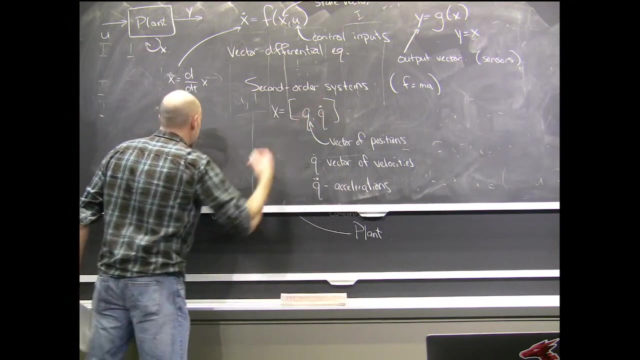 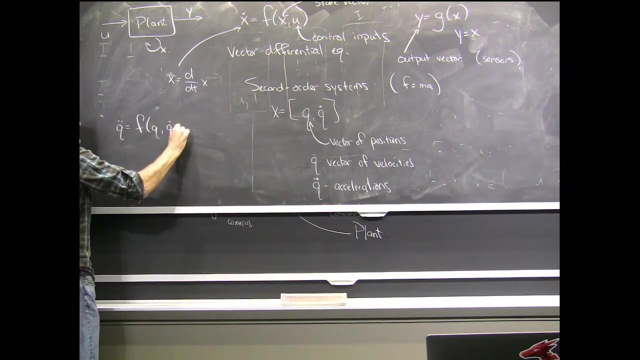 Q dot is a vector of velocities. Okay. Q double dot is accelerations, right? So Q, for instance, imagine if I have a bunch of rotary joints on my robot that I will just stack the radian measurement of each of those into a long vector list, and that will be the Q. And the joint velocities will be Q dot. I made a decision in this class. So there's cases where if you're doing 3D rotations and stuff that you don't want to, you want to be a little bit more careful about this representation, I can get through the entire underactuated material with ignoring that detail. So it's, it's, so for, in this class, Q dot, I'm going to, it's sufficient. Okay. If you know about quaternions and the like, you could be more careful if you have quaternions in your state. Okay. Once I've decided to have a second-order model, then the governing equations, I can start writing like this. Okay. Q dot follows naturally. 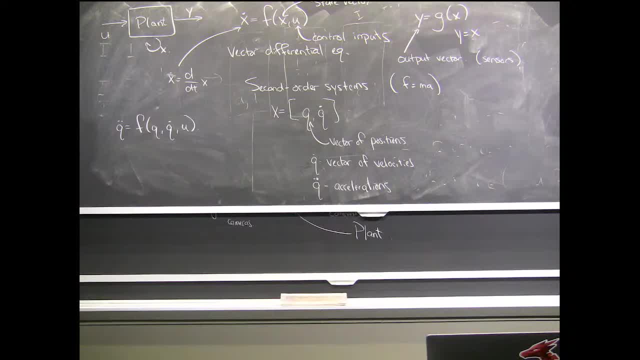 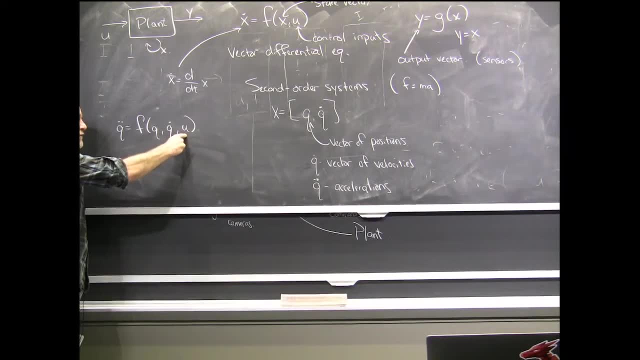 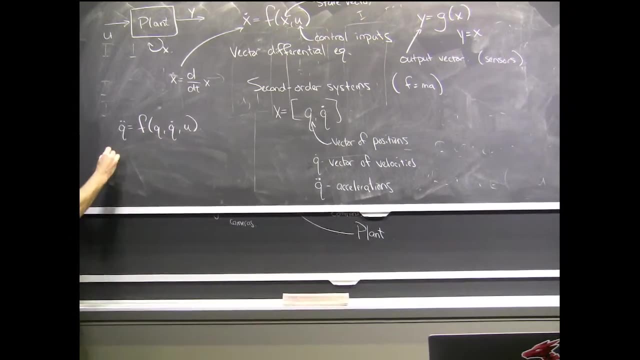 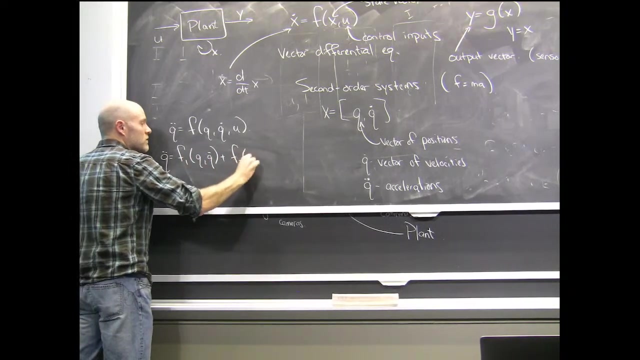 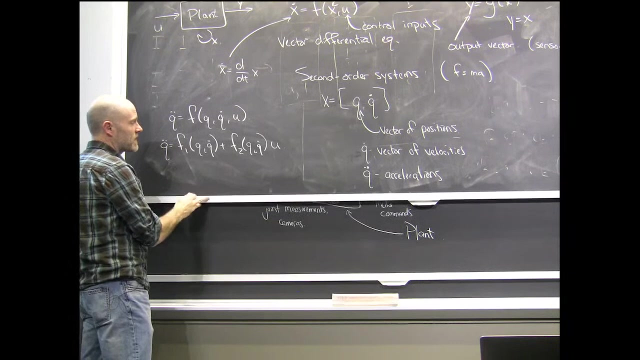 okay and then even more so if i'm going to get those governing equations from mechanics then almost always if i think about these as force or torque inputs which would be a standard output for my motor almost always there's even another level of structure that happens very quickly which is that almost always i'll try to convince you of this with the mechanics in a minute but 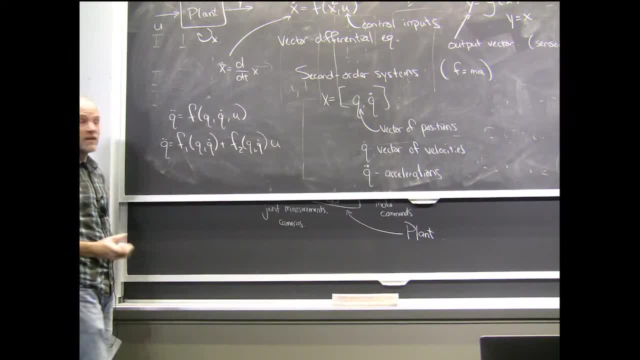 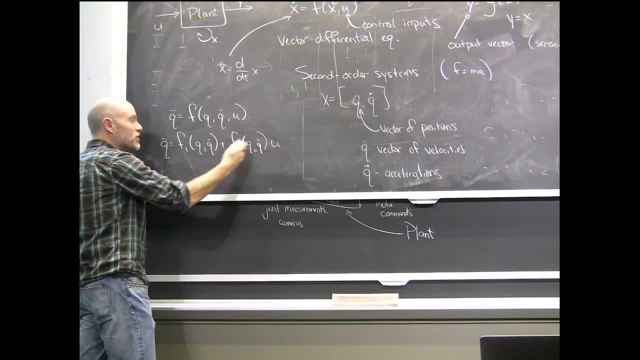 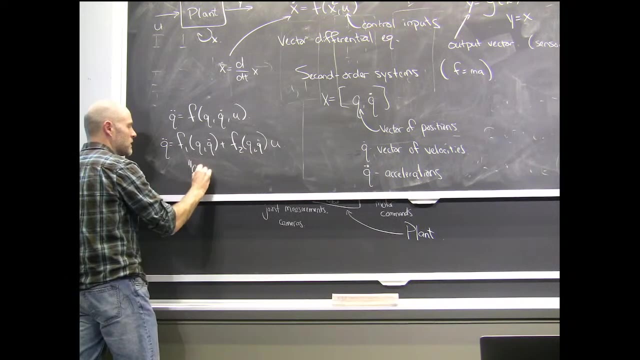 almost always the u enters in a particular way the equations are actually affine in u the only thing i'm from going from here to here is just saying that the way u enters the equation is not arbitrary it comes in just in an affine way so these are control affine second order differential equations 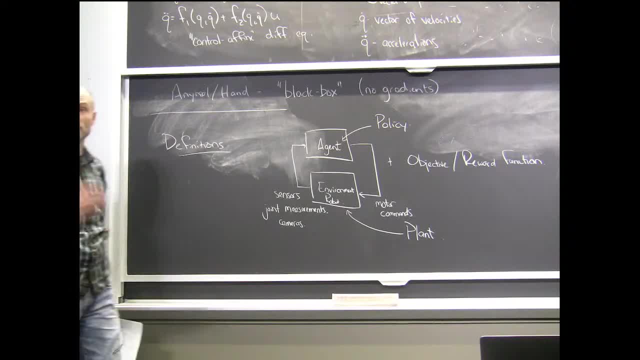 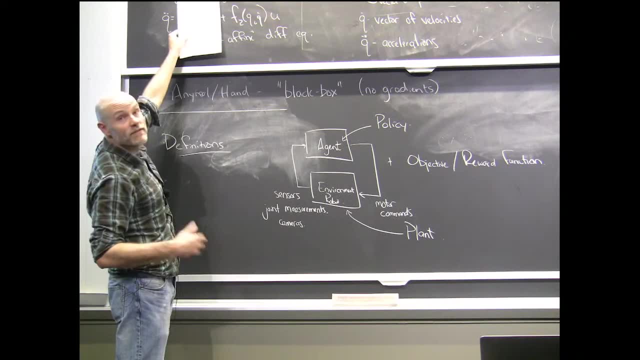 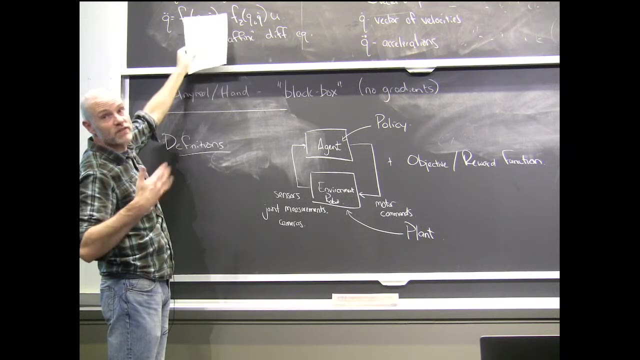 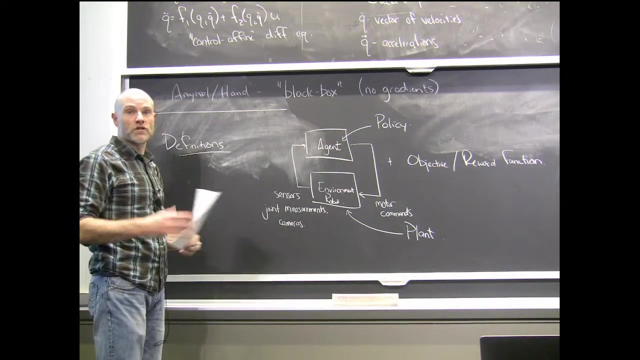 and for most of the robots we'll care about that's a reasonable model yes yep so linear would be if i just if i just had this then i have a linear relationship between u and q double dot because there's another term that's a potentially a constant so a linear plus a constant would be an affine function so in with regard with respect to to u that function looks like affine good question okay 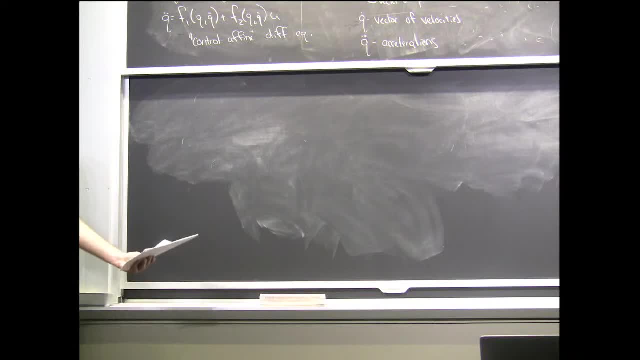 I don't actually have a answer if you if you permit me that equations look like that then I can define under actuated on this equation very easily and then we'll try to understand why that 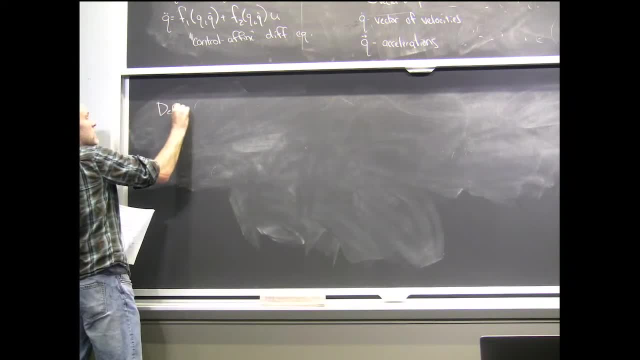 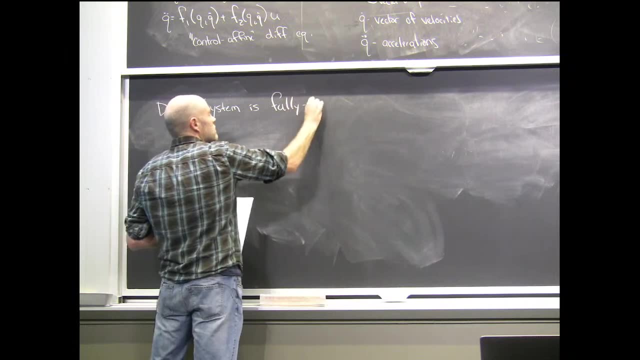 has all the implications I say it has okay so let me say a system is fully actuated if you allow me to say this is a system that is fully actuated 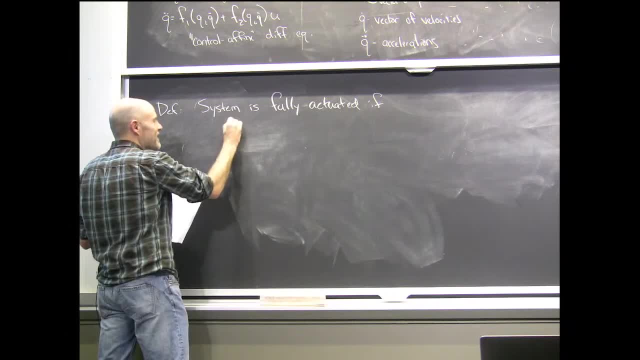 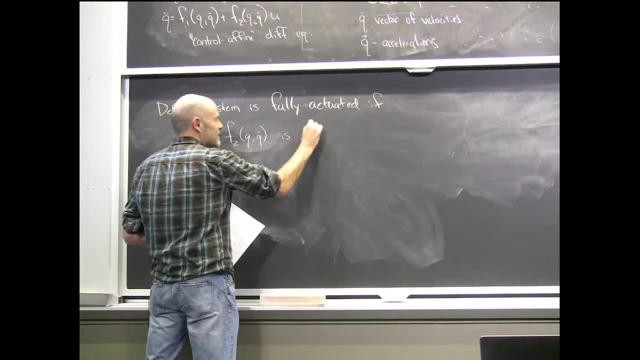 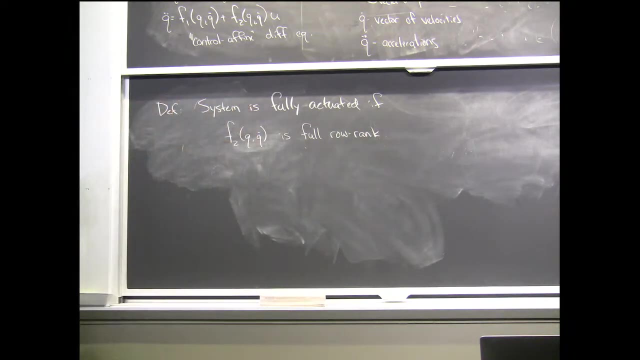 If f2, q, q dot, is full row rank, similarly, it's going to be underactuated. 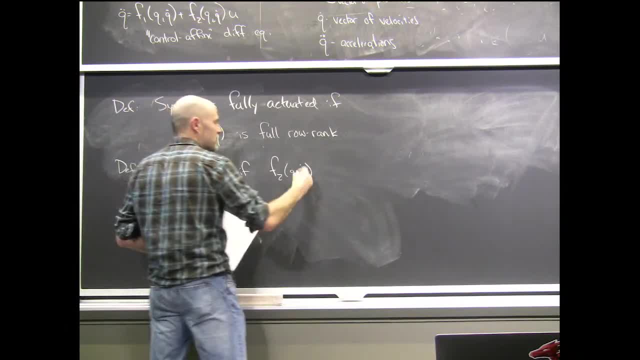 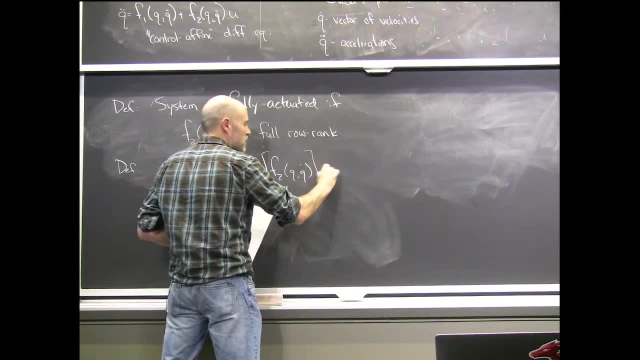 If f2, q, q dot is less, if the rank of this is less than the dimension of q. So let me unpack that. So first, let's just make sure we understand the mechanics of it. 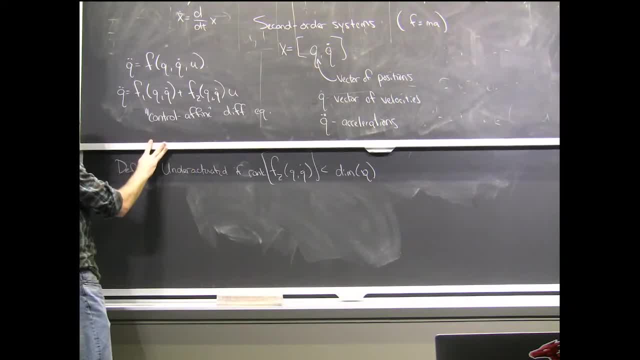 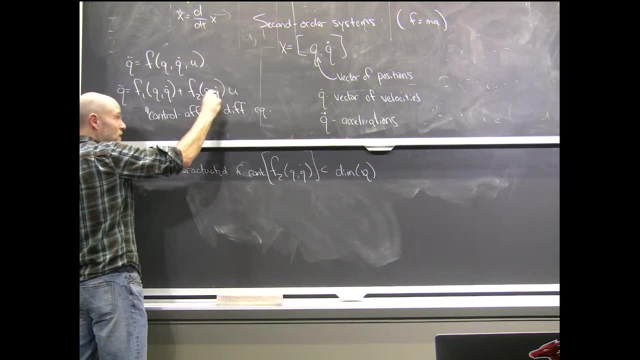 So if I were to put in any q and q dot, then this thing here, this is a vector. f2 is actually a function of q and q dot. It outputs a matrix times a vector. So this is a matrix. Its size is on the right side. It's going to have the number of columns is the same as the dimension of u. 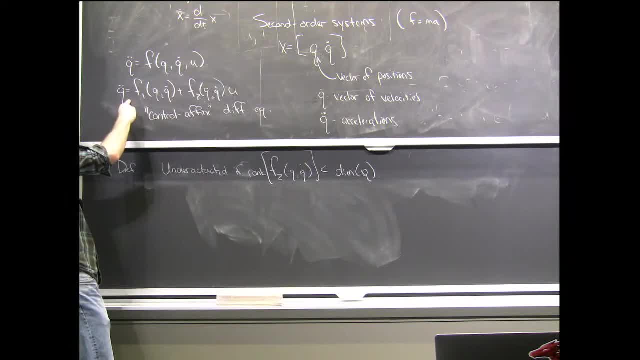 The number of rows is the dimension of q. So this is potentially, it doesn't have to be a square matrix. 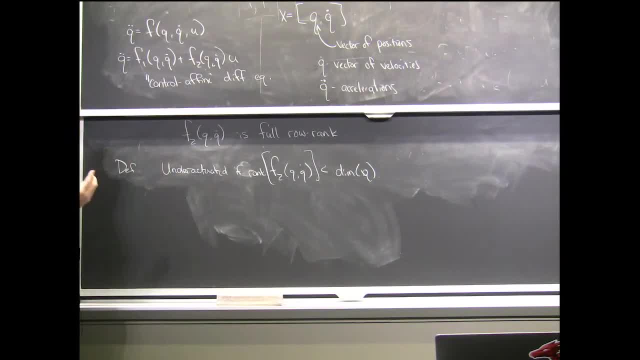 And it doesn't have to be a full rank matrix. So I can ask the question, when does that matrix, for any particular q and q dot, I can ask the question, is that matrix full rank? Which would mean that it has to have the rank of the number of rows, full row rank. 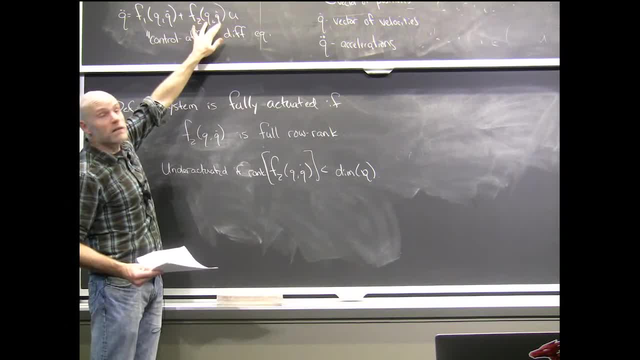 And my claim is that, so that's going to be a function of q and q dot. 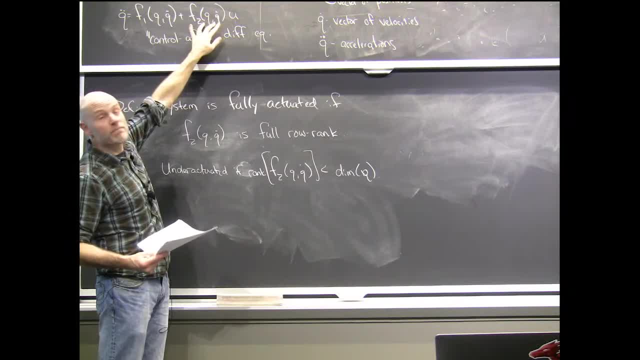 But we'll see that most of our systems either have that property for all q and q dot. 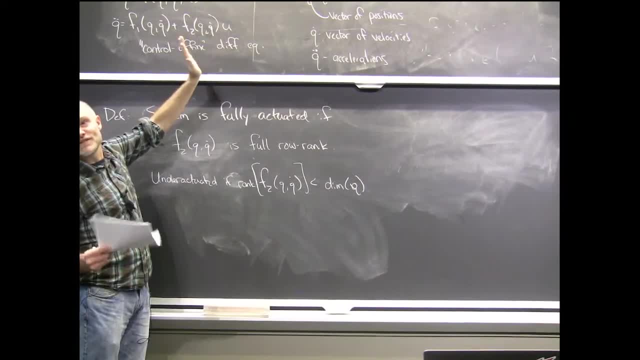 Or for no q and q dot. There's a few subtleties there about singularities and stuff. 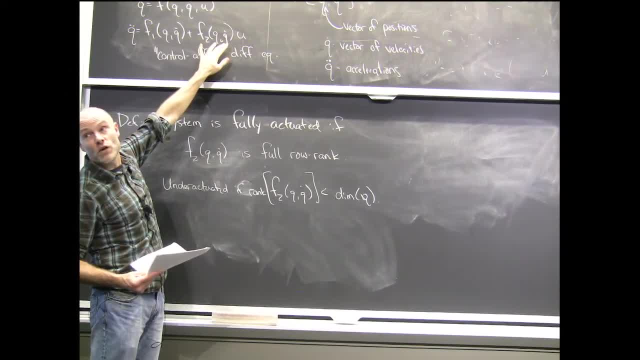 But roughly, we're going to generalize the notion from a state-dependent notion to a system-dependent notion. So that's a matrix. 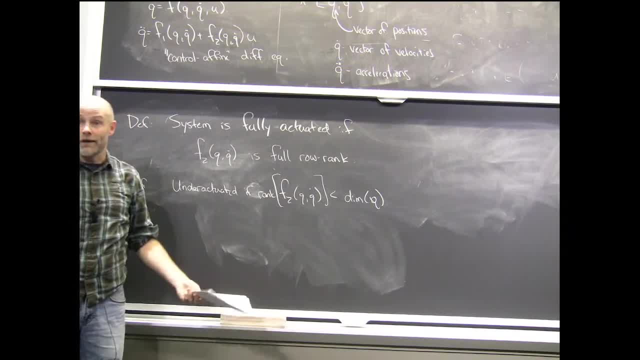 My claim is that the rank of that matrix affects whether control is hard or not hard. 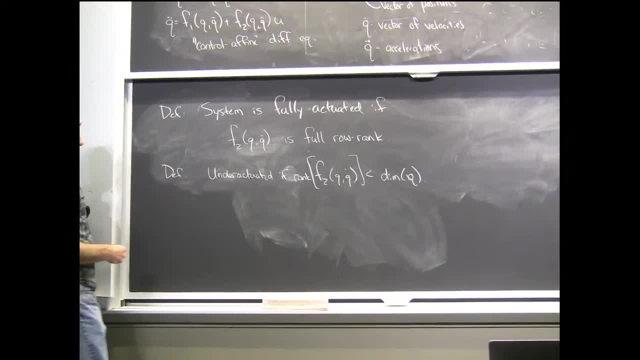 Why is that? The reason for that is because of a trick called feedback equivalence. 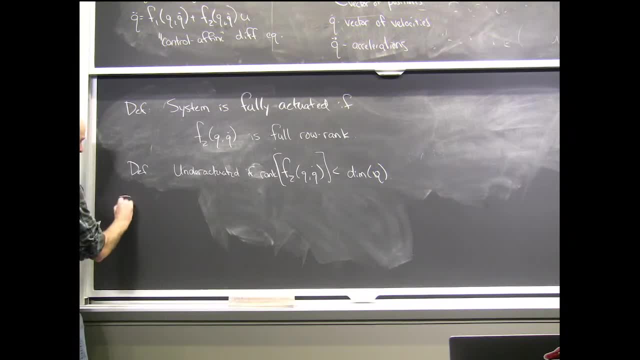 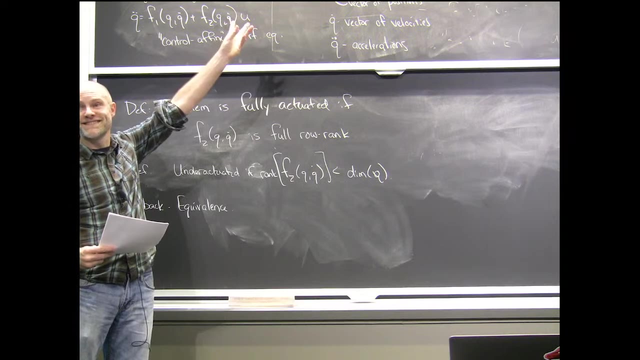 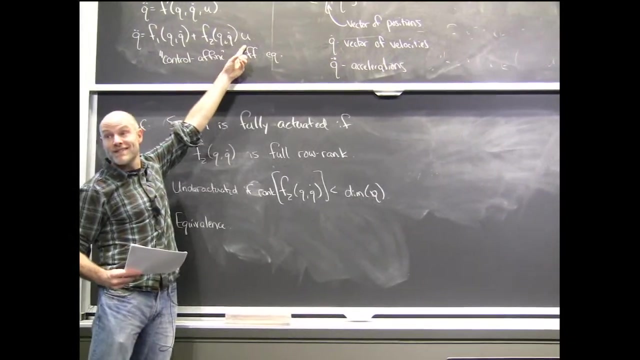 I think the intuition actually goes back to your question about if g is invertible, then that problem is sort of easy. And the same kind of thing is going to happen here, is if f2 is invertible, then choosing the right u to make q double dots happen is easy. That's the big idea. Right? 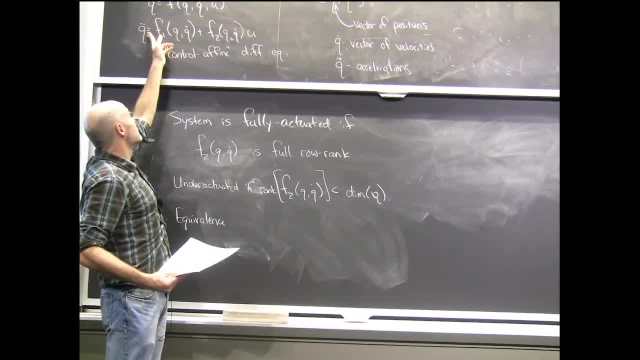 If this is invertible, then if you have a desired q double dot, then finding the desired u is easy. 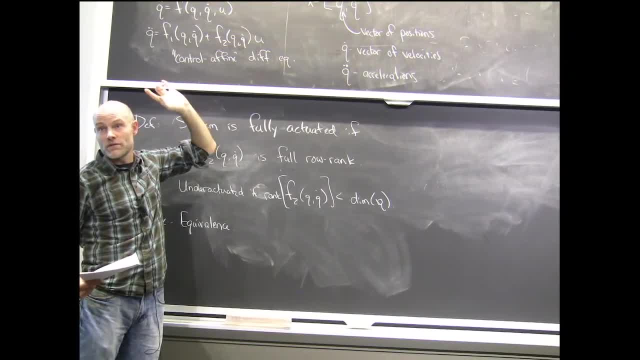 When it's not invertible, then you have to do more work. Right? And this is an invertibility condition. Yes? 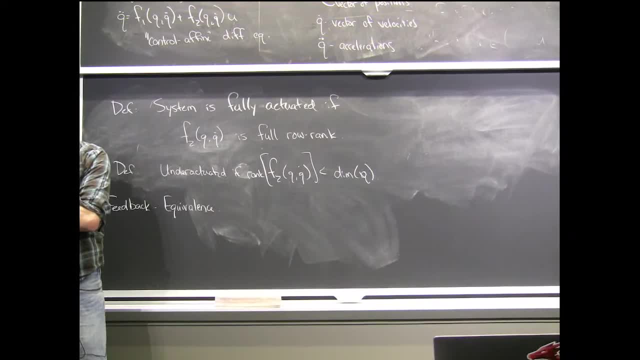 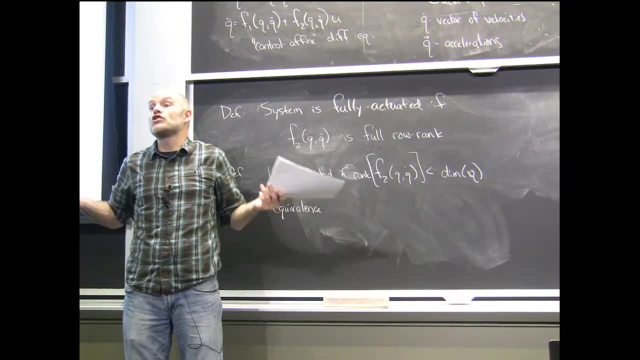 In scenarios where it's overactuated, where it has full row rank and not full column rank, is that still easy? It's still easy, but you get to make a choice in your redundant degrees of freedom, or redundant actuators. 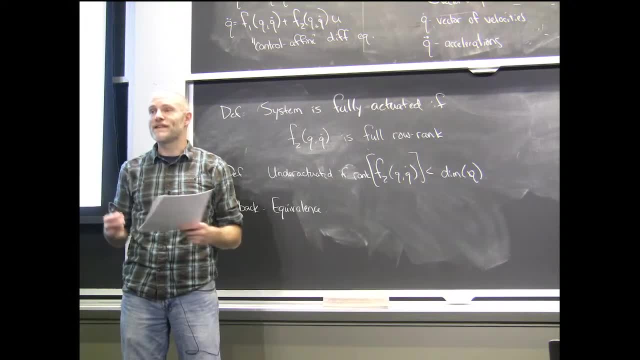 OK. Yeah. OK. Yeah. You have to do some work to make that choice, but that's still an easy case. Yeah. 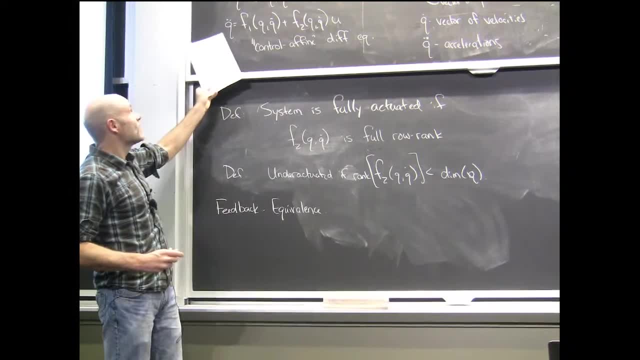 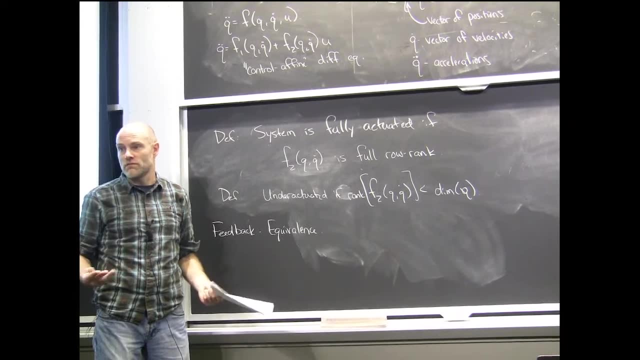 So if this is invertible, then if you give me a desired behavior of the robot, then I can just invert f2 to make that happen, roughly. 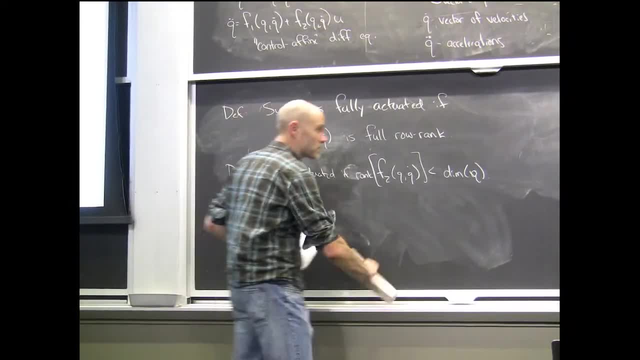 Right? So I'll write that. Maybe I'll come over here to leave that up. 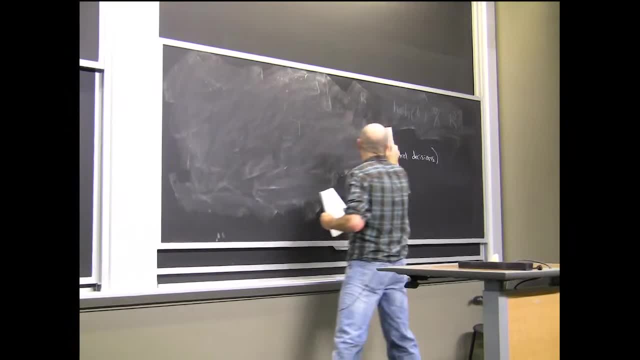 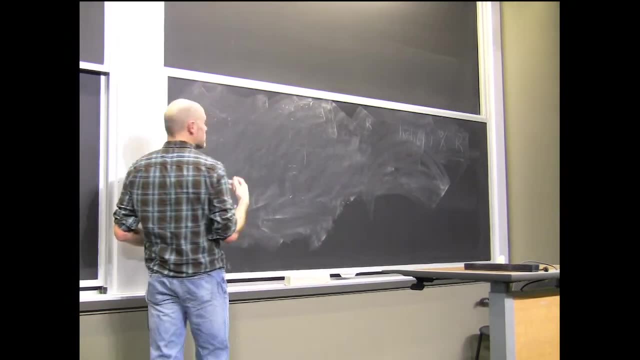 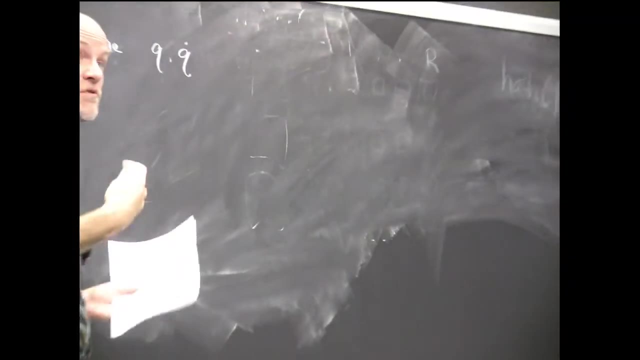 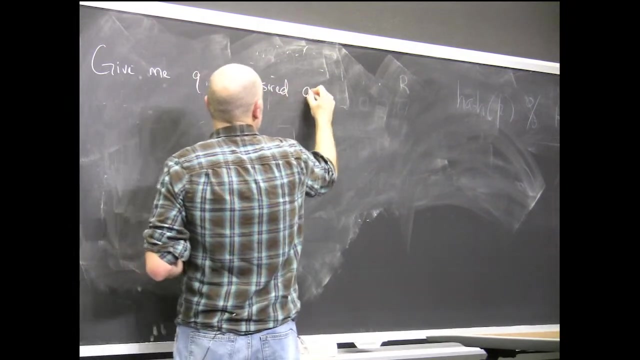 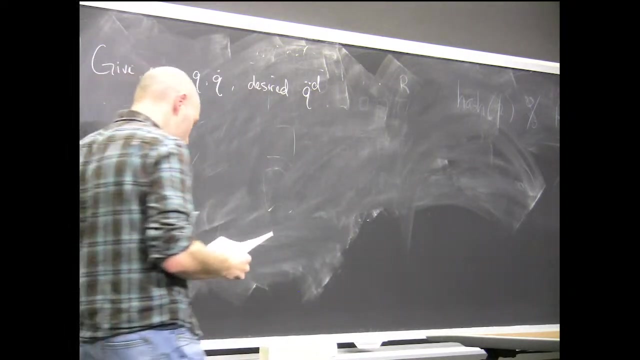 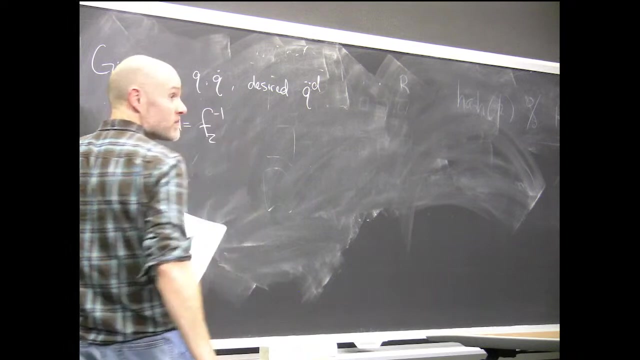 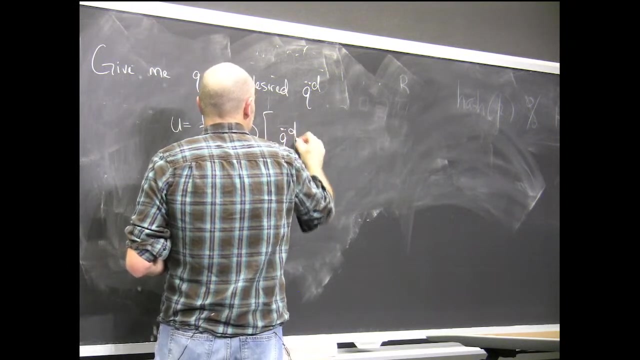 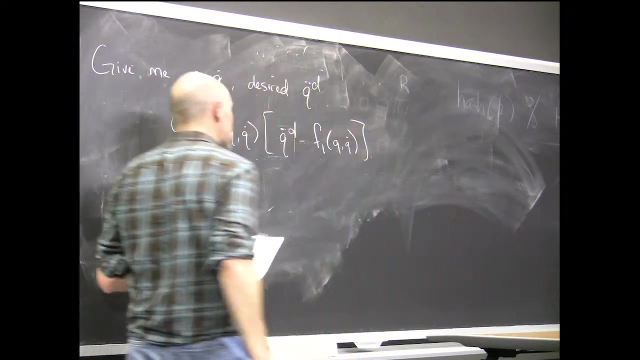 Let's say if you give me q q dot, which is the current state of the robot, and a desired q double dot, I'll write q double dot desired as a superscript. OK. Then if I were to just choose that u is f2 inverse, q q dot, times q double dot desired, the algebra has to go through, but then that implies, if I were to stick this back into that equation. 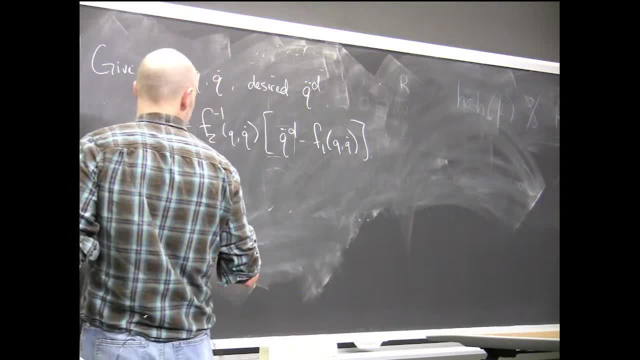 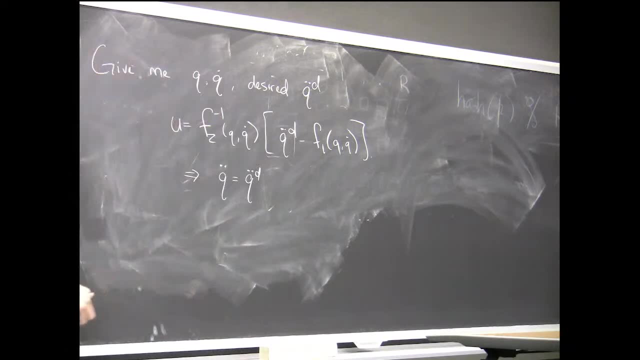 OK. Then if I were to stick this back into that equation, then that implies that the q that actually happens is whatever I desired it to be. I can just, whatever acceleration you want, I can provide it. Right? And the only condition there is that this f2 is invertible. 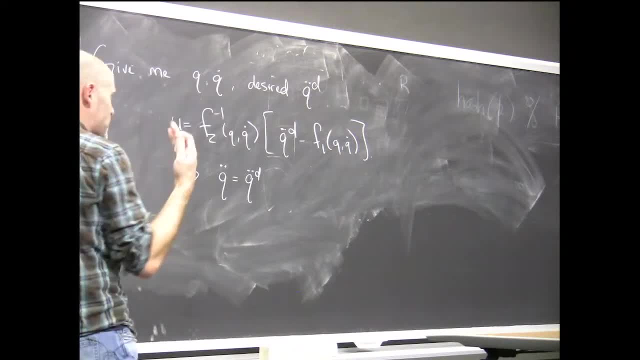 Because of this, we're going to say that fully actuated systems are feedback-equivalent. 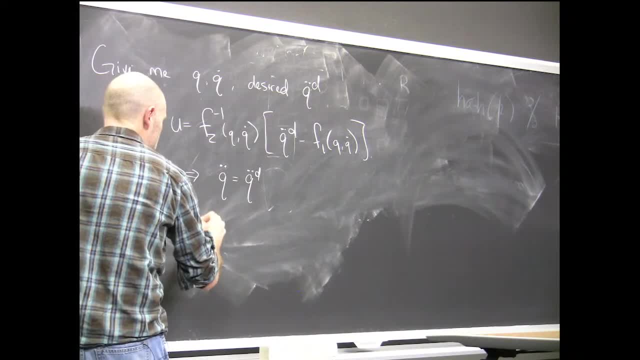 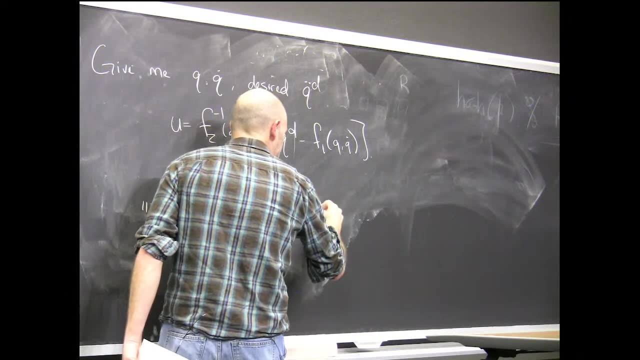 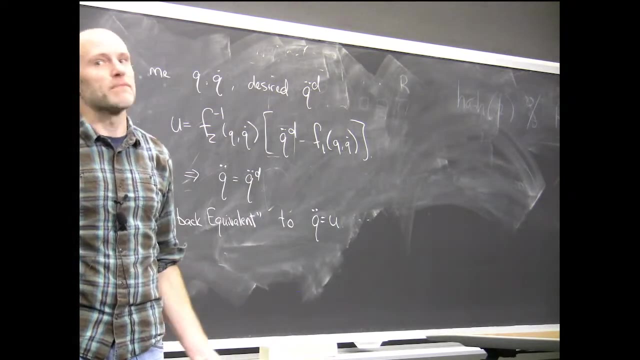 To the system q double dot equals u, which is a sort of a trivial diagonal linear system. It's still second order, but we know a lot about how to control that. So that makes control easy again. 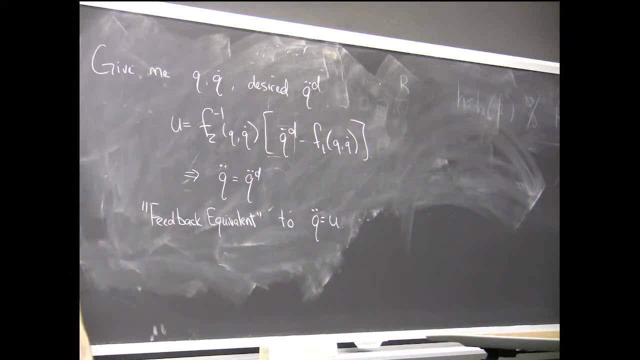 When it's not invertible, the under-actuated case, then I have to do more in order to achieve some longer term objectives. 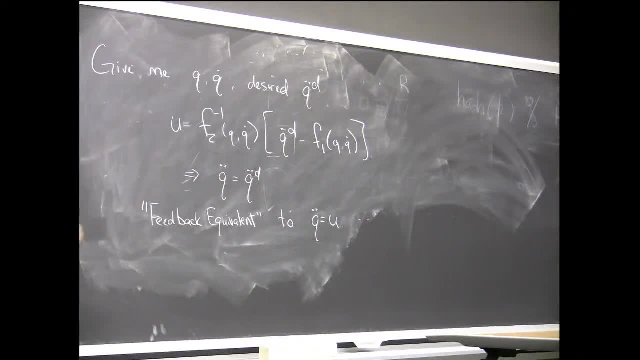 There's kind of another way to say, if you're coming from the learning or optimization view of it, I could say it maybe differently. 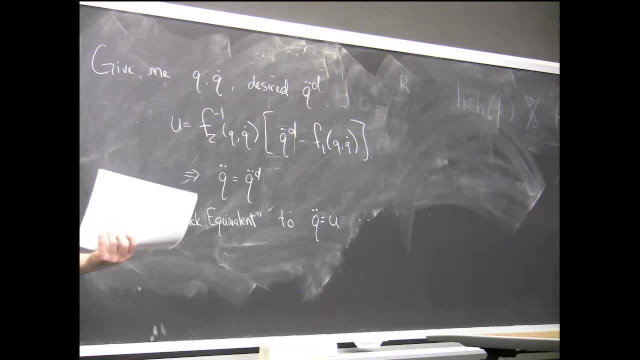 I could say, if the system is fully actuated, that we know a change of variables that makes the optimization landscape easy, convex, for most people. But when it's not invertible, I have to do more work. 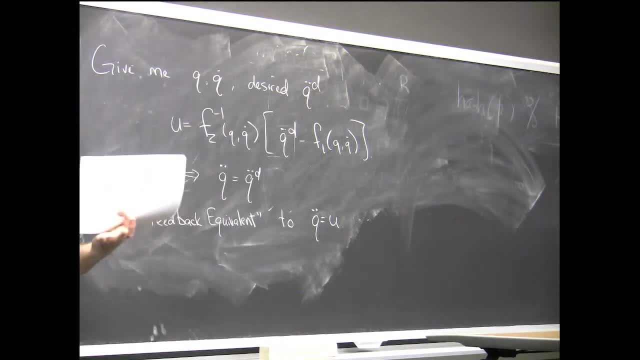 There's exists a simple change of variables that uses this inverse that makes the optimization landscape easy. But when it's not invertible, then I have to do more work. What's surprising maybe? That doesn't seem surprising. 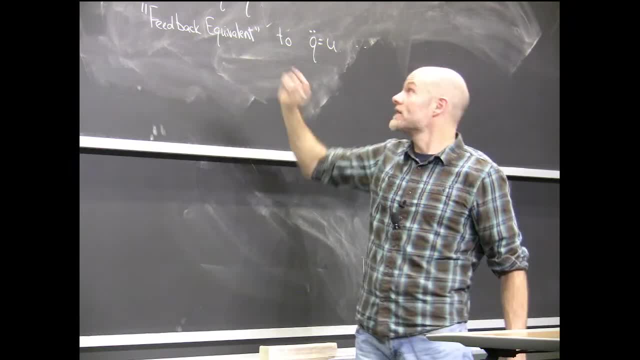 I guess what's surprising is how far we got in robotics without considering that case. 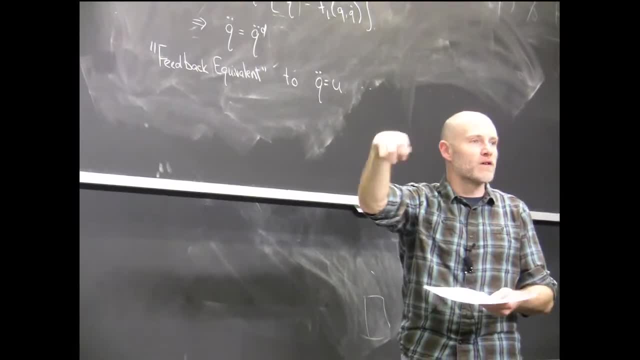 Because a lot of robots. All the robots that were on the assembly room floor, or even doing pretty dynamic things with a robot arm, 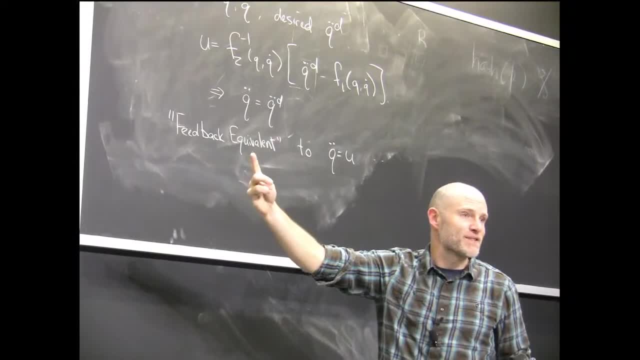 F2 is invertible. But once you started starting back flips and other things, then that assumption breaks. And we'll see that. 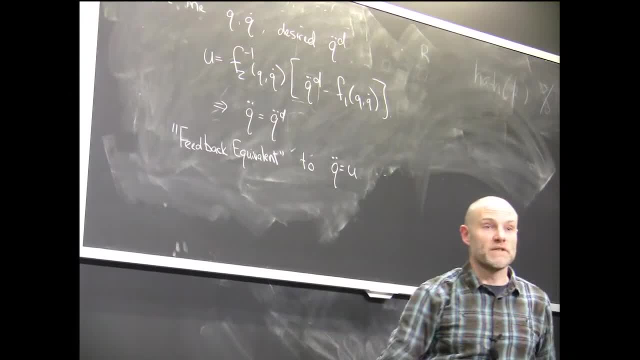 And then we have to think about this more interesting problem. Yes? 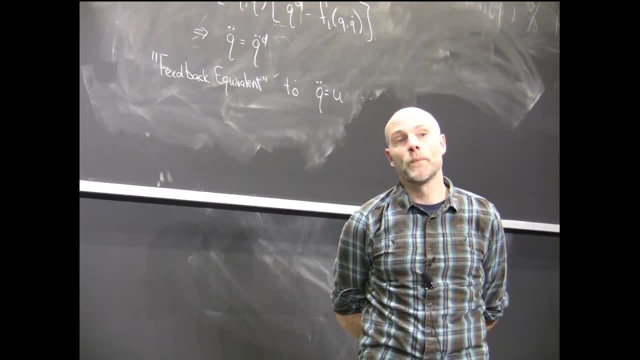 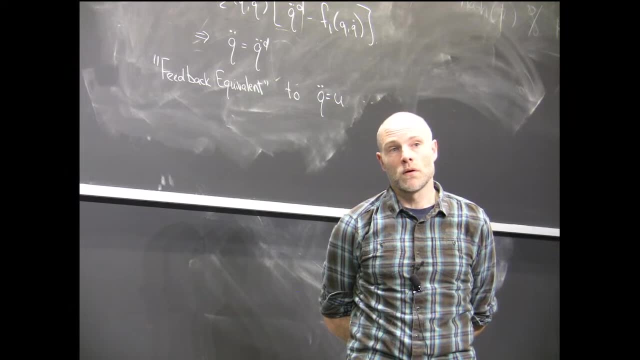 Can you sort of express the whole concept of feedback equivalent in sort of system reachability? Or is there a bit of a difference? Yeah. 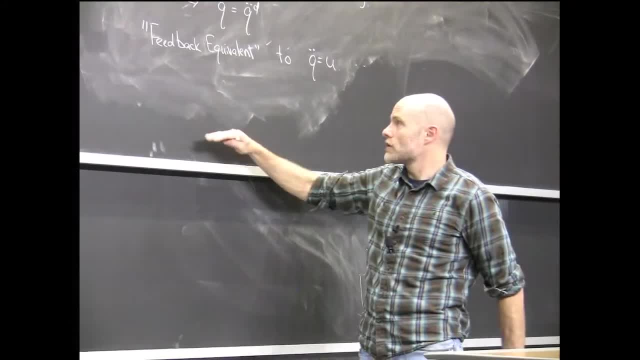 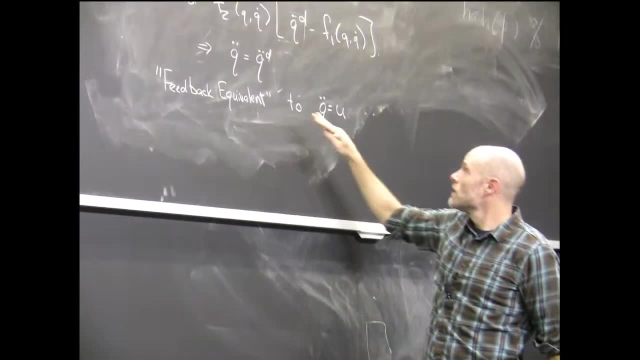 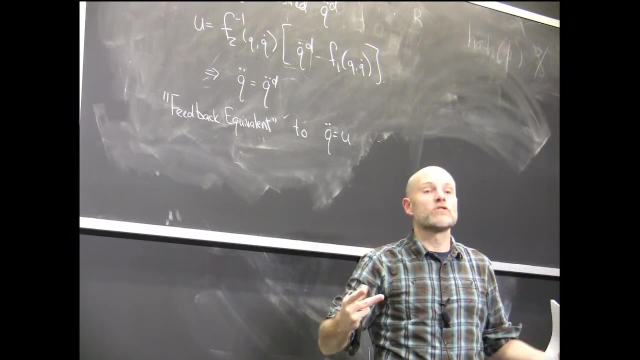 So the question is, can I talk about feedback equivalence with the language of reachability? So I think what it would say is that there's a basically the idea is that I could write two controllers. 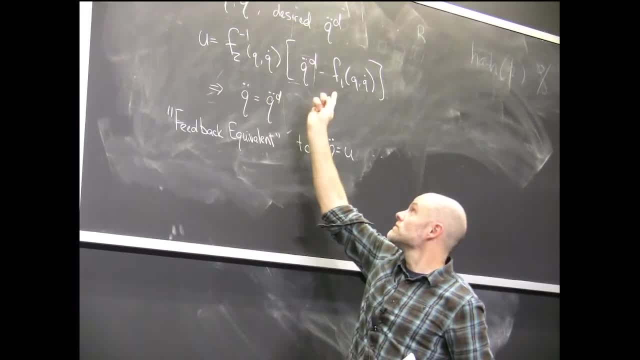 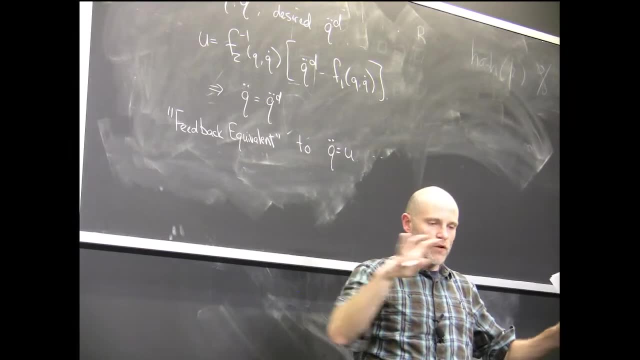 The first controller is this form here. The second controller could set Q double dot. So that the system, which involves my low level controller, and the plant, looks like this. 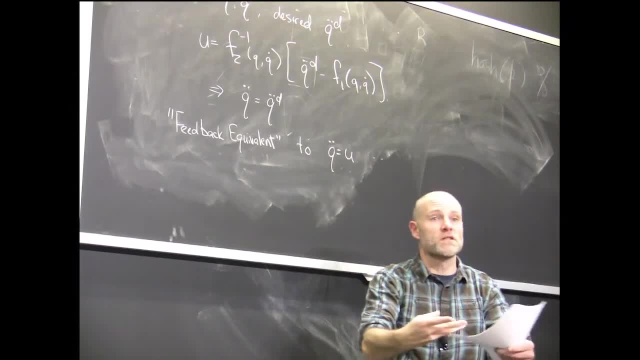 So it would say the reachability of that closed loop system would be equivalent to the reachability of this, which we understand everything about. 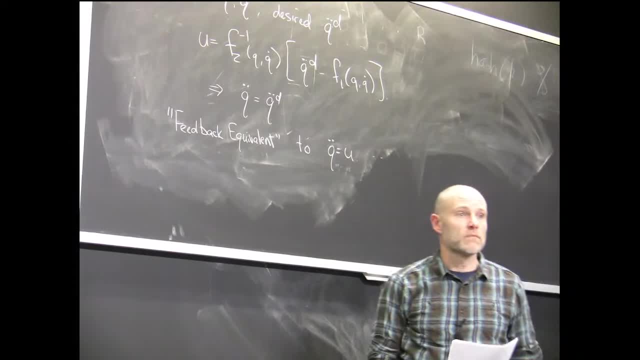 I guess that's the way I'd like to connect those two ideas. Yeah? 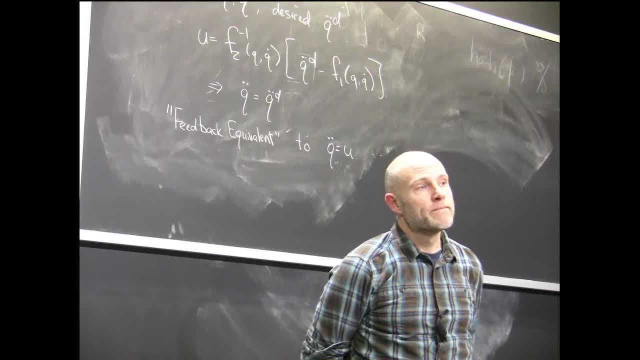 Yes? What instance might you ask for determining 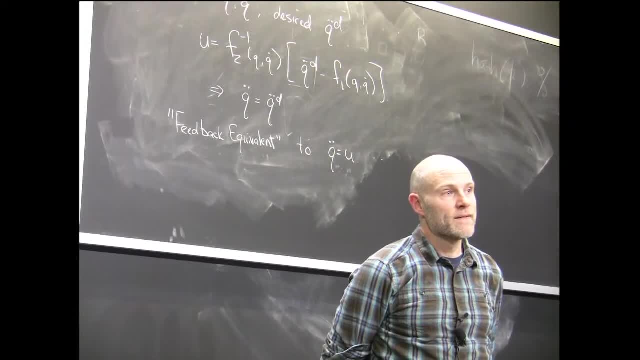 if your system is under-axilated? If there are things in the system that are under-axilated? Oh, good. Good. That's a great question. 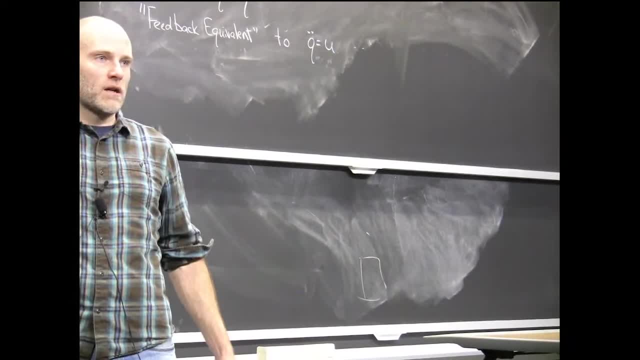 So if the system is not control affine, then what tools do we have? What tools do we have to make sure that it's under-axilated? 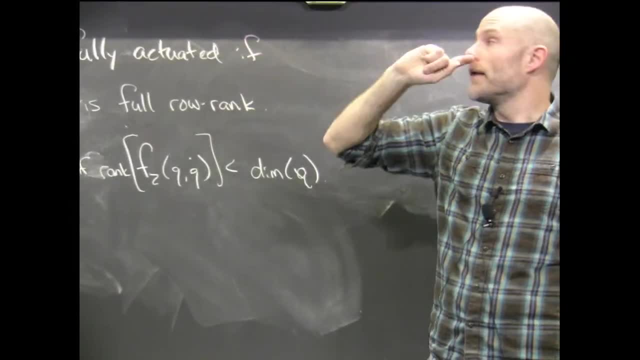 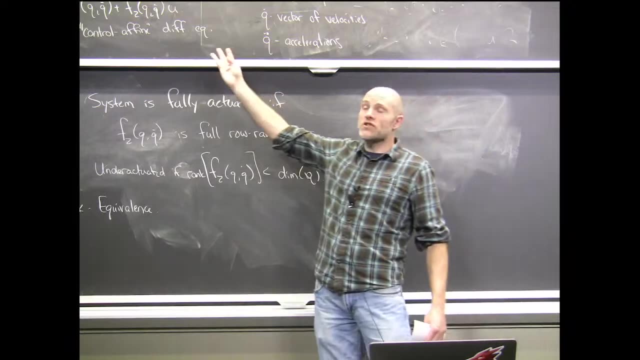 So I actually put a careful version of that in the notes. It also gets rich if you think about higher order derivatives. It's not just a second order system. So I think the generalization of that is roughly talks about the rank of the derivative of the highest derivative. 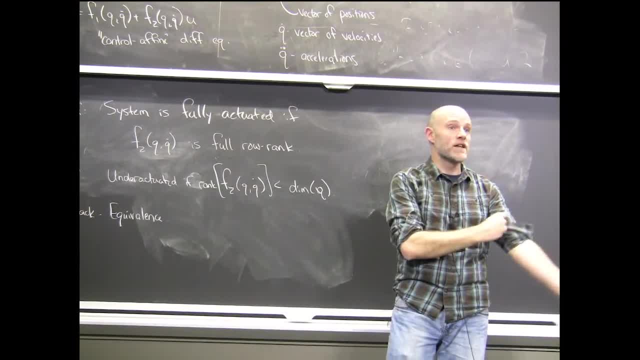 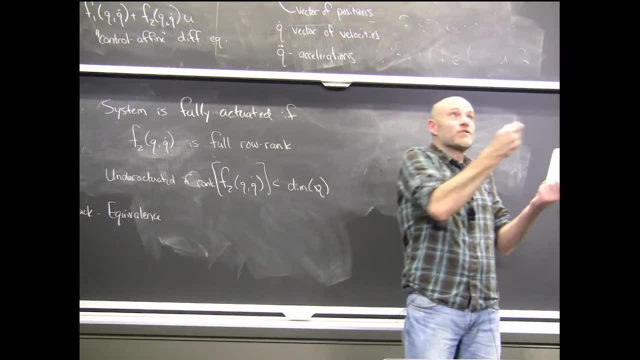 And I tried to write it carefully in the notes. So I do think there's a way to do that. But most of our robots don't need that extra machinery. It's roughly, can you control the highest relevant degree? It's roughly a degree of a derivative, completely. 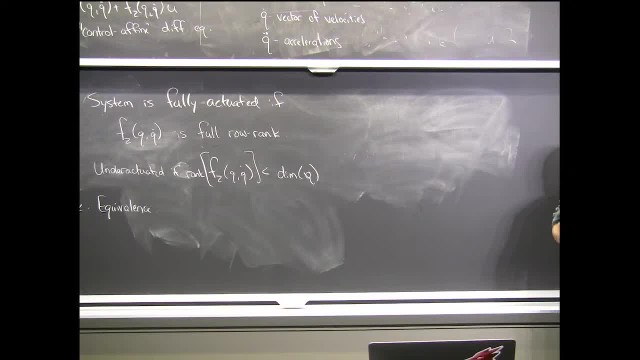 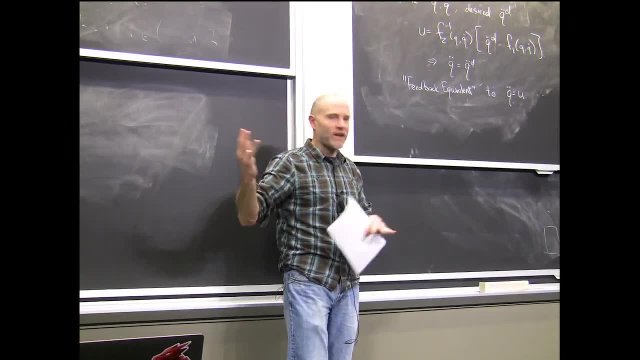 OK, there are other things that make control interesting. I picked under-actuated almost because of the history. The people that were thinking about making walking robots work and making interesting dynamics work were the ones that were thinking about this under-actuation problem. 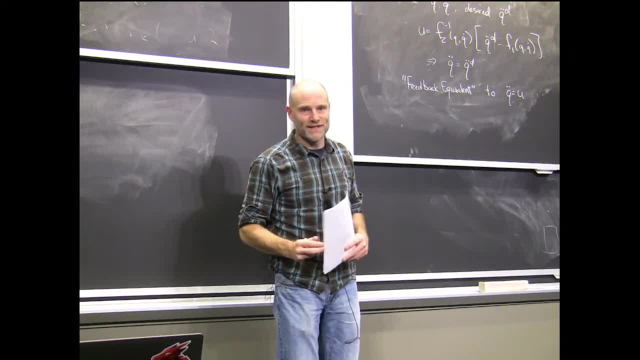 But it's not the only thing. I will admit, it's not the only thing that makes robot dynamics and control interesting. So if you have. 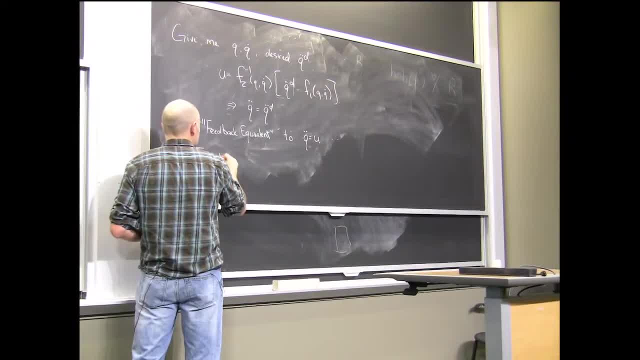 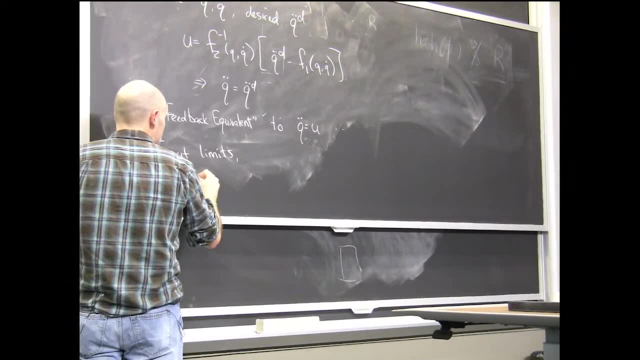 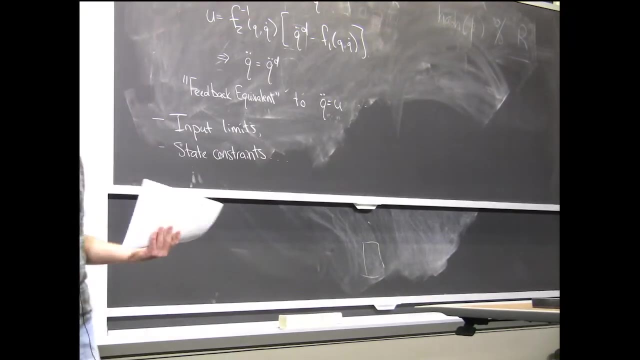 Input limits, torque limits, state constraints like you have for collisions or contact dynamics, for instance, these all also can cause you to have to make long-term reasoning decisions in order to accomplish a task. 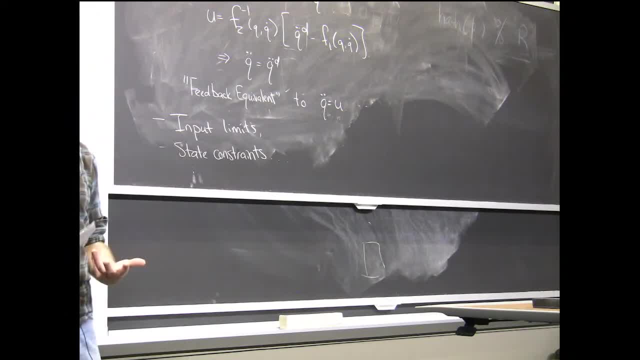 So it would prevent you from just saying that the system is equivalent to a linearization. But I think the. The. The. 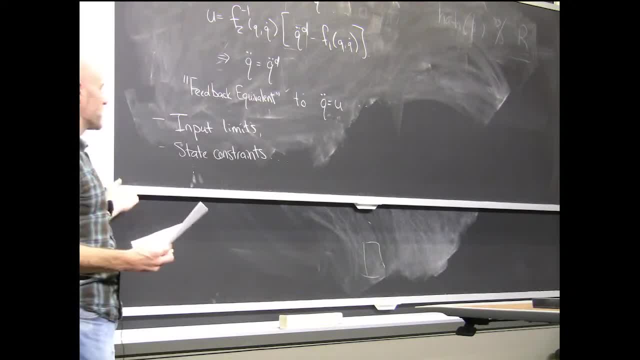 I think this is maybe the one that we'll lean on right from the beginning. Many of those will fit right into our constrained optimization framework. 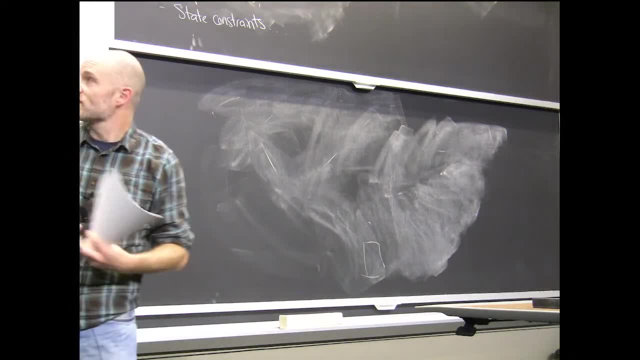 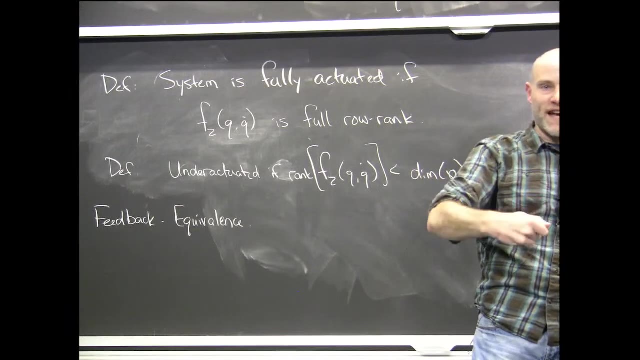 OK, so the way that I want to do one more level of that. So we said we're going to assume it's second order. But it turns out robot equations are still more structured than this. If I turn the crank on my mechanics textbook, given a robot. And given the actuators and all these things. And I get the equations out. Then there's even more structure. 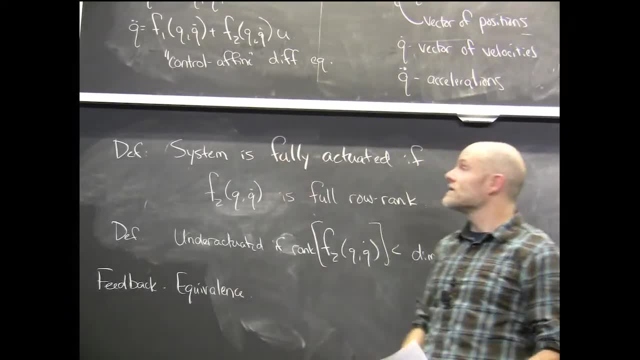 And the test for underactuated is even easier. So I won't do it on the board. 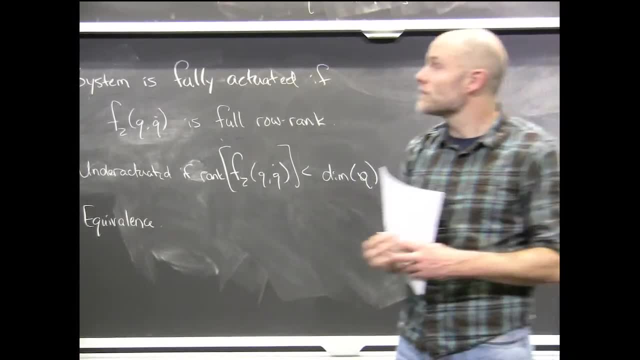 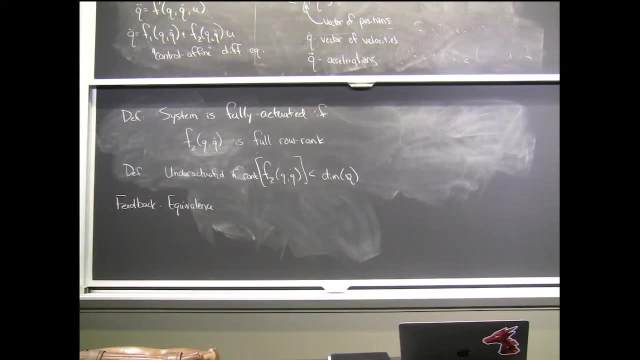 But let's just say I did it for this system. So this is my cartoon dynamics. We'll use these kind of little diagrams a bunch. So I'll try to be clear about it. Right? 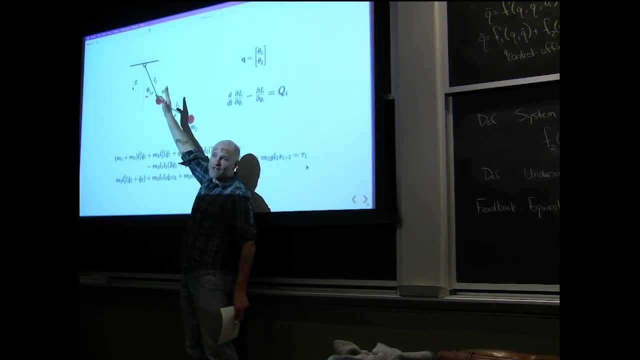 So I've got a pin joint attached to the world. That's what my little hatch marks means. 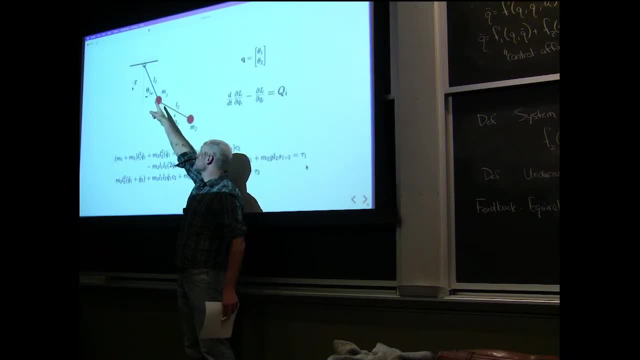 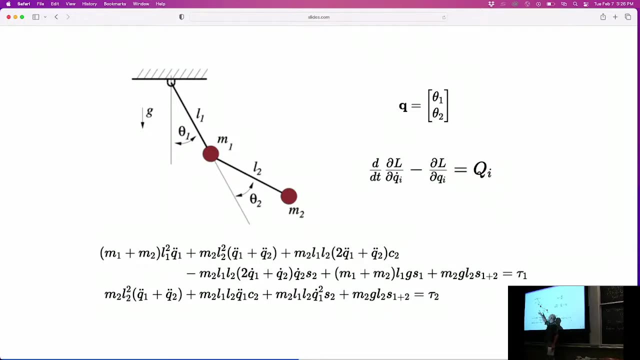 The world is bolted down up at the top here. OK, I've got a pin joint. I've got another pin joint here. The circles there are my indication that in the simple model, I'm going to concentrate all of the mass of the first link at that point. So that's a point mass assumption. It really doesn't. 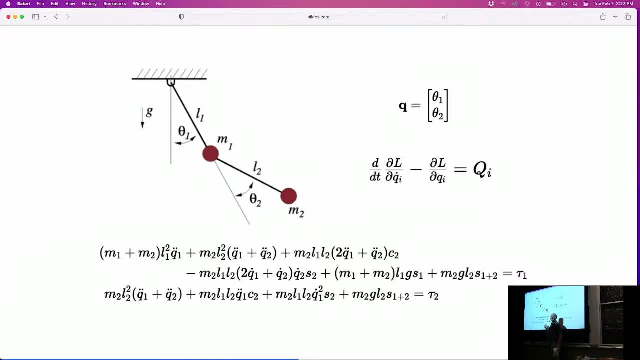 It's easy to generalize. But it makes the equations easier to write on the board. OK? 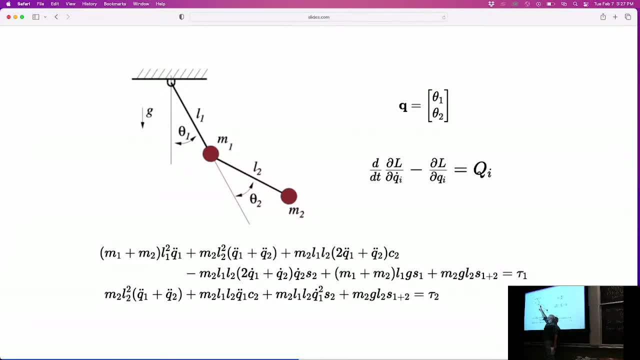 Similarly, I've got a second link here. So I just have parameters mass. The parameters of this mass, the length of the links, and then the q will be theta 1 and theta 2. 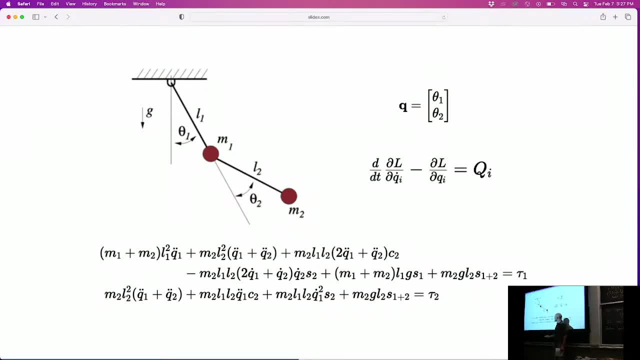 Those are the total positions. And then the positions plus velocities define the state. And I have the gravity. 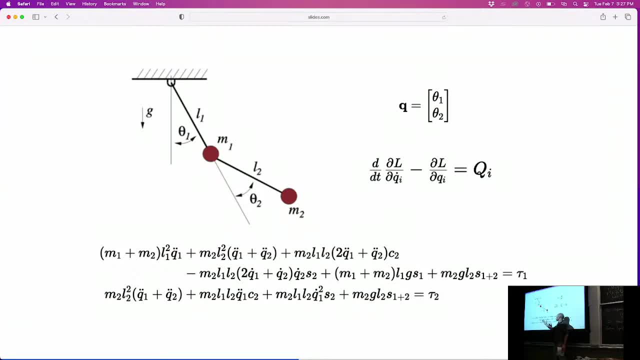 I don't want you to have to do it in the class. But I want you to know that it's easy to generate the equations of motion for these kind of things. It gets cumbersome if you get a lot of links. But it's not hard. There's nothing hard about it. There's a simple formula that you follow. You write the kinematics. 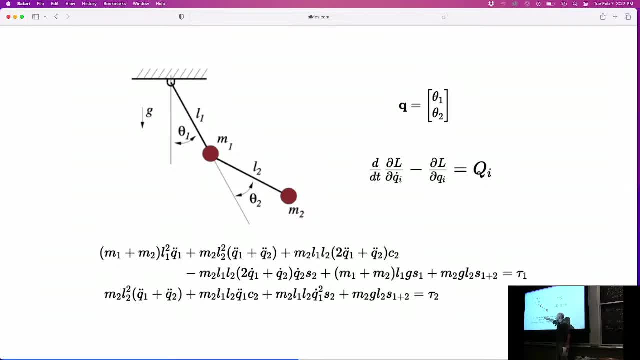 You take the derivatives. You put in the Lagrangian. And you get equations out that look like this. 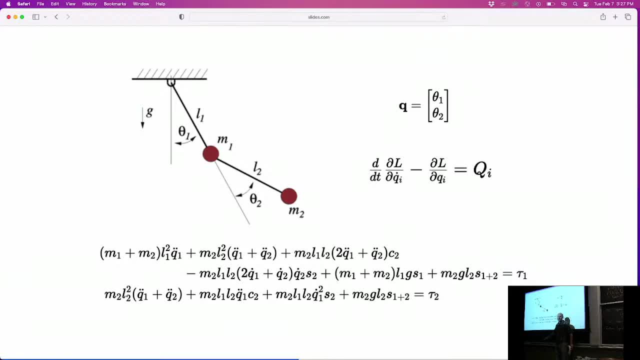 If you have five links, then they wouldn't fit on the page. They wouldn't even maybe fit on all the boards. It gets big fast. 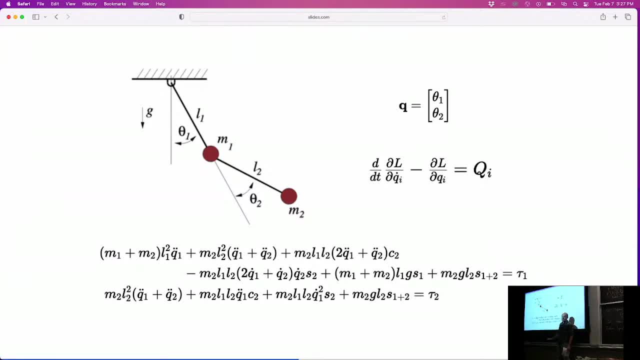 OK? But they all have this kind of structure. OK? 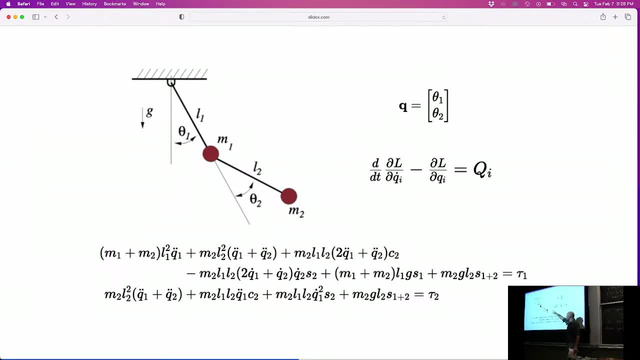 And in particular, so I called the control inputs here tau for torque. 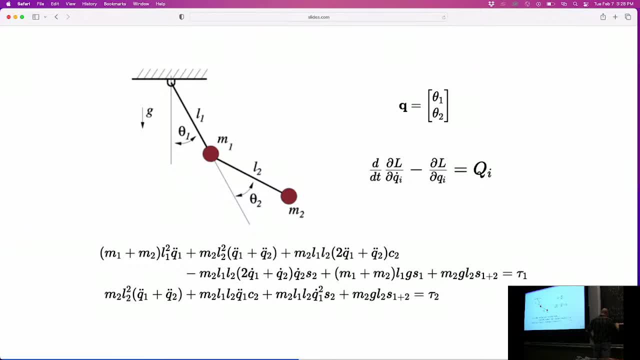 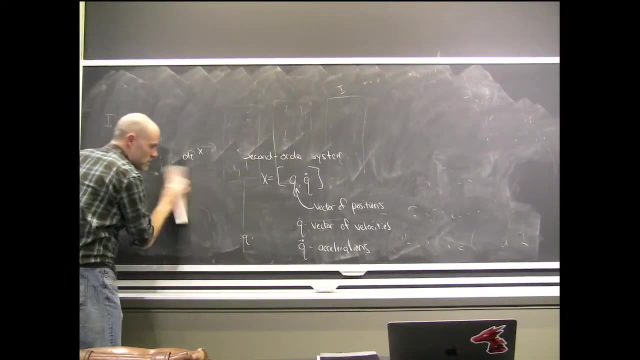 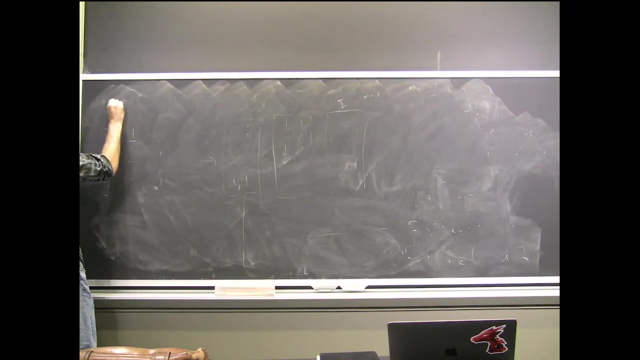 Just to be clear, in that picture, in that picture, I'm going to say the positions of that system are a vector theta 1, theta 2. Right? The state is q plus q dot. So it has four elements. The input here is torque 1 and torque 2. And I can write the equations. This is just a particular form of, well, I would have to solve the equations for q1 double dot and q2 double dot to get my equations that I just erased. OK? But I can solve for these. OK? 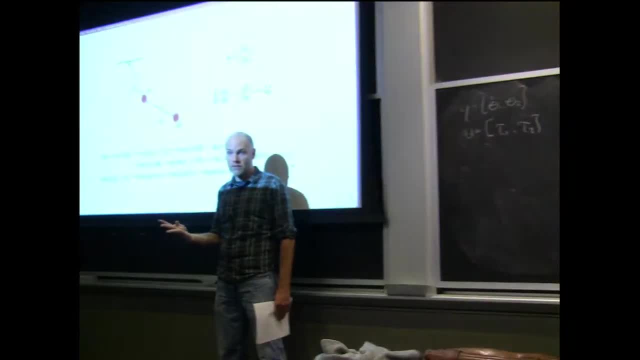 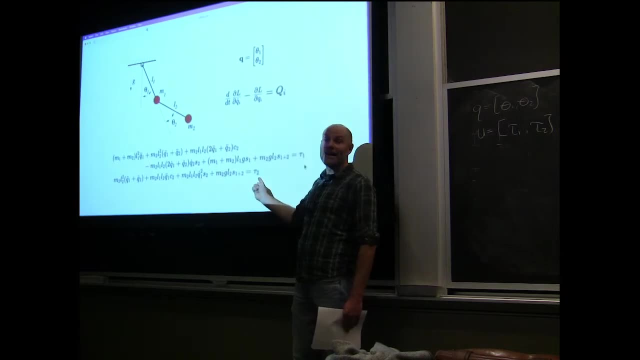 And get f1 and f2. And what's interesting is that when I do solve for these, you'll see that the torques come in in an affine way in this particular equation. But we'll see it actually happens generally. OK. 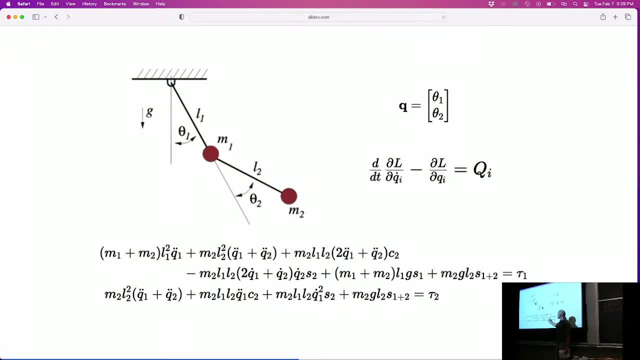 The way the mass comes in is in a very typical way. And there's actually a ton of structure in here. And we're going to, one of the goals for the class is to understand that structure as well as possible and how we can exploit it, if and when we can exploit it. 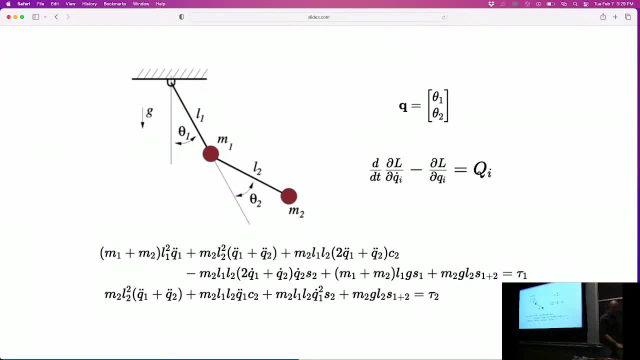 The nice thing is that you don't have to do that anymore. Right? 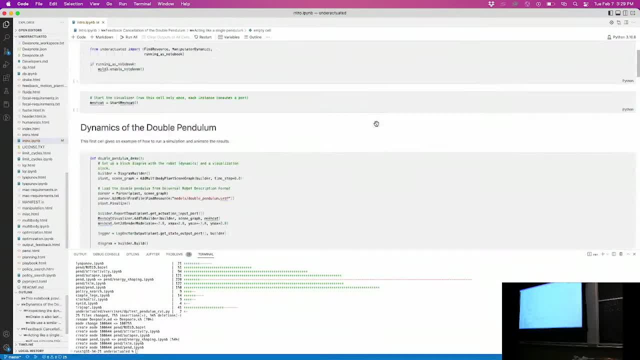 So you can just ask software to do it for you now. You can make this a lot bigger. OK. 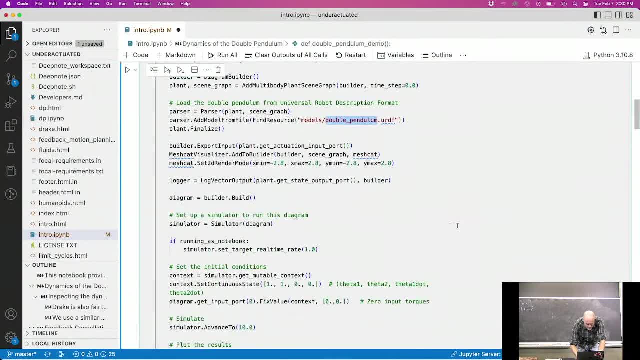 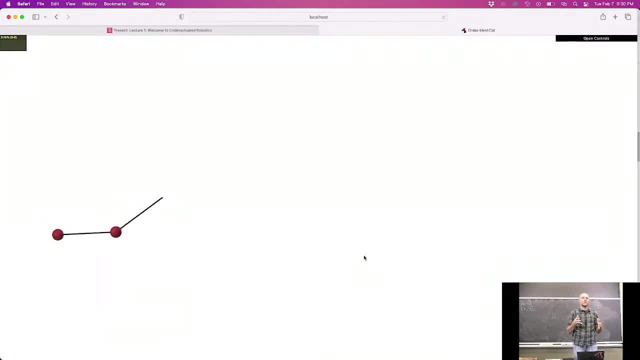 So I basically just said load. You can load a double pendulum and run a little simulation. And it'll generate the equations and run a little simulation. This is with torque equals 0. So I just dropped it. I also have little or no friction in that particular one. Right? It was just going along. 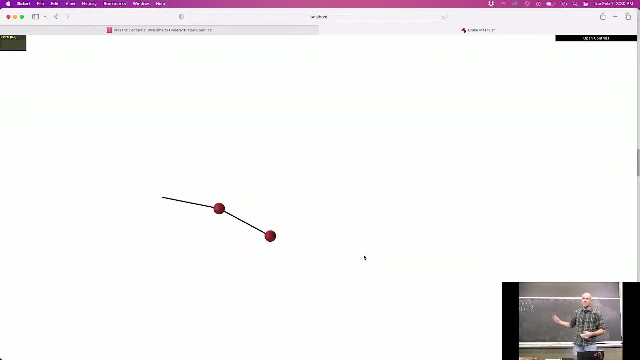 OK. And you don't have to write out the equations 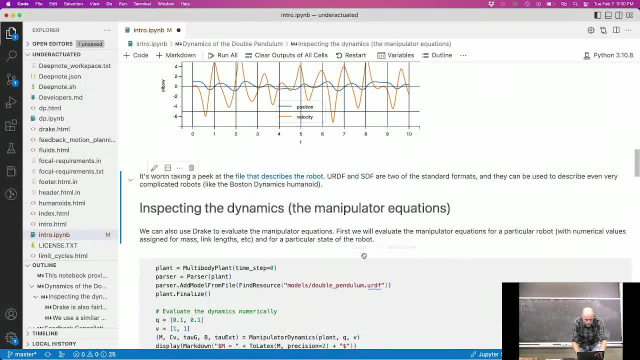 to get to that point. You can if you want, but you don't have to. And you can see the result there. 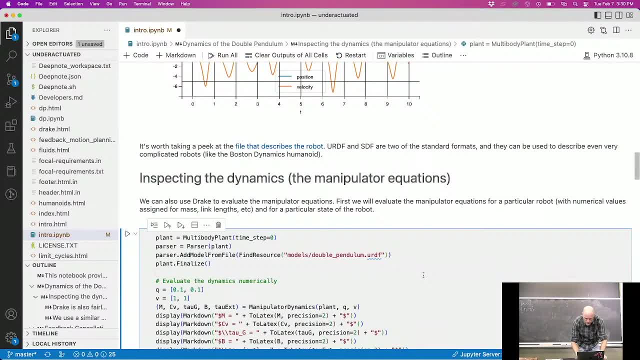 The software for the class, Drake, it tries to do more because I believe in the structure of those equations being super relevant. 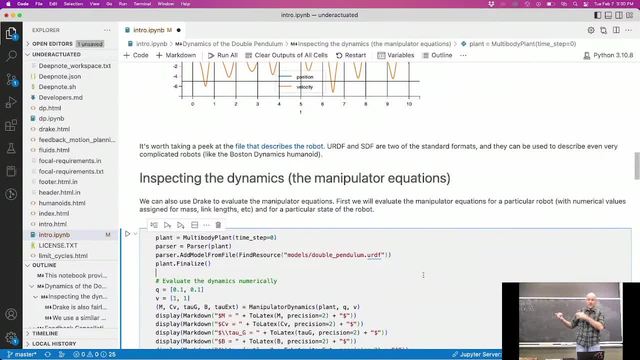 You can also, a lot of simulators will allow you to do that first thing, but they won't let you look inside the equations. And Drake really tries to, this particular software really tries to make it so you can inspect the equations and change the equations and write optimization against the equations. So. 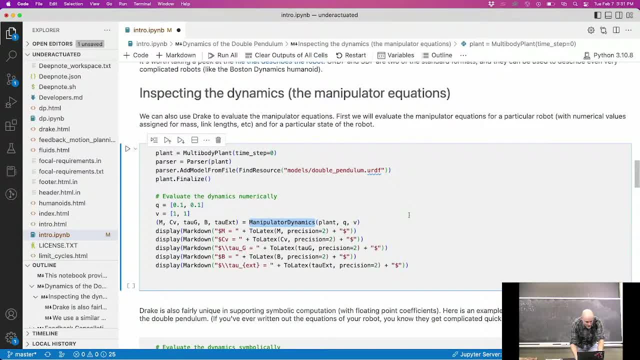 You can, for instance, ask for the manipulator dynamics, which we're going to write in a second. 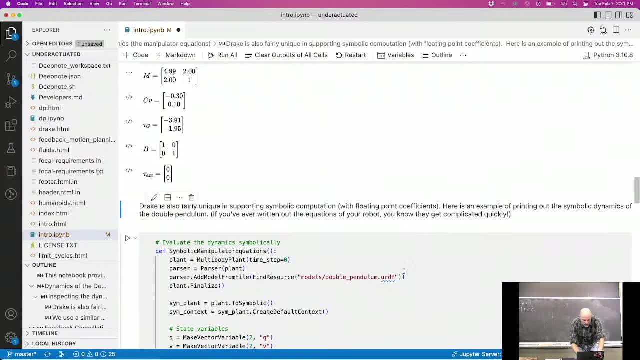 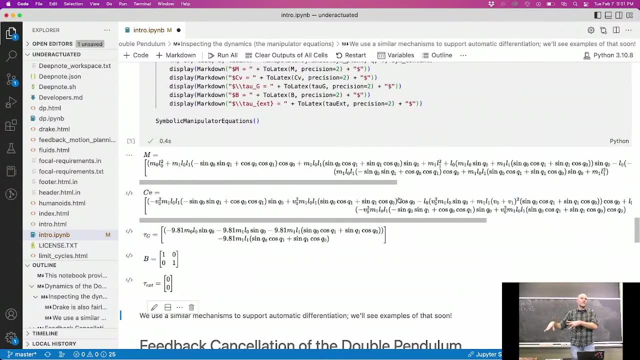 You can get the equations out at any state. And you can even get symbolic equations. The equations that I just wrote on the board can come directly out of the dynamics engine. So you give me equations of Atlas and say, I want to see the symbolic version of that. Not just run a simulation, I get the symbolic version of that. And that's possible here. Although if you ask it to print, it's going to take a long time. OK. 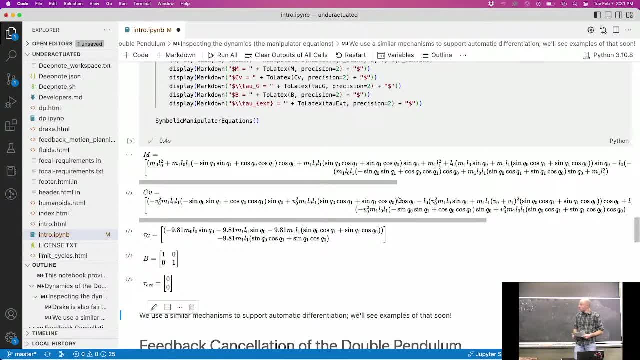 Because that Atlas would be ridiculous. But that's a super useful thing. But the thing that you do if you do this over and over again is that you realize that the equations of all of our manipulators have even more structure. And that structure is what I used in the code. I forgot I used it in the code. It's called the manipulator equations. 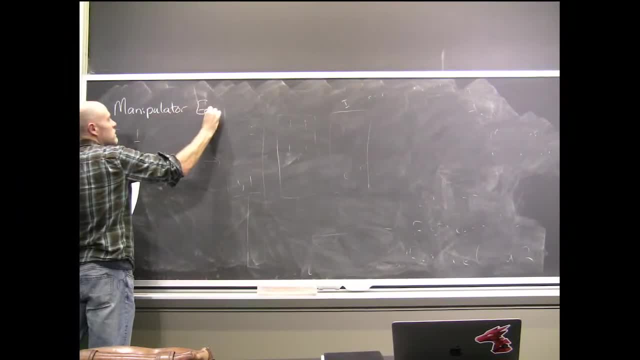 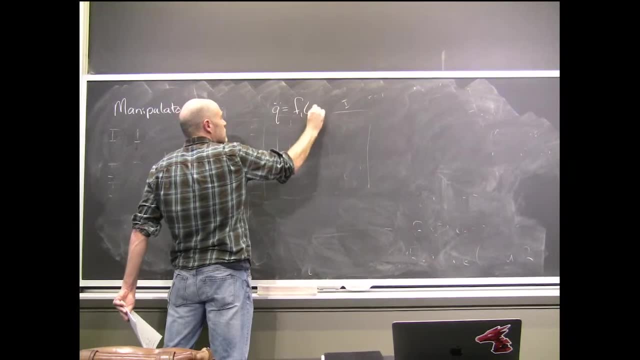 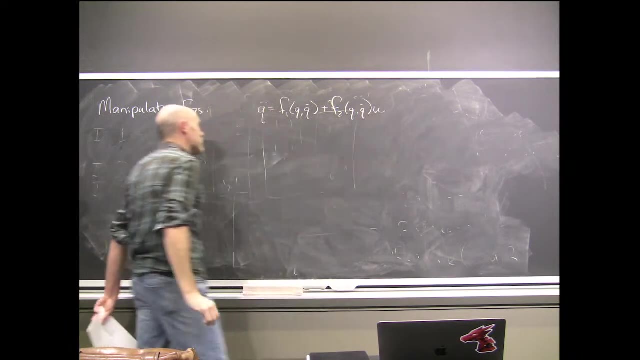 So every time I go and evaluate this second order dynamics for my robot, it turns out I could write it even more structured like this. 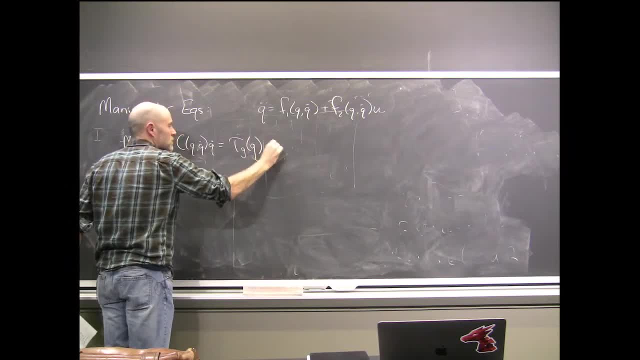 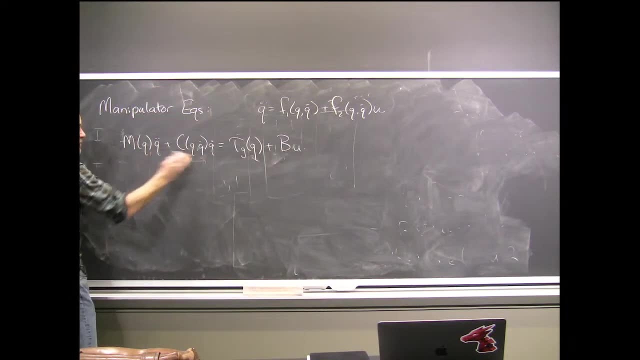 So this is the second order equation. If I just take mass matrix inverse, I can get it into this form. So let me just say that this thing is called the mass matrix or the inertial matrix. It happens we know a lot about the mass matrix. 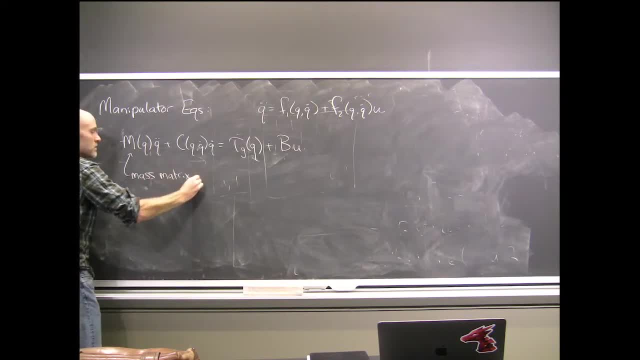 It's positive. And it's ultimately going to be positive. 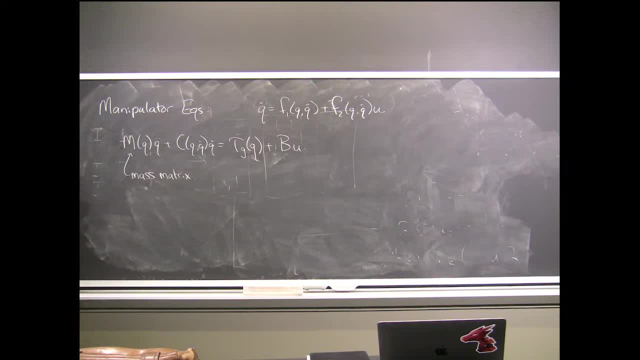 So this thing is called the mass matrix. And it's going to be positive if you do this. 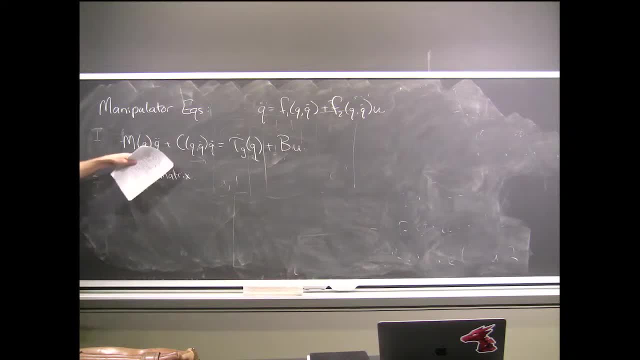 We need to know. And it's always invertible. It's uniformly positive. It means for all q, it's going to be positive. 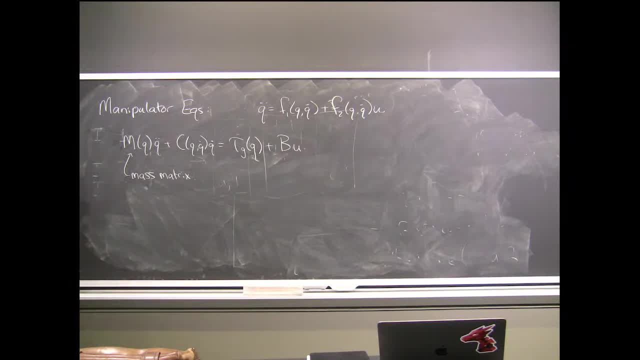 Mass tends to not be negative, which is good. 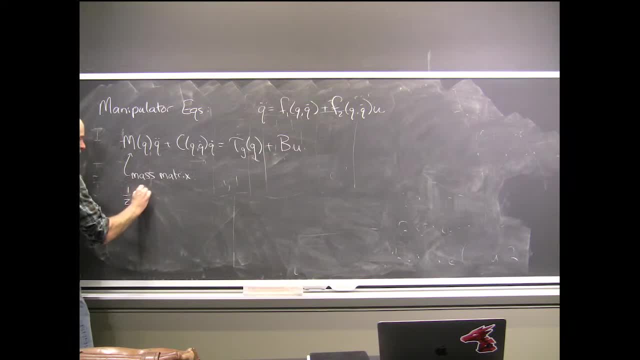 Kinetic energy is actually just 1 half q dot mq q dot is kinetic energy, for instance. 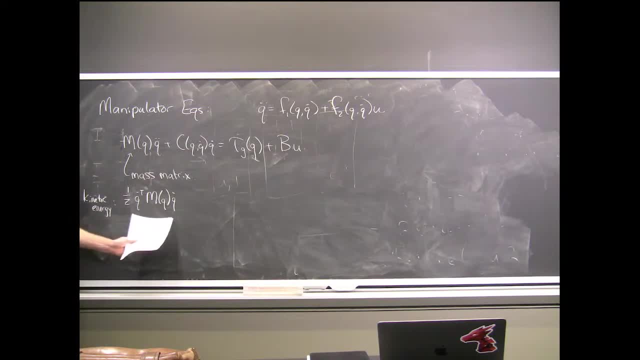 We know a lot about it. And just by saying that, m must be positive definite, because kinetic energy is positive. This thing is called the Coriolis matrix. 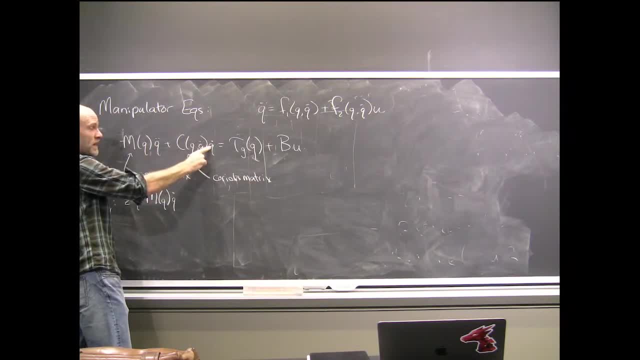 And it always has dependence on q dot, which is useful to know. If your velocity is 0, that term completely drops out. 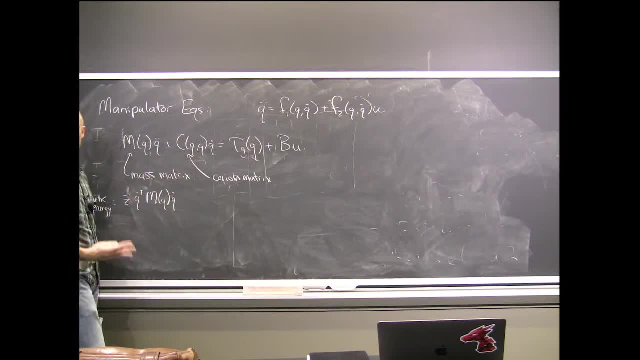 Calling out that structure just makes me instantly see that if I'm in a 0 velocity state, that's not contributing anything. 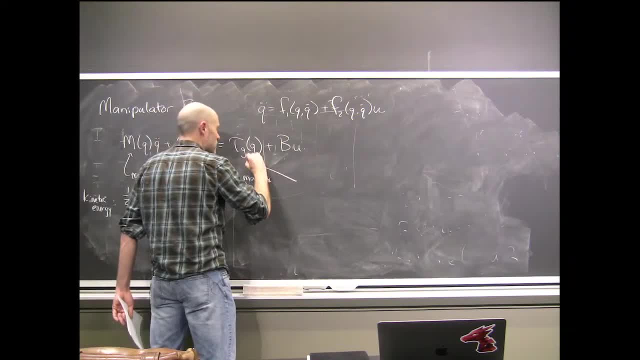 It has more structure, too. But this is a gravity vector. 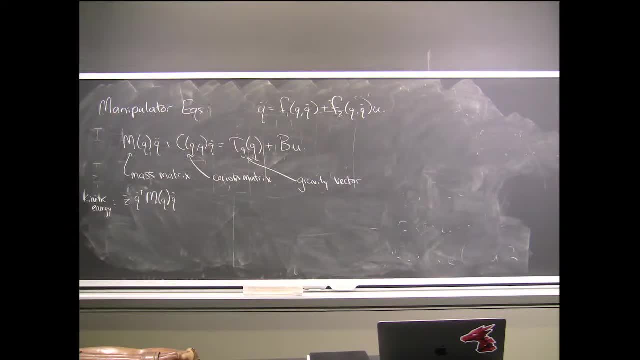 More generally, we could have springs or other potential terms that hide in there. 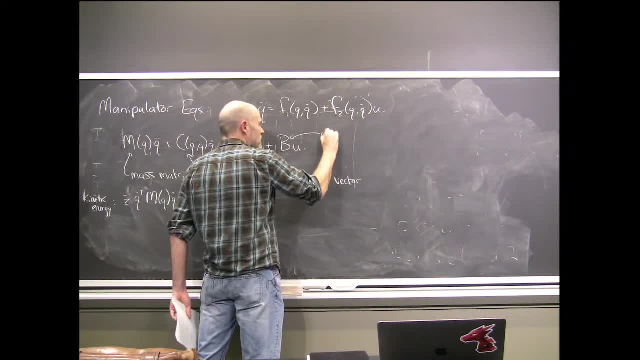 We know this is my control input. And this one we call the actuation matrix. 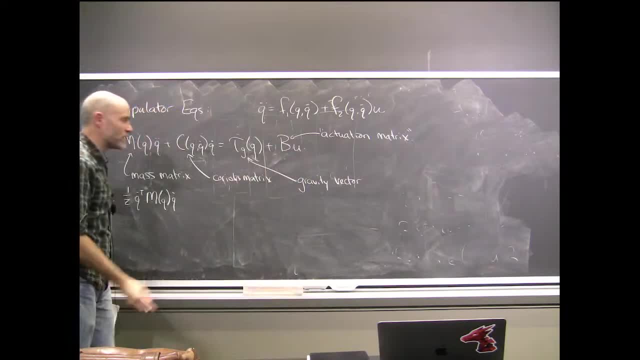 It maps my control input into the third. OK. So this is the q space. OK. 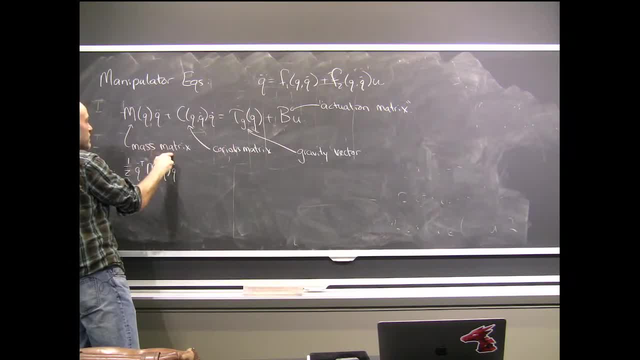 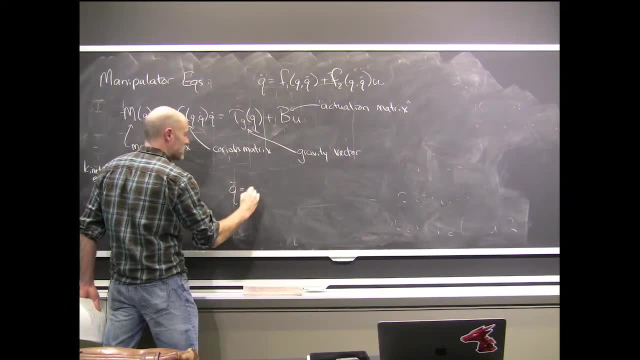 So if I want to get this form out, then because I know mass matrix is positive definite, then I can always invert this. So I can say the q double dot is the mass matrix inverse times the rest of that. 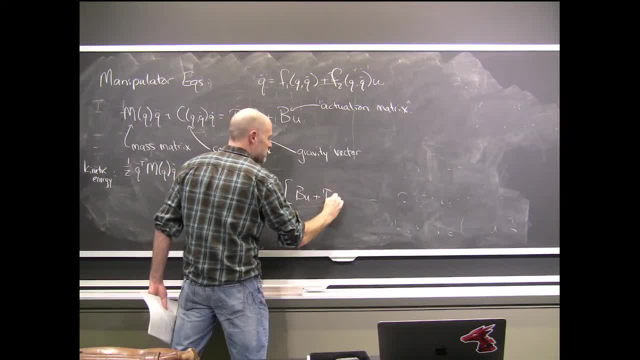 You know, eu plus tau g q minus c. 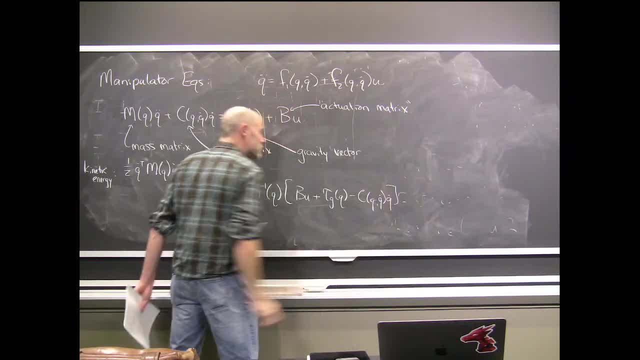 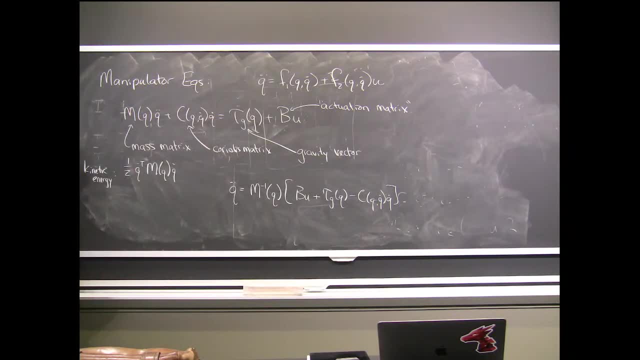 I can take, for example, this product and put this into the formula. And that puts it back in this form. And that puts it back in this form. This is always positive definite. 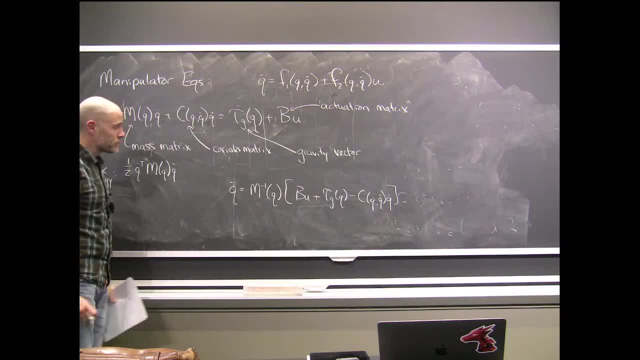 So it turns out, remember, the condition we cared about for under-actuation was whether the rank of F2. Whether F2 was full row rank. 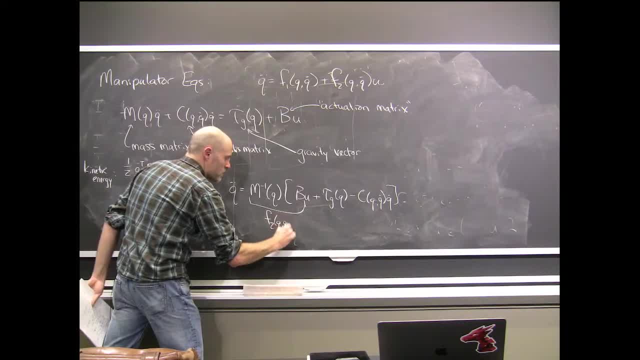 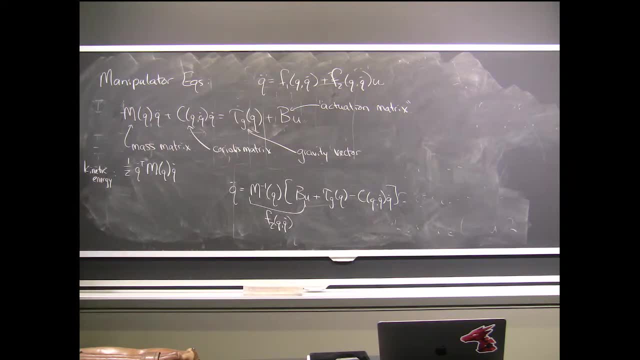 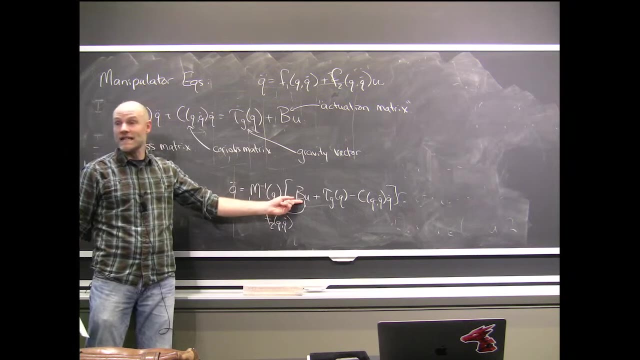 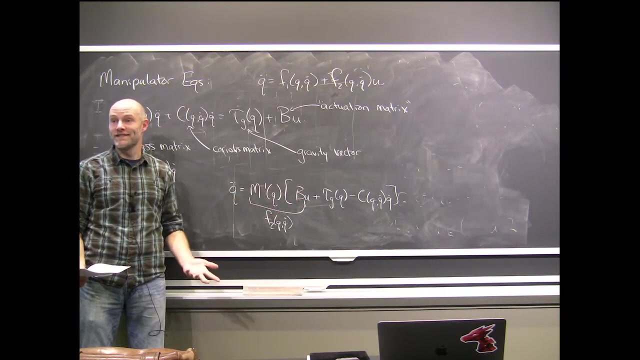 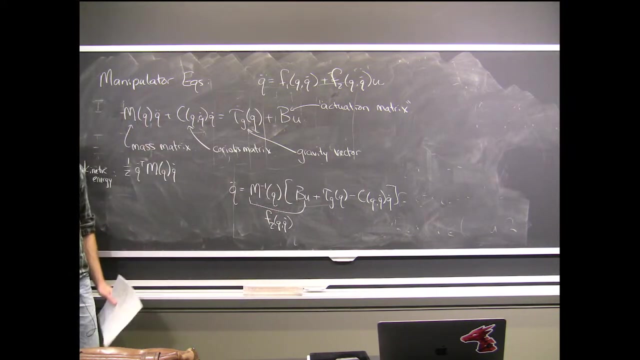 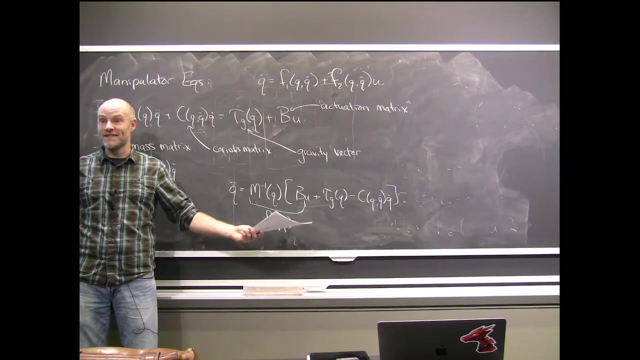 is right here so in the manipulator equations the test is even easier you can just ask since this we know is going to be full rank you can just ask if B is full row rank if your actuation matrix is full row rank then you could you are feedback equivalent to Q double dot equals U so what's a what are ways to get that now we can have start thinking about thinking about this more mechanically right so if I have an actuator on every single joint I have a robot arm attached to a table and I have a motor at every joint then B could be even the identity matrix and that system is fully actuated that's the canonical fully actuated system okay if I'm a humanoid I am a humanoid if I'm a humanoid and I'm doing a backflip I have Q variables that 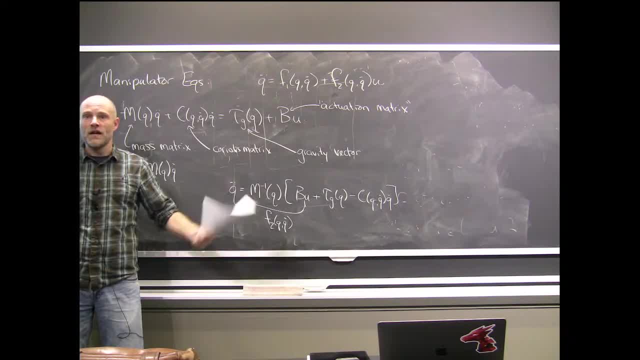 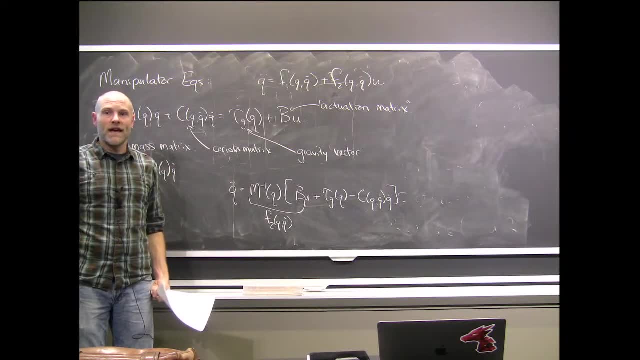 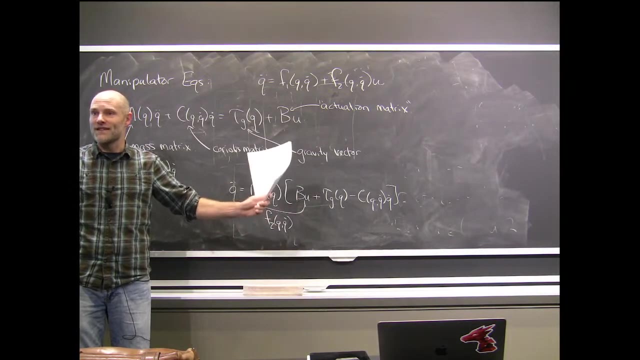 represent my joints which do have actuators but I also have Q variables that represent the position of my center of mass and the orientation of my center of mass and when I'm in the air right nothing I can do with my assuming there's no air resistance or whatever nothing you know if I'm in space doing backflip that's the canonical fully actuated system okay if I'm a humanoid 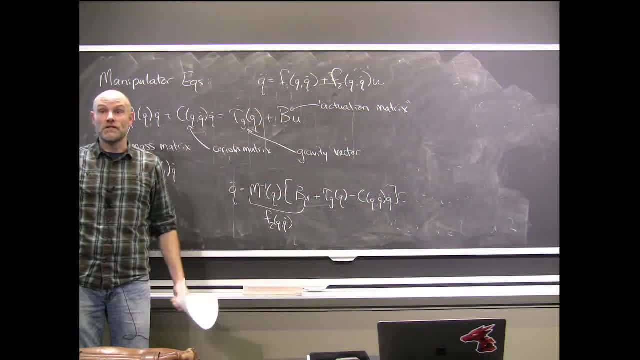 if I'm in space doing backflips right then nothing I can do is going to change the ballistic trajectory of my center of mass okay the way that manifests is 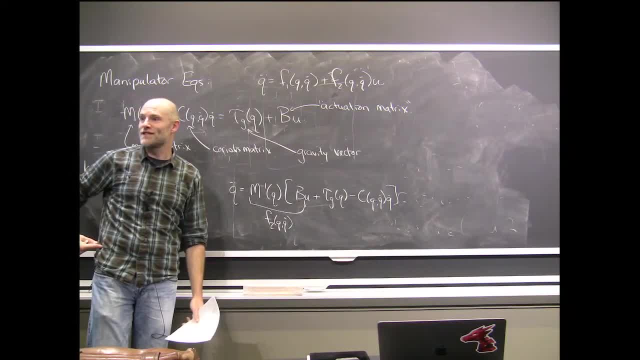 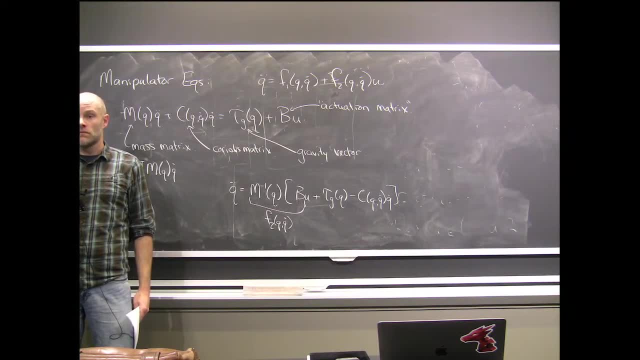 because there's some some cues which represent the position of my center of mass and I become low rank I cannot instantaneously affect those equations 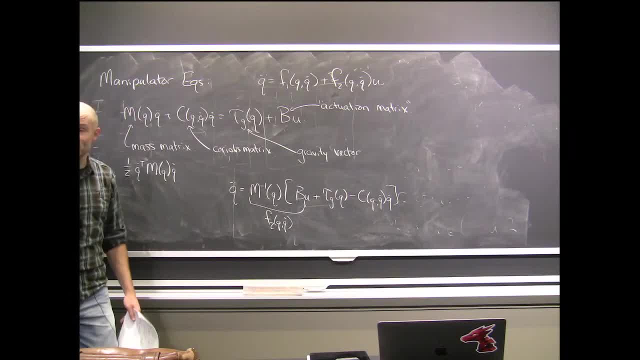 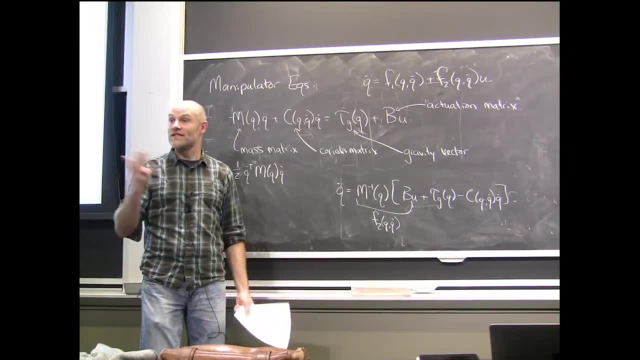 now there's all sorts of subtlety that happens right so if I'm standing on the ground right at what point am I bolted to the ground like am i tipping from the ground and there's a there's an interesting there's places where legged robots look like they're fully actuated as long as 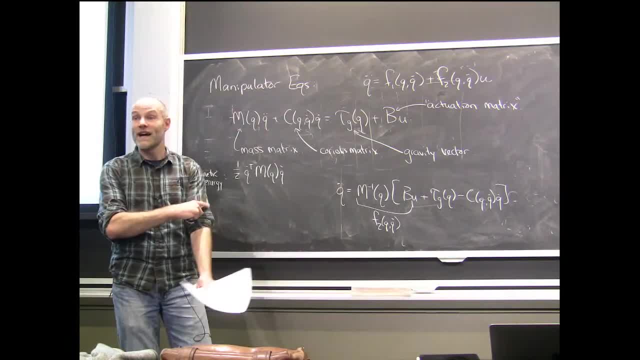 your foot doesn't tip from the ground and we got surprisingly far in the world of walking robots thinking like that and that's why a lot of robots the older 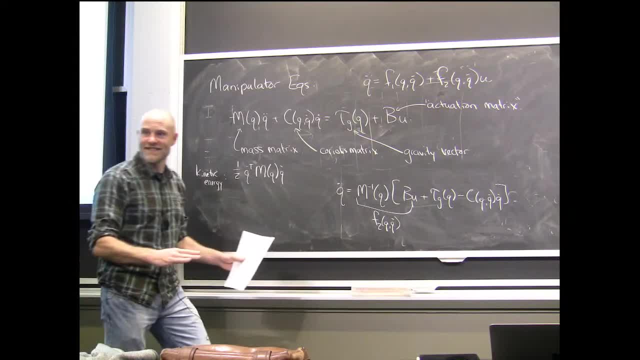 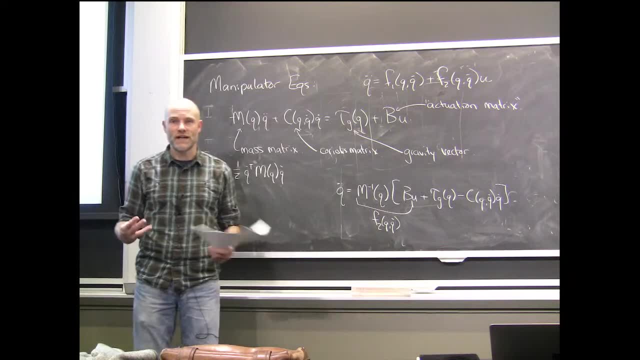 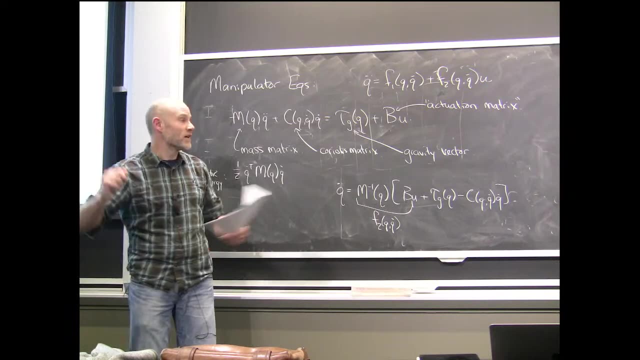 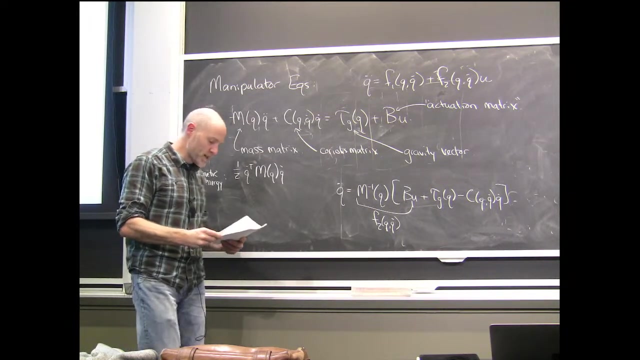 robots you might have seen kept their foot and I did nice and flat on the ground right all right did the kind of classical walk in that regime then we can act like a fully actuated system and we have control is more easy and more easy you tell me a trajectory you want me to follow I can tell you f2 inverse to follow that trajectory okay but once you take that away it's it's harder yes 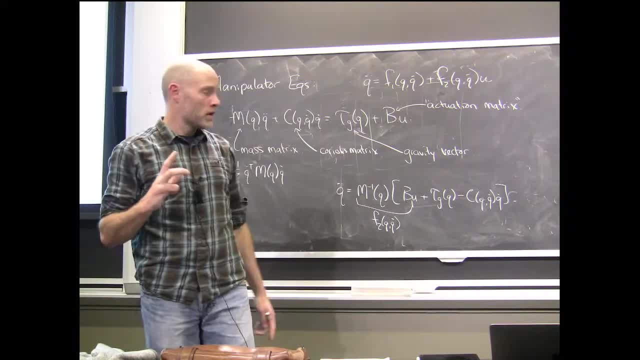 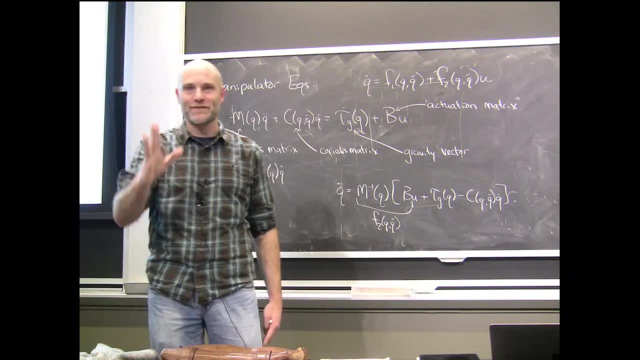 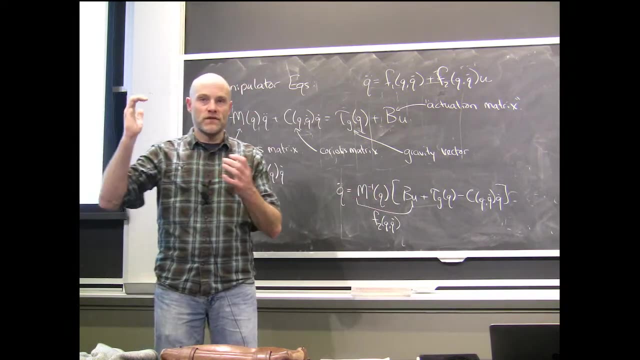 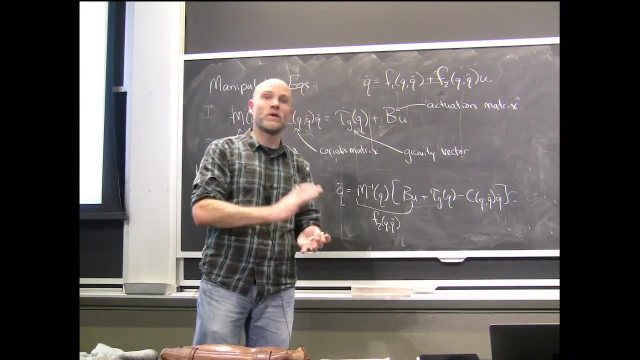 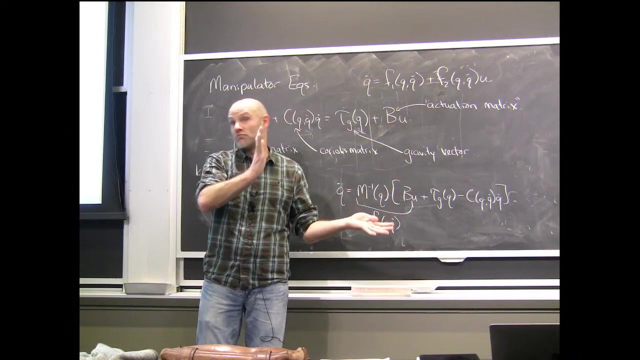 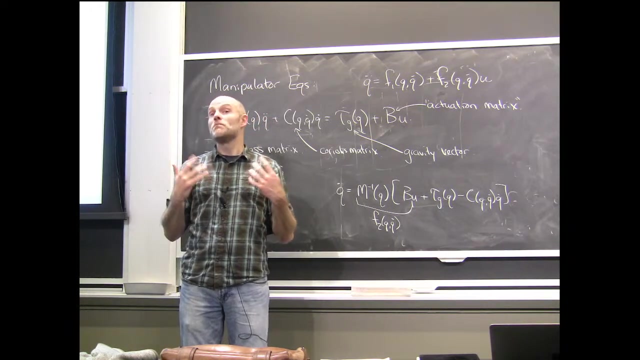 good so the question was about hybrid systems so hybrid is hopelessly overloaded term just because we're going to use it heavily in a different way let me just clarify we're gonna often think about hybrid as being both continuous dynamics and discrete dynamics for instance a robot that is you know governed by F equals ma Q double dot and every once in a while has discrete collisions with the ground we will model that as a hybrid dynamical system you're talking about hybrid in a different way maybe where you have some parts of the robot that are fully actuated for instance and another part that's under actuated so we'll have partial answers to that there's there's things called partial feedback linearization for instance or 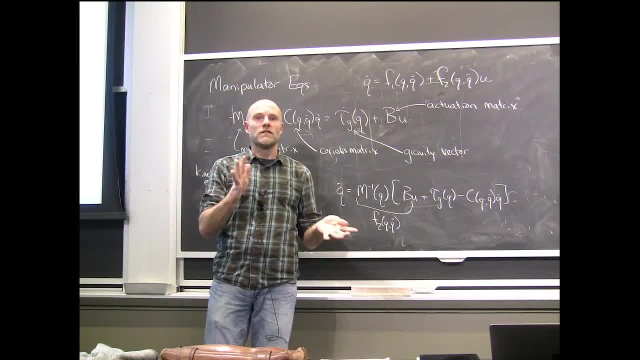 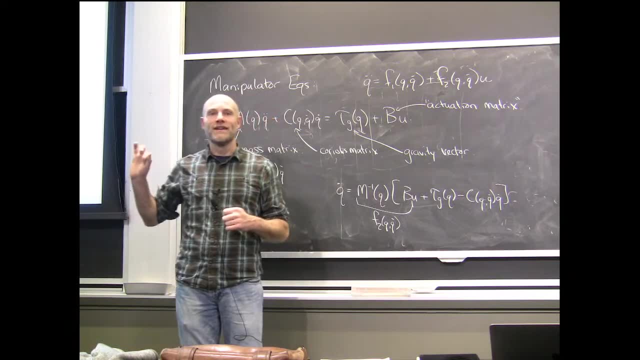 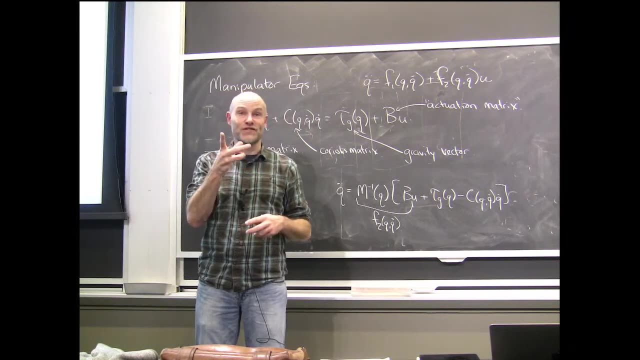 partial feedback equivalents where you can make part of your system and even sometimes it can be surprising how far you can go with that rough rule of thumb is if you have n states M actuators assuming coupling you'll get to control M of those states roughly but it gets it well we'll see you in the next class 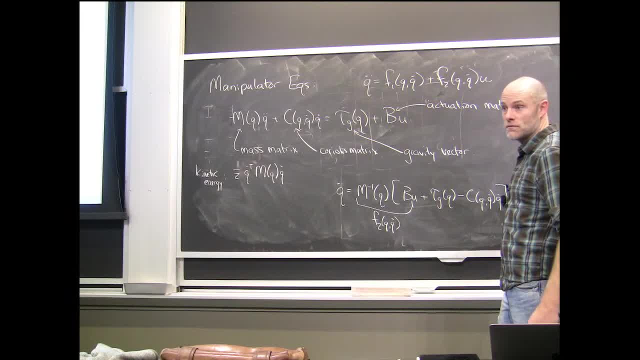 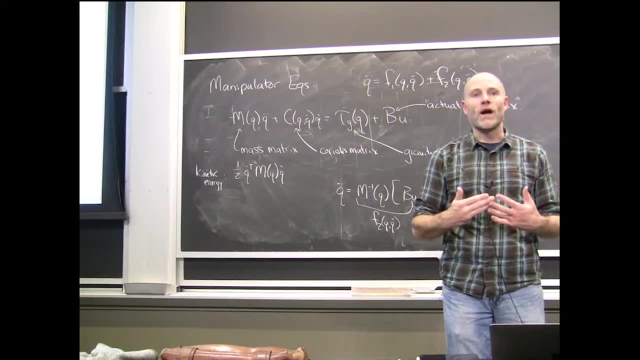 we'll see the details soon and write in a new set of equations so to just make that point right so if I did feedback cancellation of a double pendulum and I want it to act like it's a single pendulum okay then I can write a very 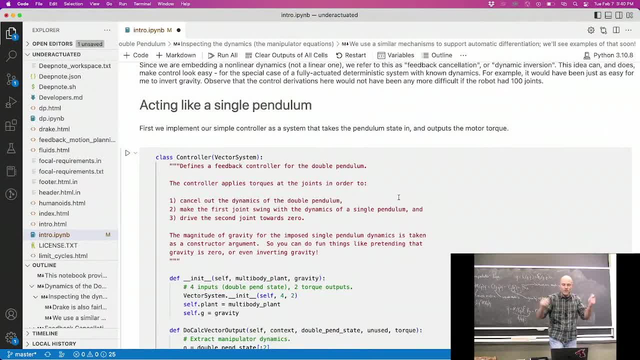 simple controller that just erases the one dynamics puts in the new dynamics 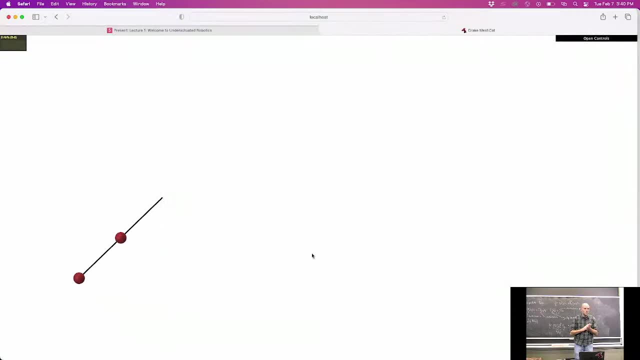 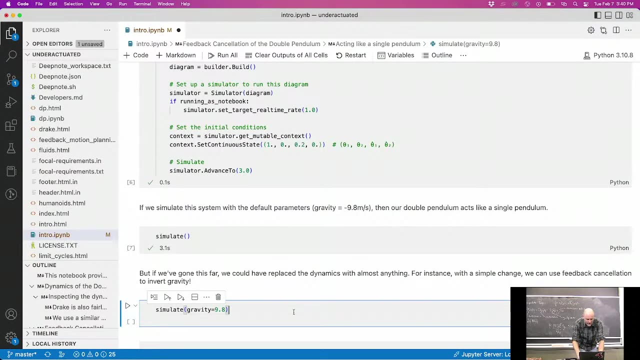 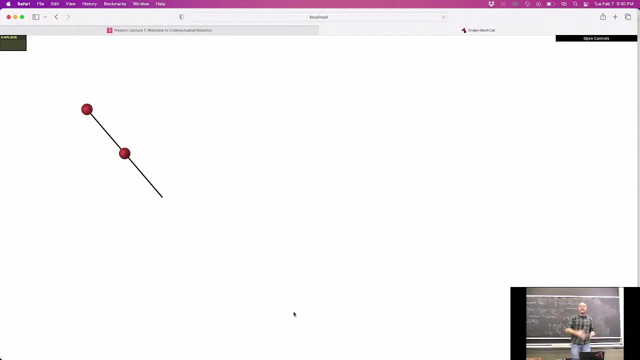 and acts like a single pendulum okay that one's not very surprising but it's also you know you can start thinking about it why it's kind of ridiculous because I can also just say I want it to be a single pendulum that's upside down I could just reverse gravity right there's really no reason why I couldn't replace it with the dynamics of a single pendulum so if my goal is to make the thing swing to the top just pick a dynamical system that ends up going to the top and you can just erase the original dynamics 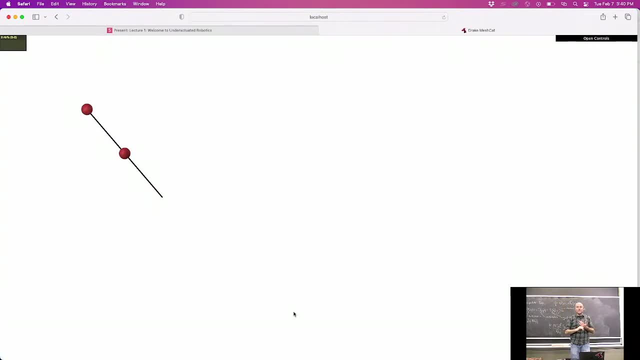 that put it in now that's not very efficient if you run into input limits 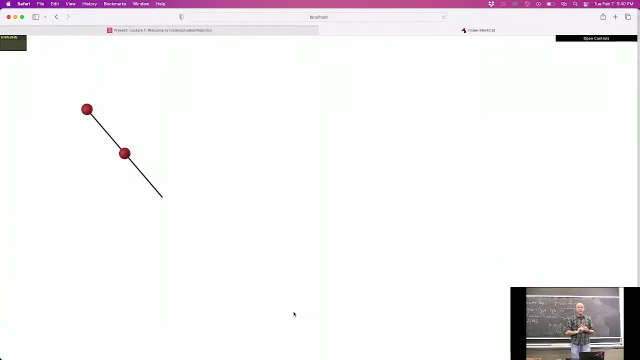 or whatever then it can be a losing strategy but it gets you pretty far and a lot of you'd be surprised how far we got in robotics without with with taking 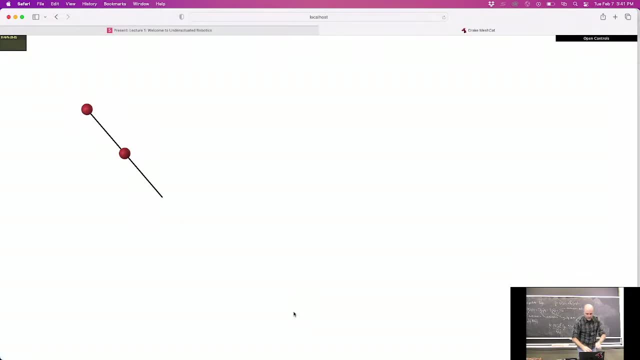 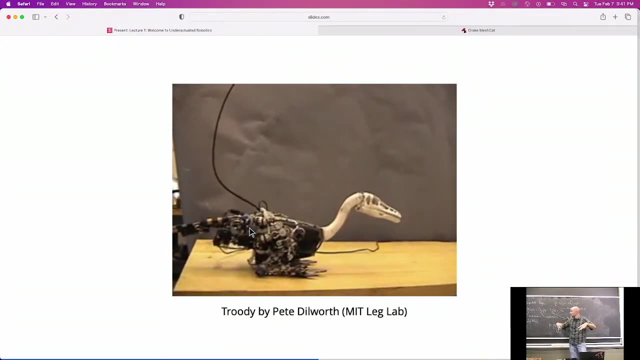 that approach locally so maybe even to make that point again here so when I got to MIT a while ago there was a MIT leg lab that was Mark Ray Burt's lab 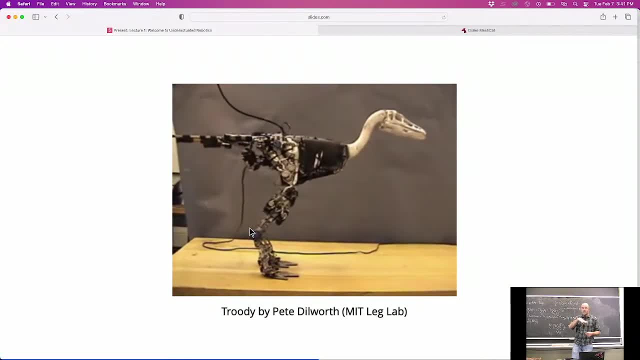 initially at CMU he moved it to to MIT and he had then left to start Boston Dynamics Gil Pratt ran the leg lab at MIT when I came by and there was a guy Pete Dilworth who was hanging out in the 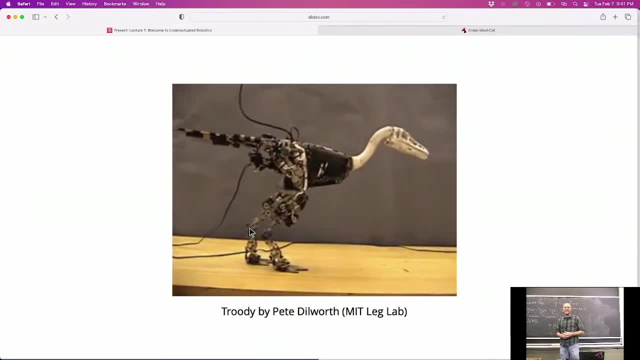 basement making dinosaur robots and I just fell in love completely I was like this is what I want to do with my life okay now this was a there's actually a ridiculous soundtrack with this too but which I see it and I start thinking 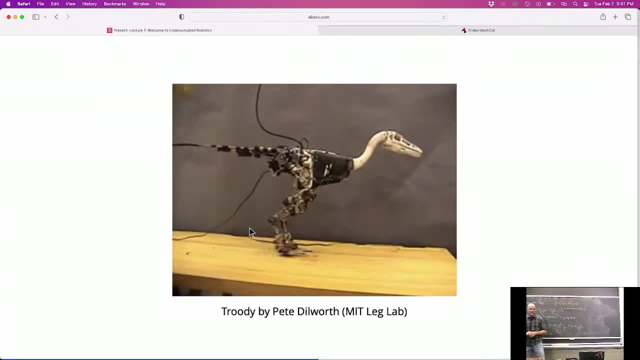 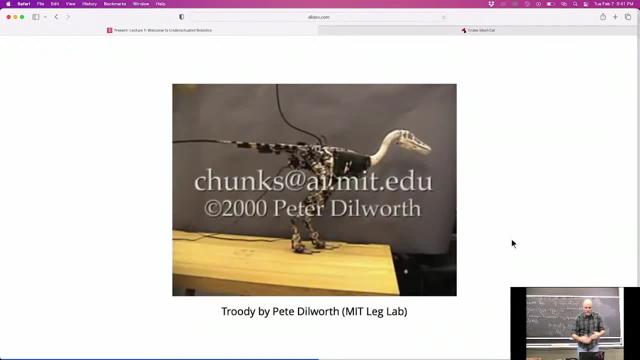 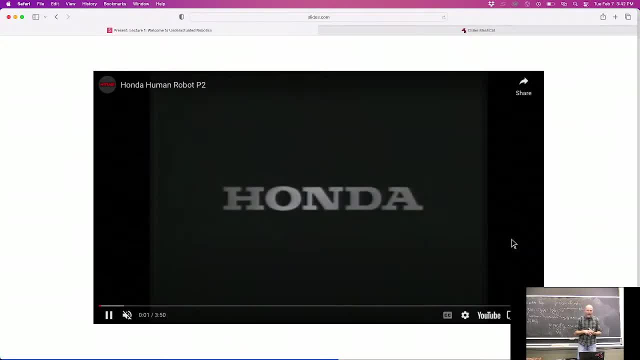 you know and then I was also in the leg lab the day that Honda stopped by for a presentation and sort of told us a by the way we've been secretly working on walking robots for the last 20 years right and everybody's like what you know that you have a complete humanoid that can walk around and it's insane 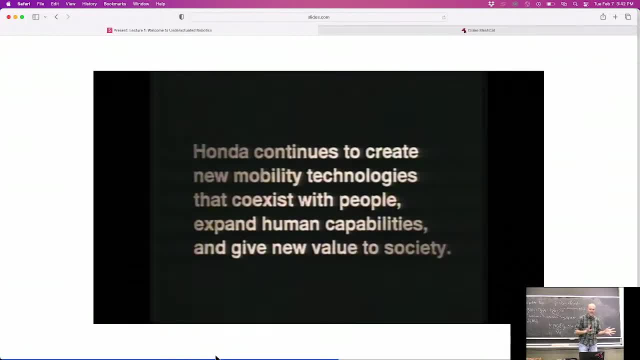 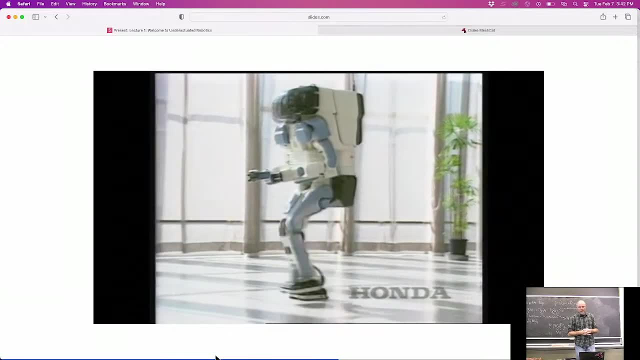 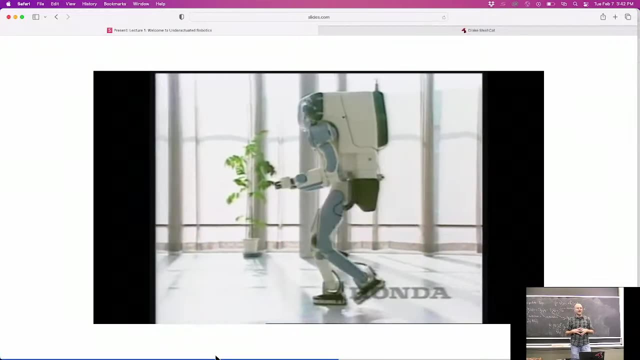 So this was, P2 is this first video, which came out around 97. I was actually not there when it first came out, but I was there for the next version of it, okay? And this was like, you know, oh my gosh, you know, Honda's solved all the problems kind of moment when we were sitting in the leg lab, right? 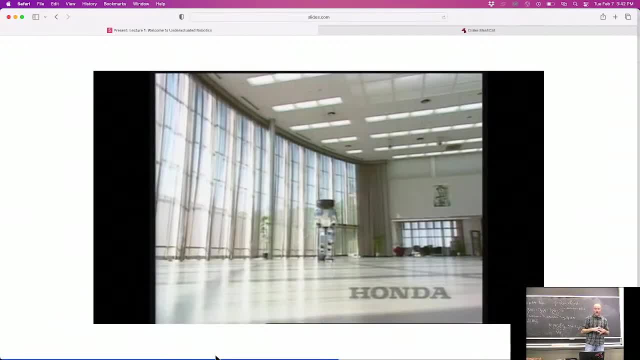 It has that canonical flat foot walking. 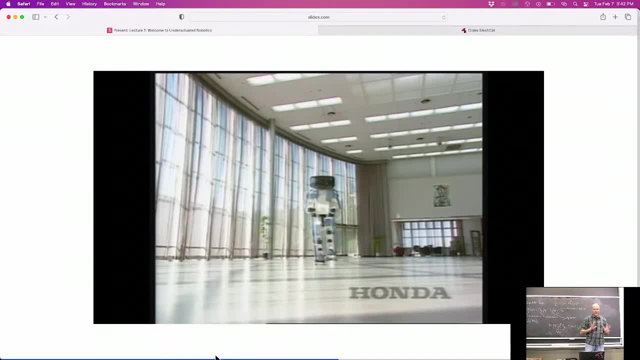 It's actually a dynamic, some people will say it's statically stable. That is not true. We'll get into that. 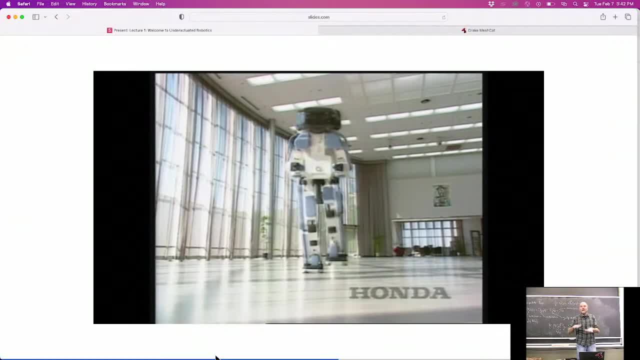 It's actually a beautiful control solution, but it is based on the extensions of sort of robotic arm kind of thinking, fully actuated robotic kind of thinking. 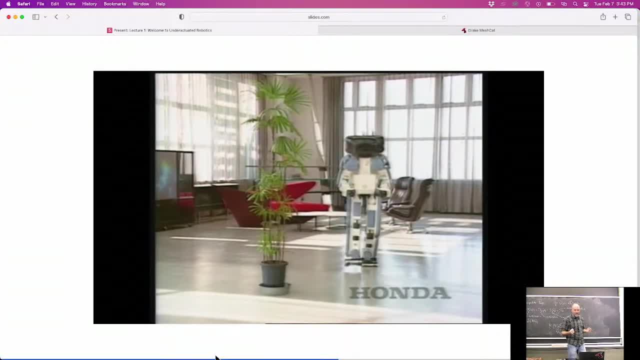 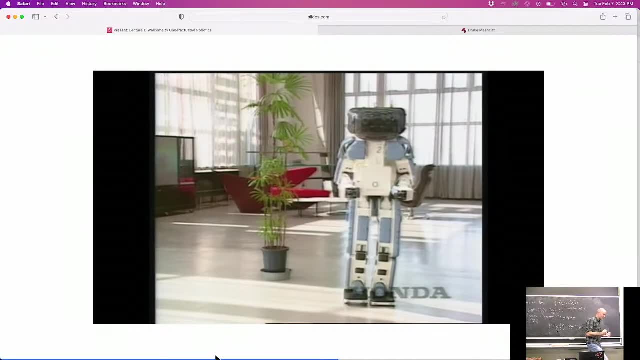 And the way you can see that is that it doesn't look very natural, right? So the actuators are doing a lot of work to effectively cancel out the dynamics of the leg, right? When you walk, your leg wants to swing forward, okay? 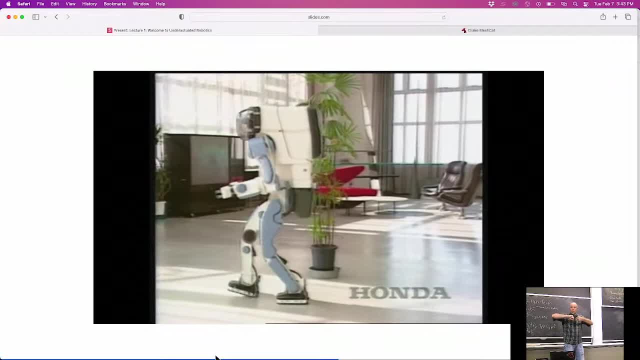 But this is, in order to, to keep things in control, we're doing a lot of work with the control system in order to erase the dynamics of the robot. 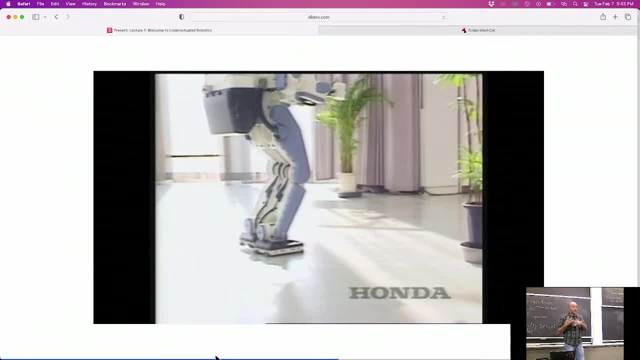 In fact, even the actuators erased some of the dynamics that you would think of of the two-link robot, okay, leg. 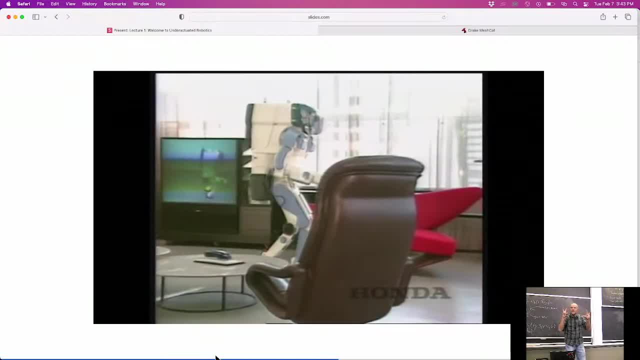 And then we're replacing it with this stiffer, but completely uncontrolled version, okay? 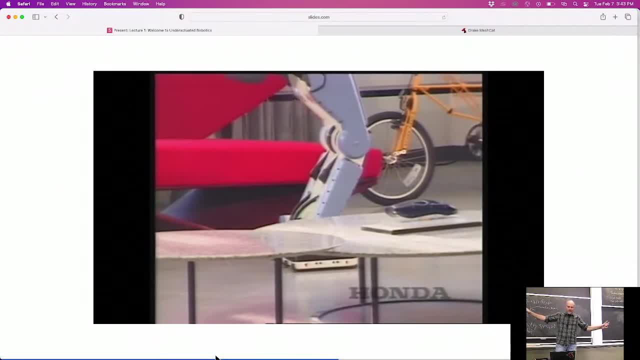 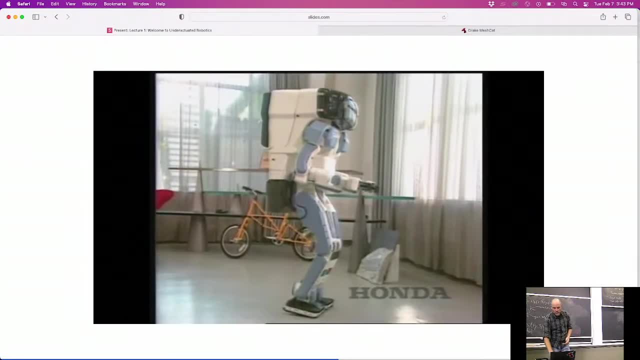 And it was amazing, absolutely amazing, changed the world stuff. But it also made us start thinking about, how that's not necessarily the only way to do walking. 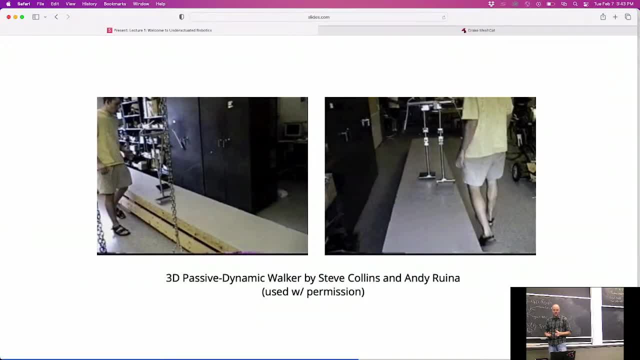 And the extreme version, my favorite version to this day, this is also a walking robot, but it has no motors, no controllers. 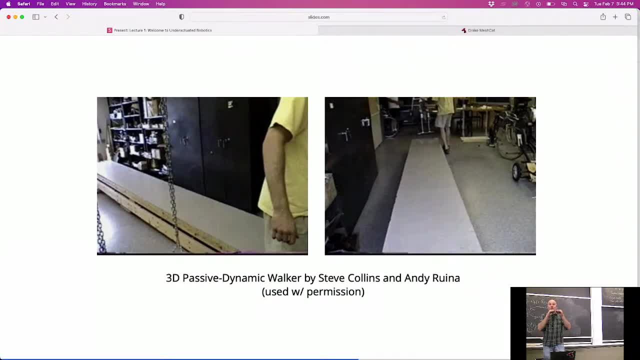 It's basically an elaborate slinky that you put on top of a small ramp. If you have no ramp, it doesn't work. It's powered by gravity. 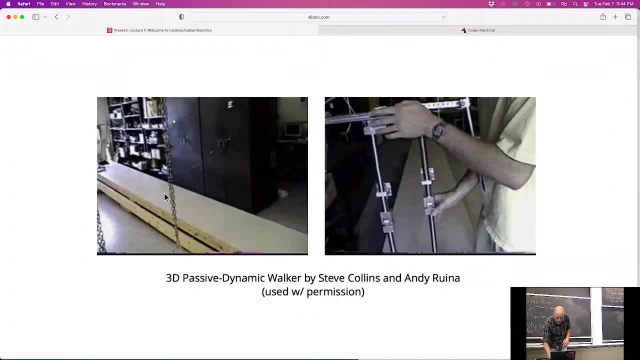 You put it on top of a small ramp. Let me see if I can get it to play again. 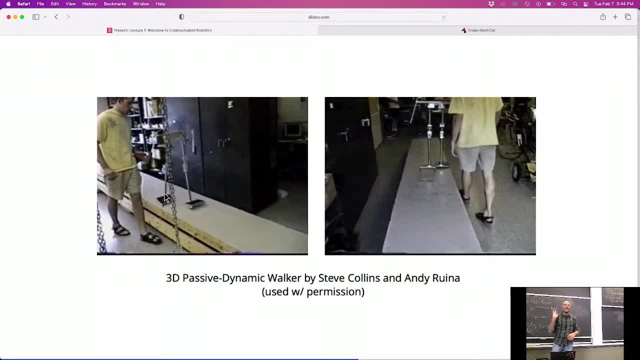 Okay. You give it a little push. And my gosh, that's a beautiful gait. That looks like a human walking through the park, right? This is called passive dynamic walking. 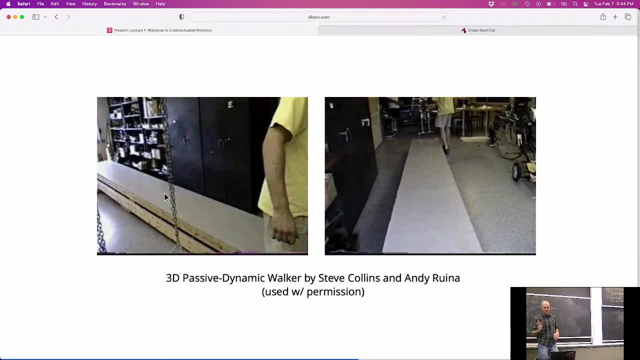 This is one of the best ever built by Steve Collins, who's at Stanford now, and Andy Ruina at Cornell. 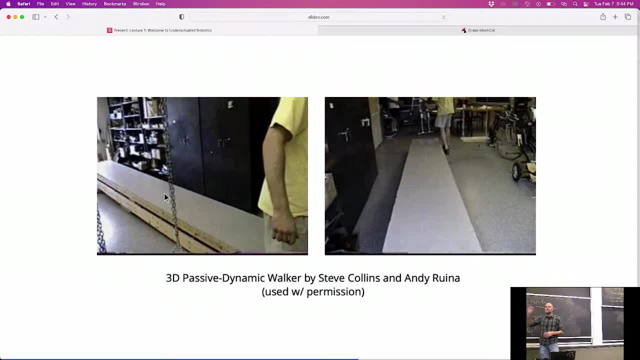 Okay, and this was the exemplar of a different approach, which could use zero energy on the ramp, little energy on the flat, right? 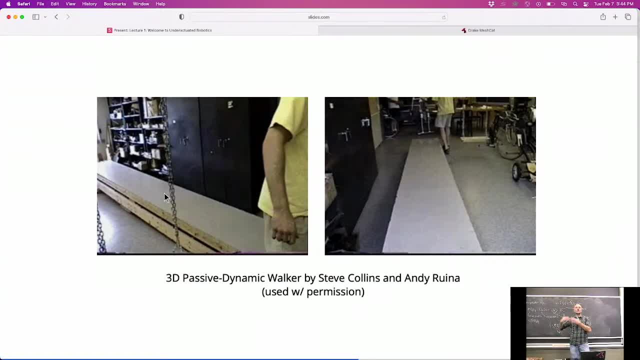 You have to solve a harder control problem. You have to think longer. You have to think longer. You have to think longer. You have to think about the long-term consequences of your actions, but the result can be beautiful. 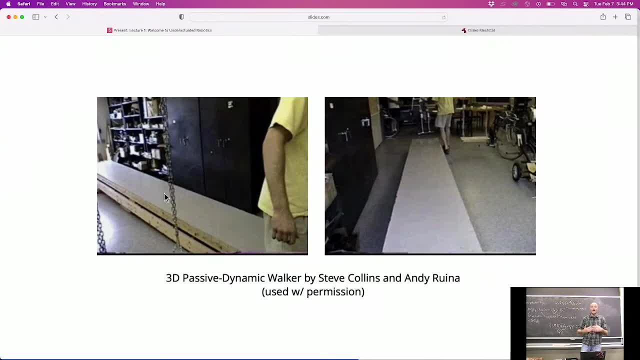 So that's how I came into all this, was being inspired by this and wanting to think about how do we build controllers that use push and pull on the natural dynamics in order to make things happen. Okay. It was actually super fun. 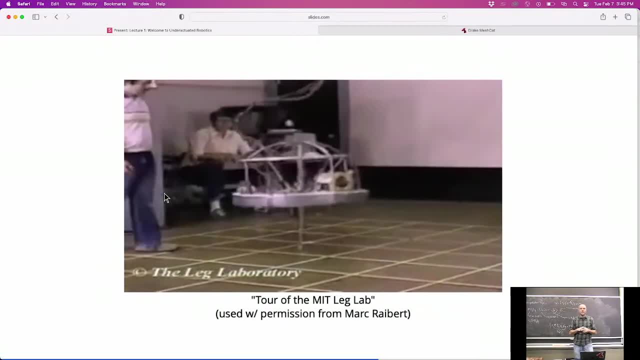 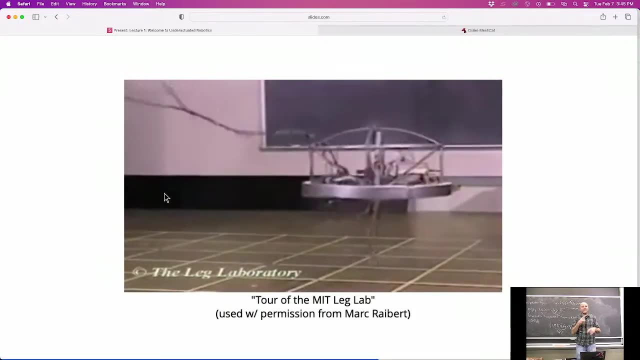 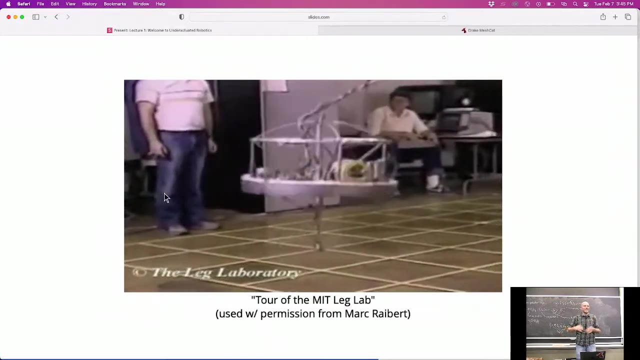 So Mark Raybert, when he was at the Leg Lab, was building robots that were just throwing themselves through the air, right, back in the day. And if you watch, actually this robot even, did a backflip back in the 80s, which was kind of a, that's why when the humanoid did a backflip, it was a nice full circle kind of thing. 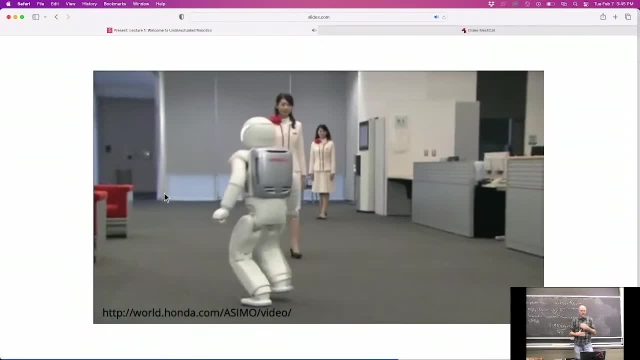 Okay. And ASIMO was just doing absolutely amazing things. It got better and better and more dynamic. It can run to some extent. 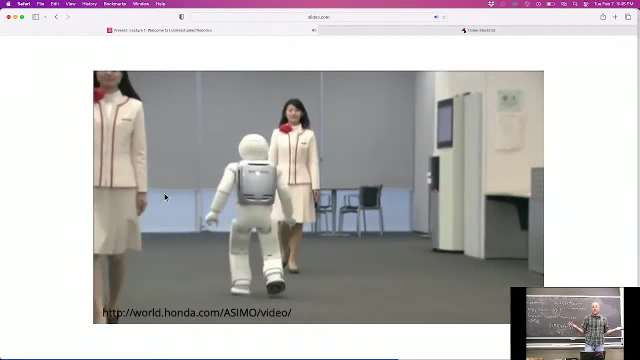 And we've seen the evolution of those kind of ideas up to what, I think, Atlas is really the pinnacle today. 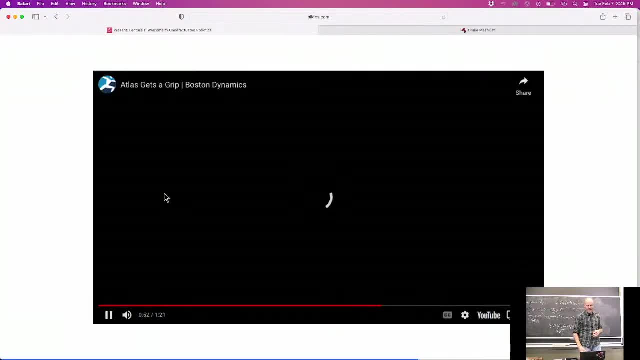 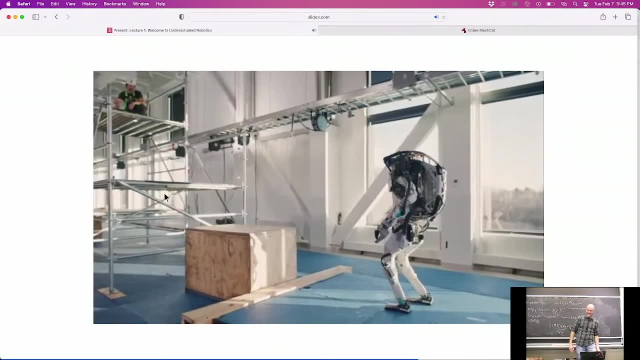 Okay. And this last move on the most recent video, oh, that's so good. That is so good. 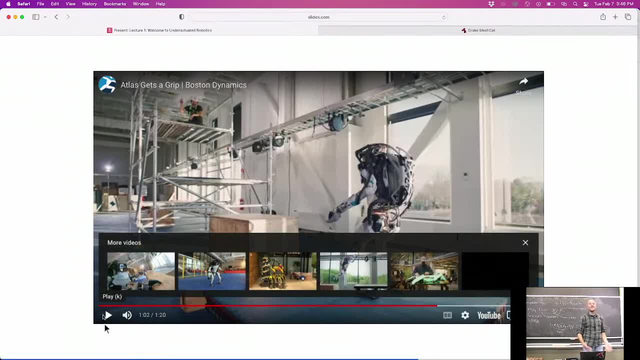 Yes. Okay. So that's the journey, right? It's going from rigid things, fully actuated, better control, using optimization, using dynamics, all these things, and getting to do like cool kickflip stuff, right? Yes. What is the journey? What is the journey? What is the journey? 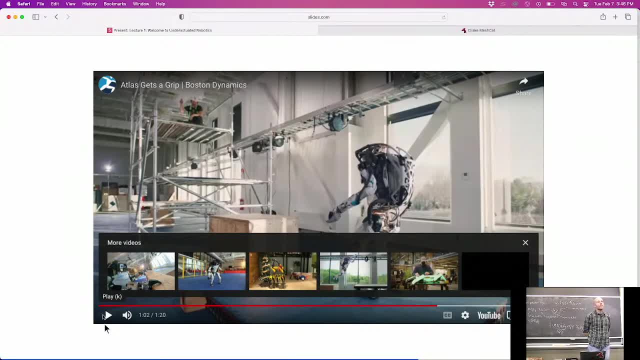 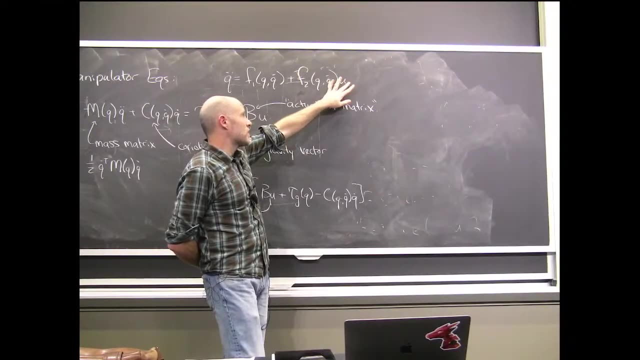 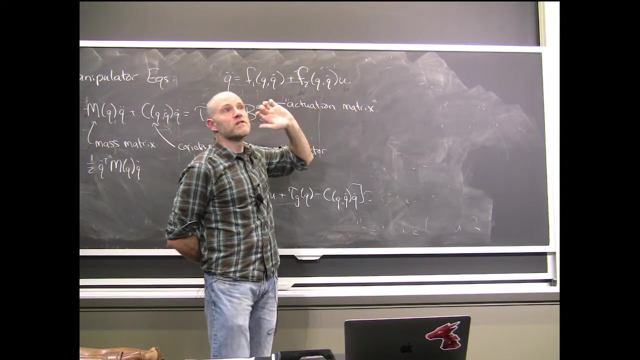 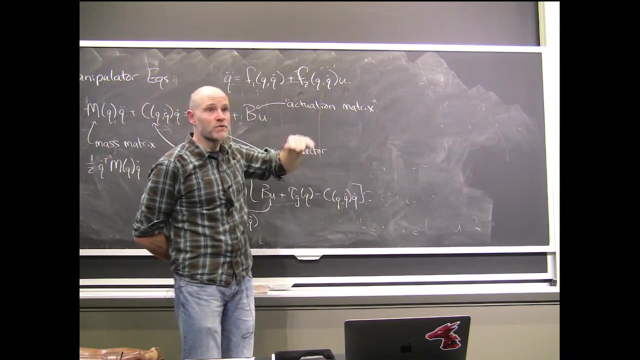 Yeah. No, it's, they're pretty darn robust, right? So I think the, one of the things that happens in a lot, in some of the practical applications is if you start having, if you don't have torque control of your joints, then you might have an actuator input. So like, for instance, on a plane, you're controlling the flaps of a, you know, and you might have other aerodynamic terms or other things that could add to the, still it has a fundamental manipulator equation, but you might have more terms that have less of that structure. 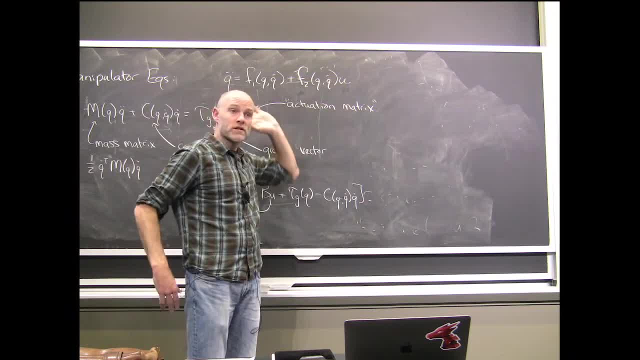 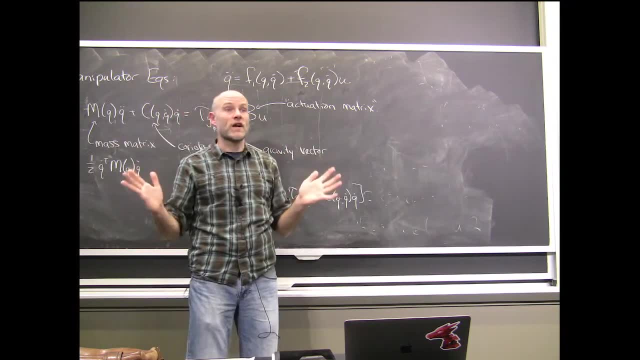 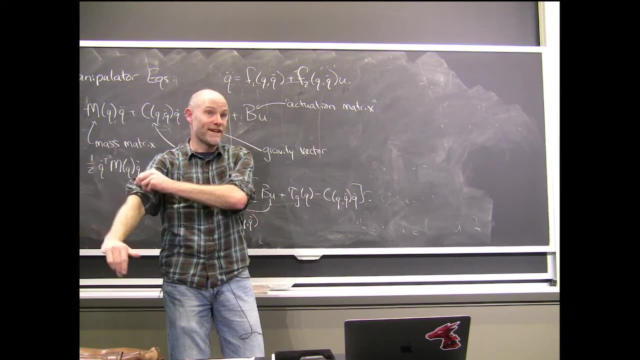 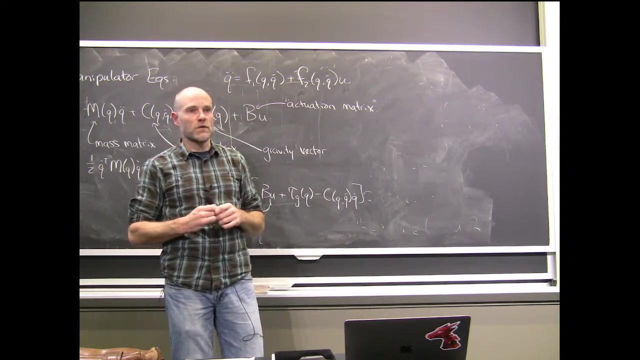 Okay. But, but even the way that the control affine works can sometimes break down if you have like velocity controlled or position controlled actuators. So you would tend to try to cut that at the control affine piece if you wanted to, or have to embrace the, the loss of control affineness. Yeah. But it's surprisingly robust. Most of these things do fit into that equation, that set of equations. Basically everything you can put in the dynamics engine, you know, roughly fits in that. Why does mass matrix take in Q? That's a great question. 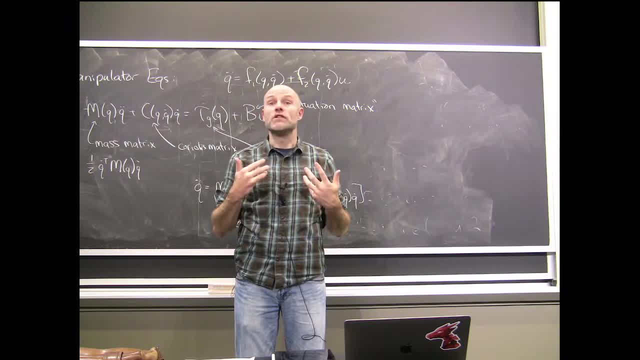 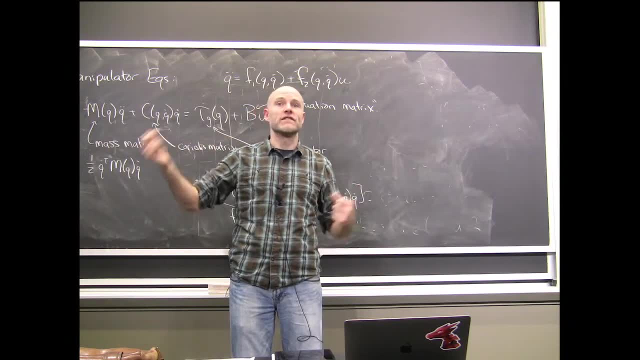 So think of it maybe as even the inertial matrix. So clearly the mass of the robot, the total mass doesn't work, but the effect that mass has on different joints is a configuration dependent thing. Okay. 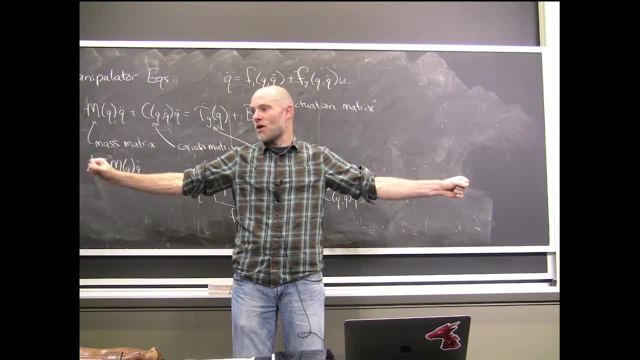 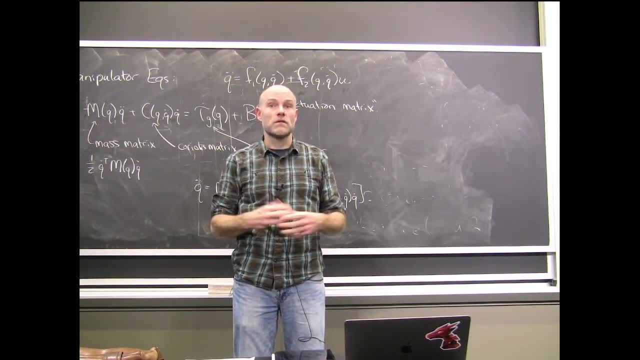 So for instance, you know, small torques when I'm like this will affect me differently than small torques when I'm like this. Just the position of my arms will affect, right? So it is a state dependent quantity. It doesn't depend on velocity, but it is state dependent. Yes. 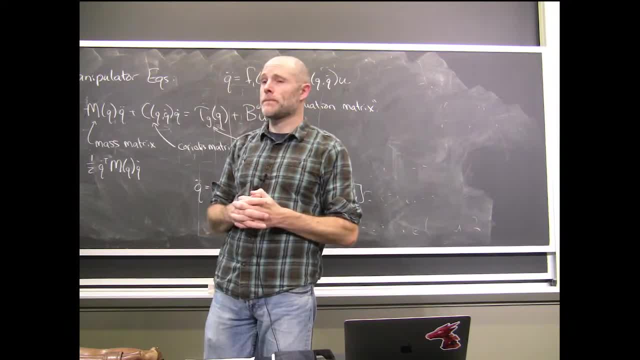 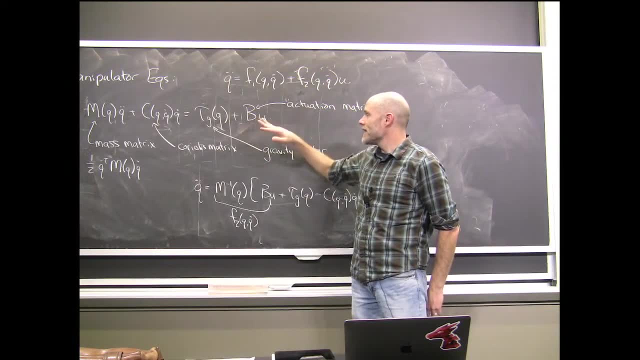 What exactly, what's the actuation matrix capturing or representing? So in many cases, it's, you can just think of it as, so in a simple case where you have one joint per actuator, 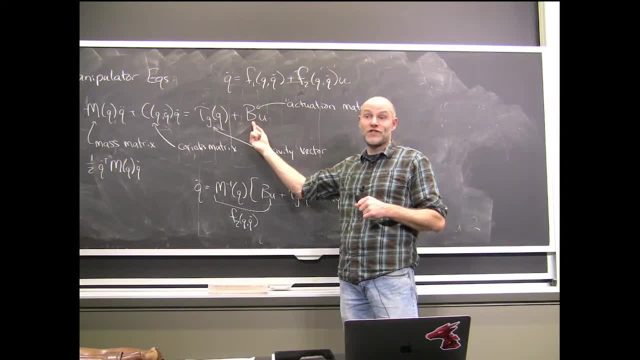 then it's just calling, it could be a selection matrix that are zeros or ones saying which joints have actuators. 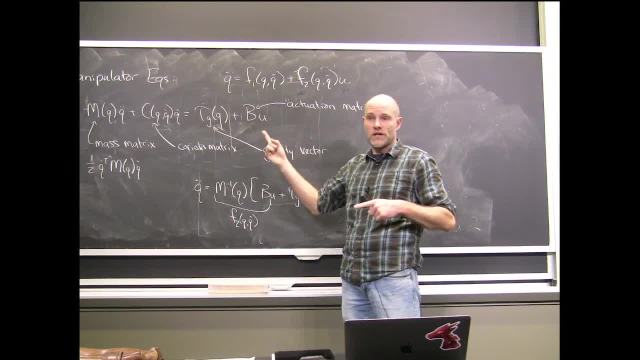 When you have, you know, differential drives and stuff like this, it gets more interesting. But in the simplest case, just think of it as a selection matrix. 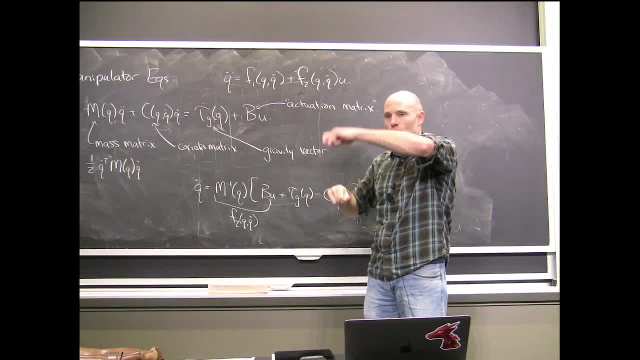 If you had more complicated linkages connecting your actuators to the joints, then you could potentially, you could bury more of that complexity into the B matrix. But oftentimes it's just a selection matrix. I love it. Yeah. Yeah, sure. I would put that elsewhere. 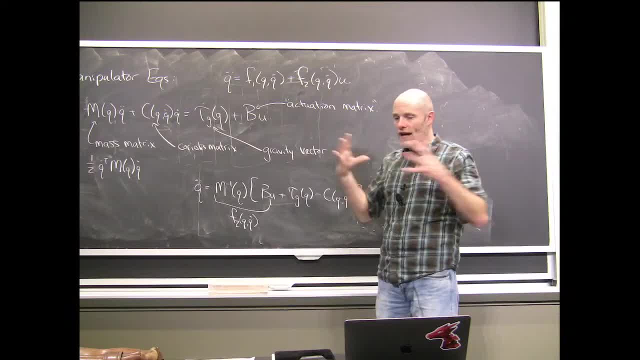 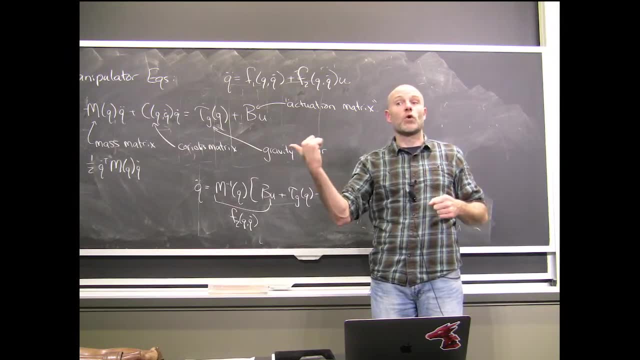 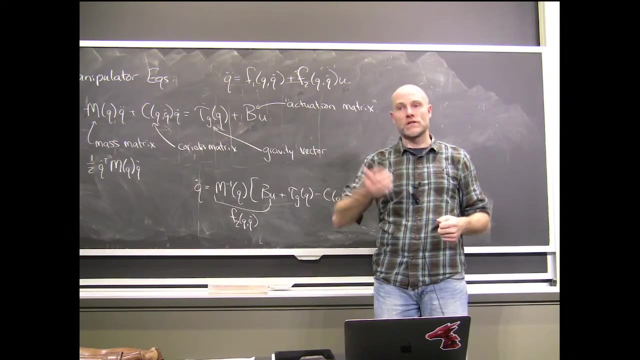 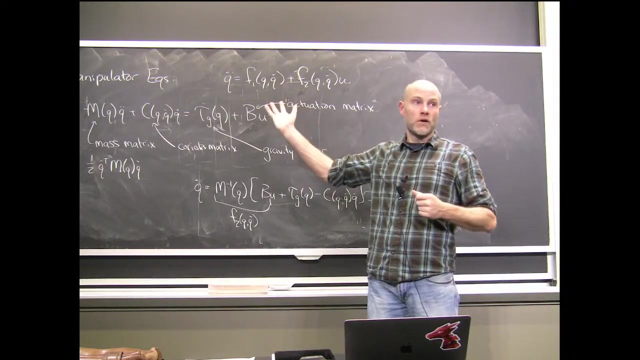 So in our modeling toolbox, we would think of an actuator model as being another dynamical system that has its own potentially internal state. And its role is to say, what are the torques I'm producing on the mechanics? At this point, and that's a port now on my mechanics module, which takes torques in, right? But you can build up more and more systems. That's another place where if you start combining more systems that you could break the manipulator equations form. Awesome. 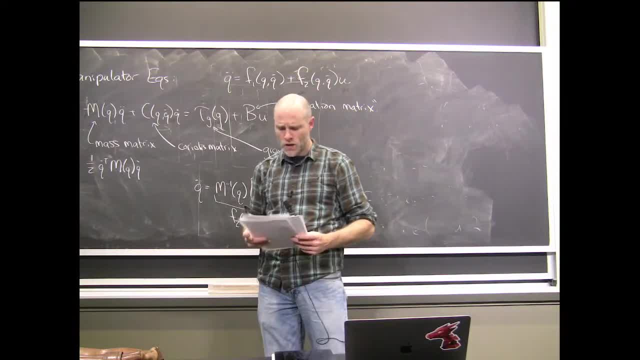 Okay, so let me, let me sort of summarize what we're going to do in the class now that I gave 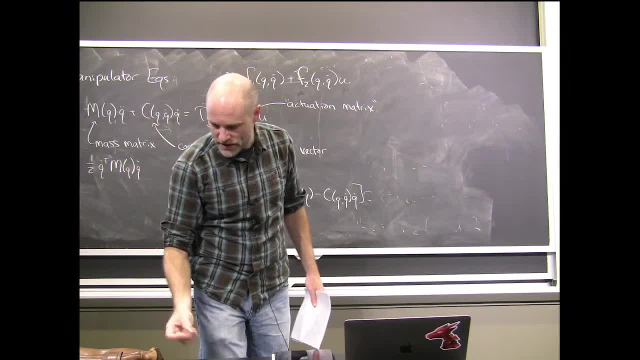 a few details and some, some high level. I'm going to hit my chalk for myself. 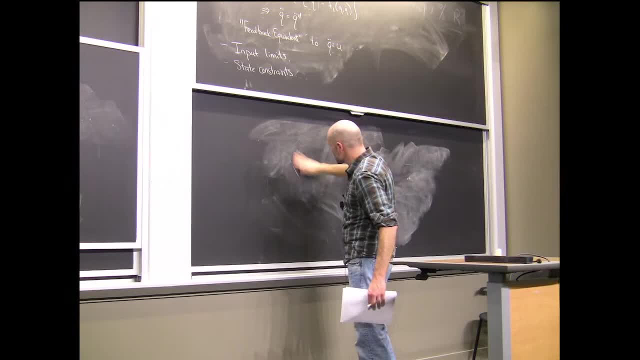 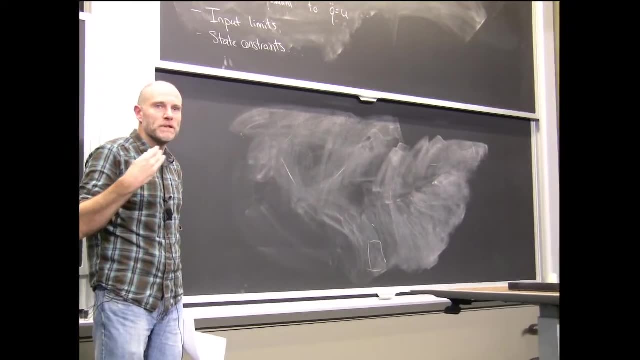 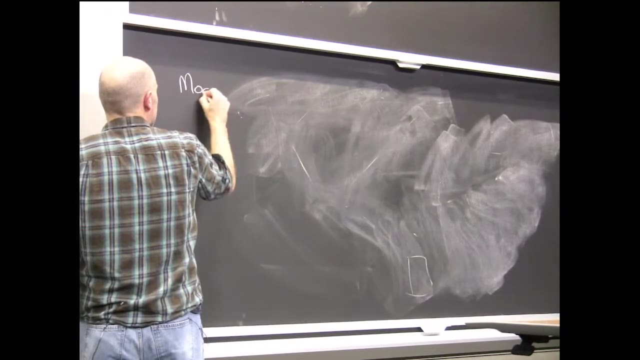 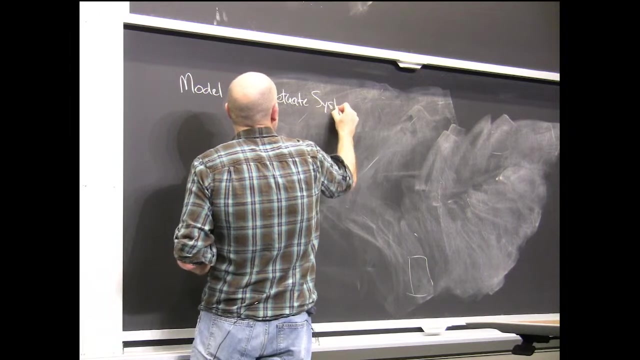 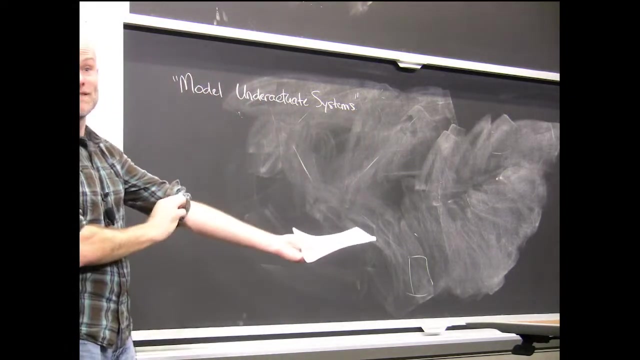 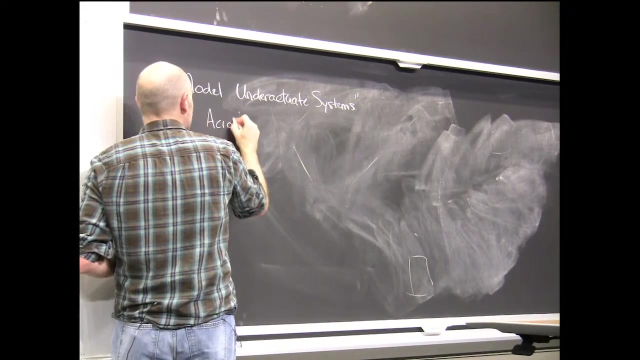 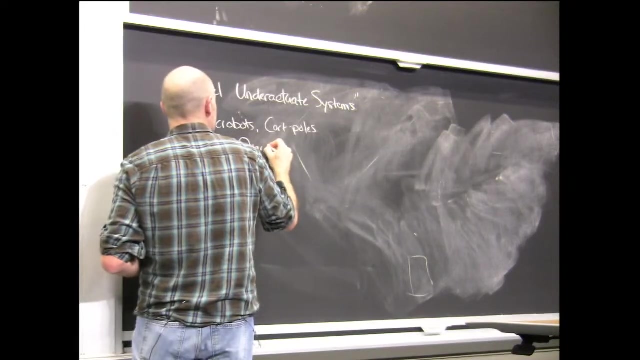 So we're going to talk about control, optimization, dynamics, learning, but in a way that is trying to, I want to do it by building up a toolkit, okay, where we're going to start with really simple robots. We have, there's a set of systems that we call the model under actuated systems. There's a kind of a canonical set of tasks, which you've seen maybe in the open AI gym or other things. These are like the acrobats, cart poles, pendulums, quad rotors, all fit in these systems and they all are relatively low dimensional state spaces. They have 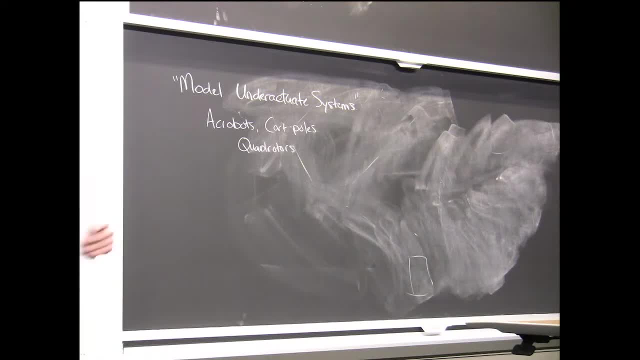 fit directly into these equations and we have lots of things to understand at that sort of core level. 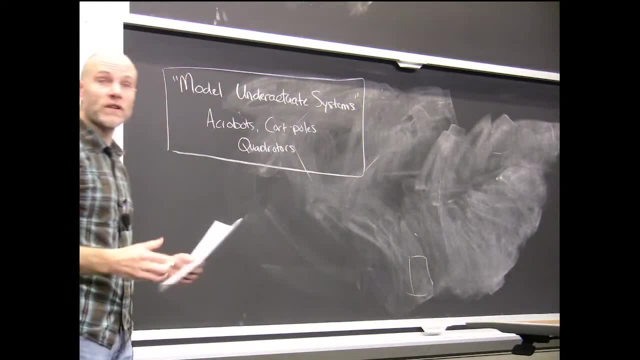 So we're going to look at the state of the art of controlling those kinds of systems first, and then we're going to spiral out into more and more complexity, right? 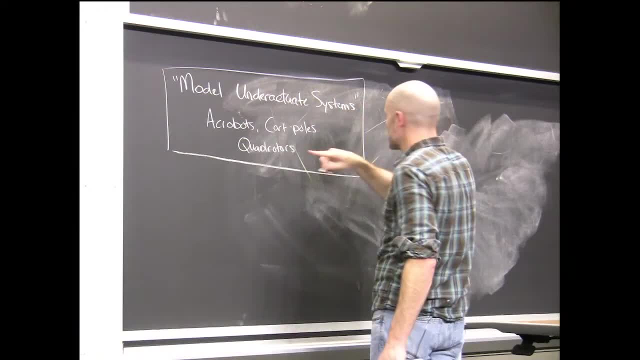 So when we start talking about even quad rotors that have to fly around obstacles, you know, we're, we're going to think about more interesting geometries. 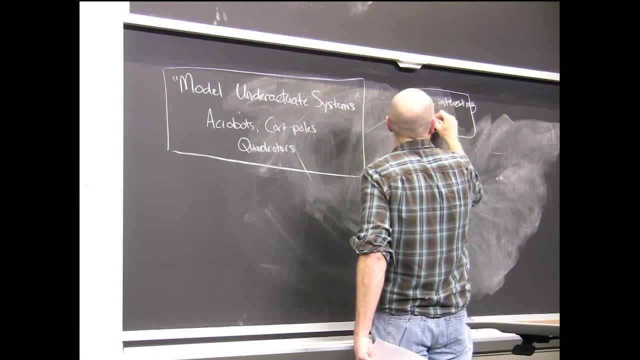 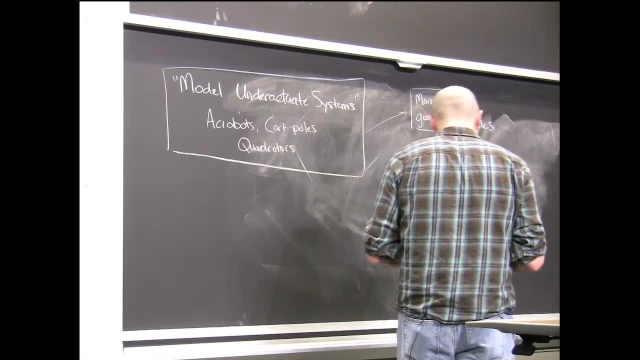 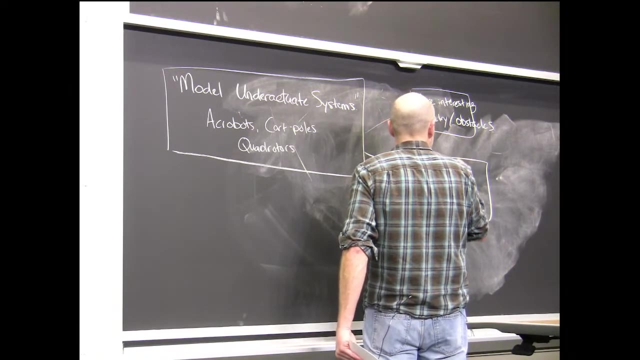 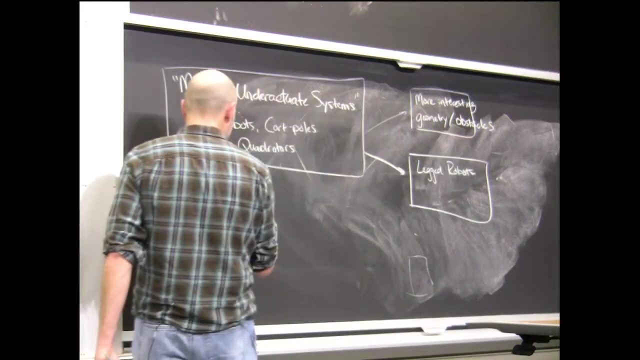 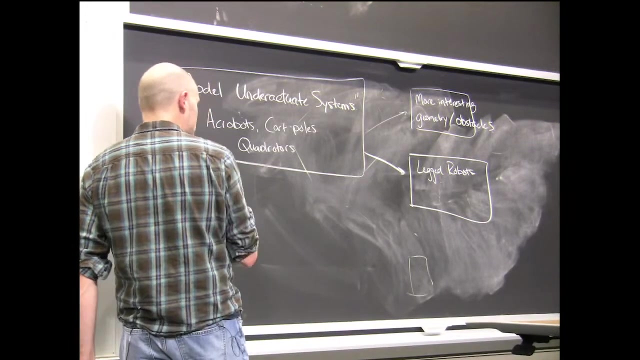 We're going to spend some time thinking about walking robots, legged robots, and actually there's some model systems like this. I mean, so the, the double pendulum is kind of a canonical one, the cart pole. We're going to look at the way that those things are distributed using the technology of machine learning and all of that. It's a very simple way to think about things like that. All right. We're going to have very simple systems like this where I can write the equations of motion on the board. 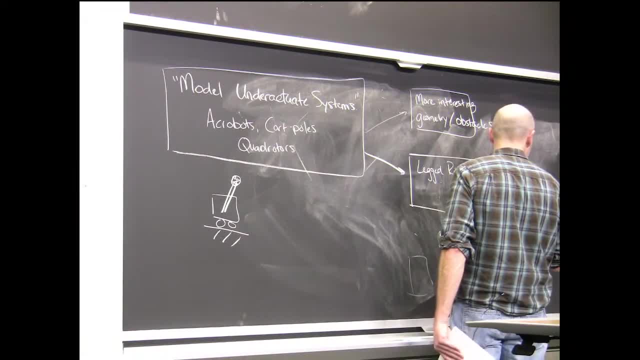 Turns out there's some very simple legged robots that are not so different, actually. 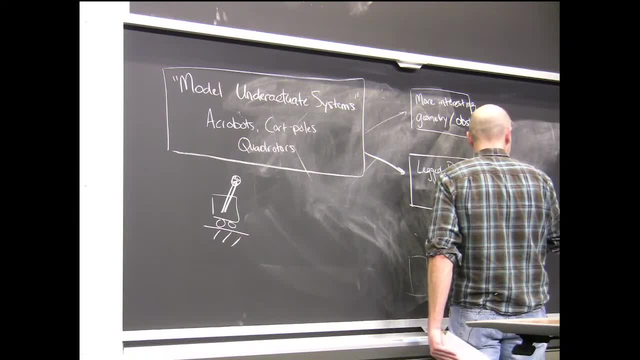 That double pendulum equation is a perfect model of one of the simplest walking robots, which is actually just a double pendulum that walks down a ramp and acts like a passive dynamic walker. 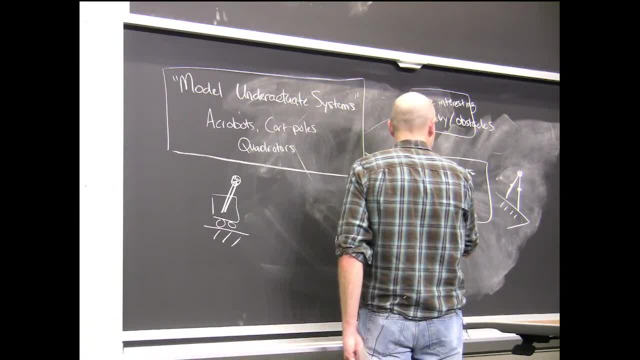 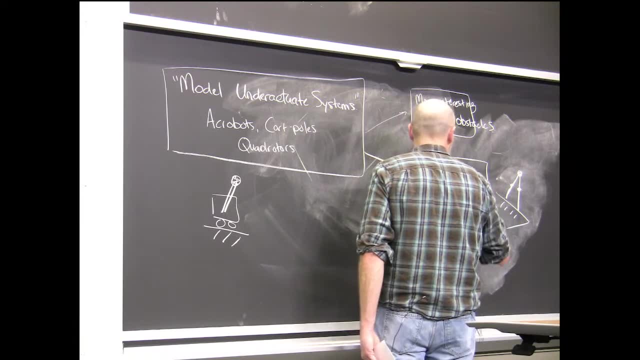 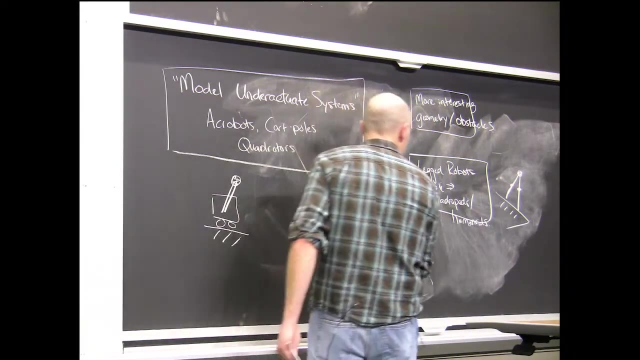 Okay, so we're going to start with that, both the simple, and then we'll get to quadrupeds and humanoids. Okay, we'll do a little bit, I'll even mention manipulation and how that fits in here, 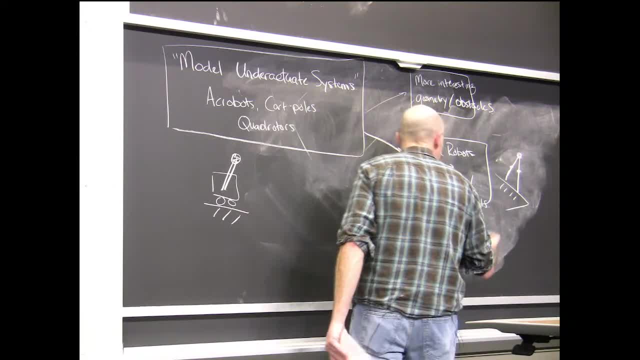 but we now have a whole separate course on manipulation, so I won't spend much time on manipulation in this course, even though I love it. 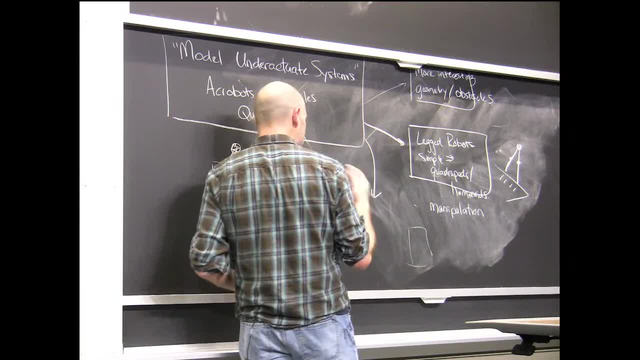 Okay, and then we're going to do more things to make the system richer and harder. So we'll make things stochastic. You know, partially observable. 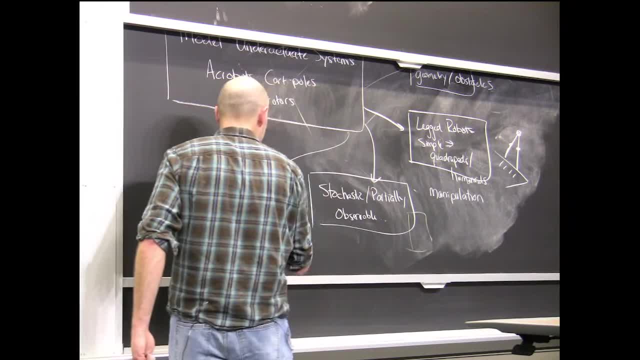 Okay, and then at the end, we'll think about things that are difficult to model. 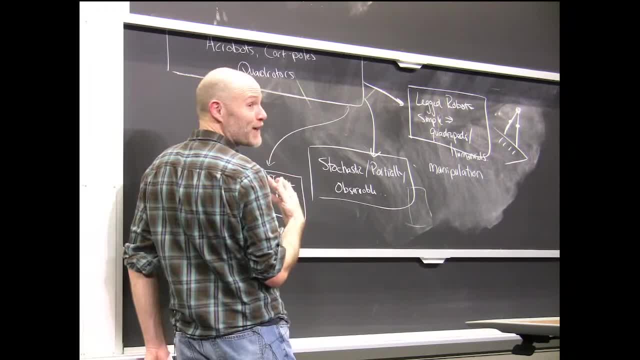 If we get to it, but like aerodynamics, hydrodynamics, things like this. 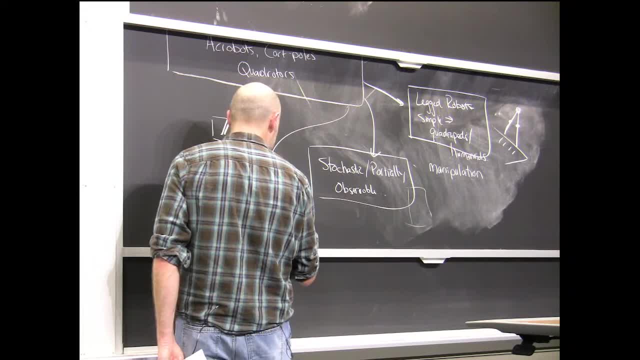 So, yeah, I'll draw a fish. Okay. 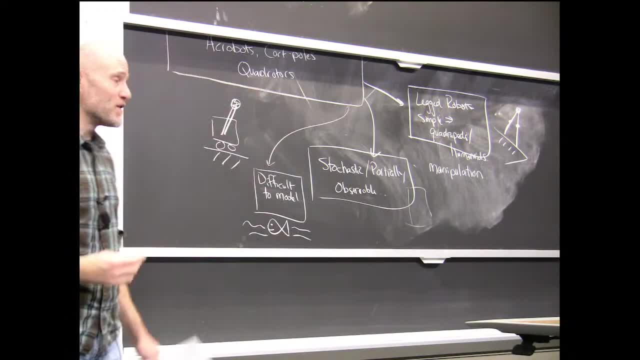 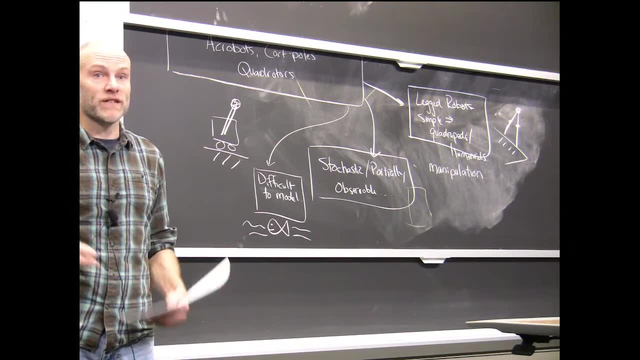 Difficult to model systems where we have to make more approximations of our dynamics and maybe don't expect to be able to just operate directly on the governing equations. They're just too complicated. 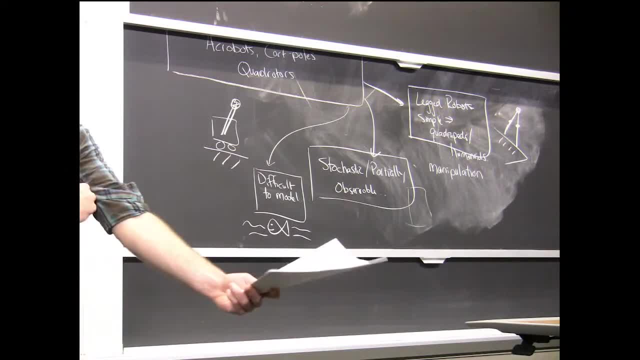 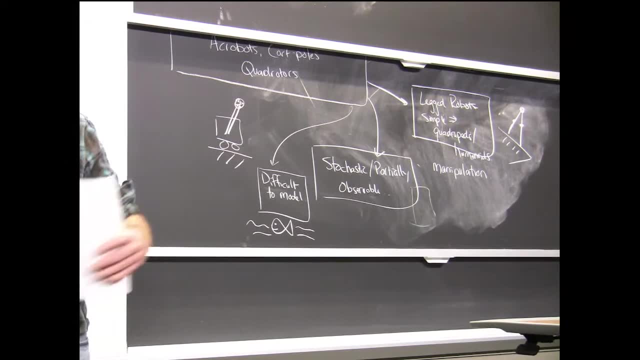 And throughout the course, I'll try to touch base on the optimization perspective. There's so much to understand in the world of optimization and the way it plays out. 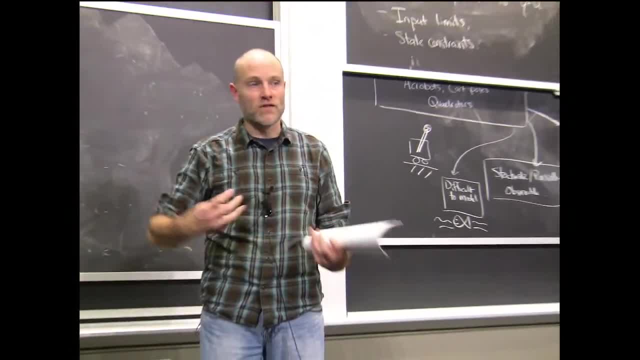 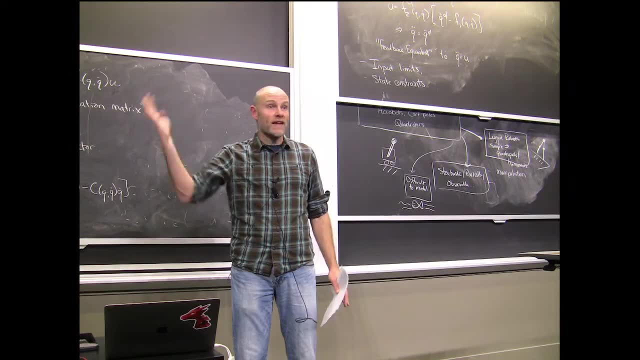 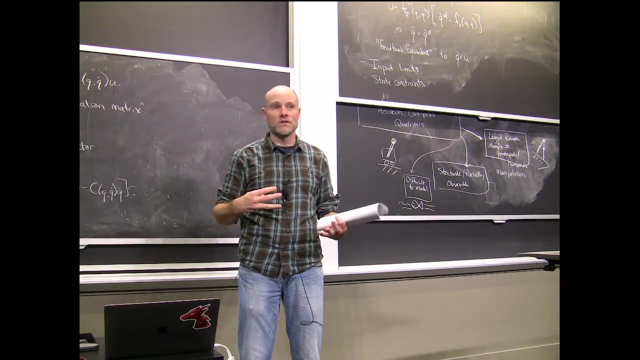 And I think that's the crux of all of this. I think there's all kinds of new stuff happening in machine learning, in particular learning theory, and how that has been changing the conversation. It controls people growing towards learning theory and learning theory growing towards controls. We'll try to bring those in when it makes sense. Yeah, I hope it's a good ride. So please go to the website. Sign up for Piazza. We'll post a few things. 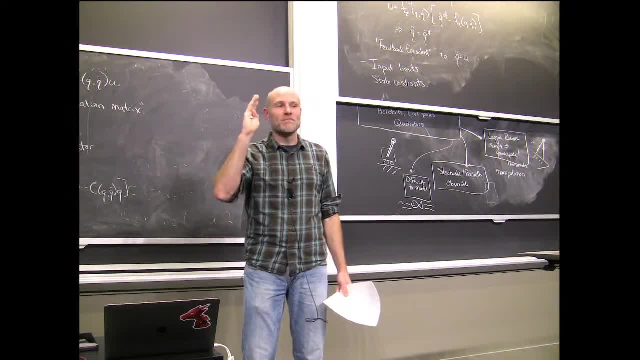 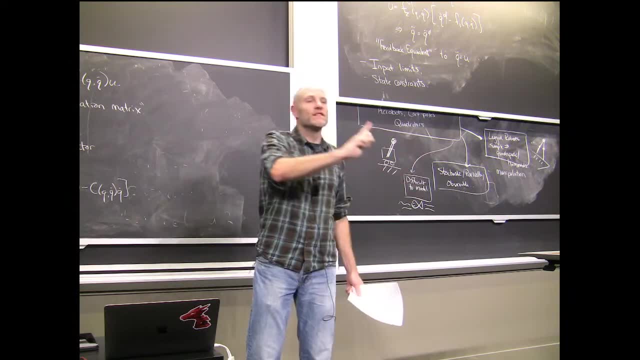 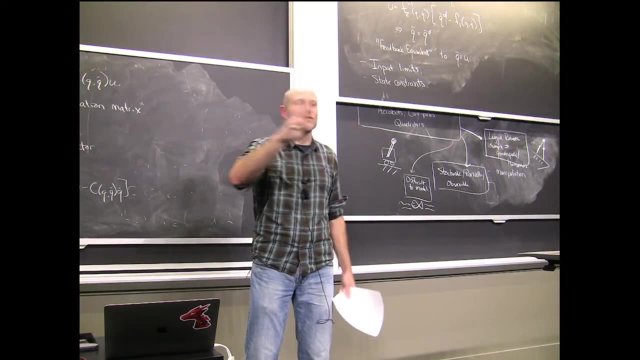 One thing I want to say to David. So the midterm was on the calendar at one day the other day, and then I found out that was Passover, so I moved it by a day. So if you looked at the date of the midterm before, it moved by a little day, and we're trying our best to make it work for people. So look at that soon and drop me an email. If that's... If that's a hard problem. I'll see you next time. Yeah? Yes? 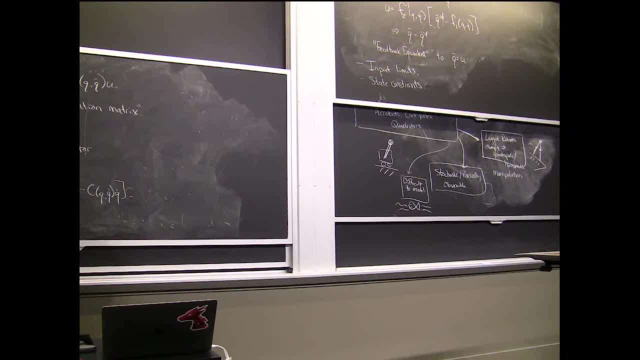 Which of the absolute states are fully actuated? It sounds like it's the position. 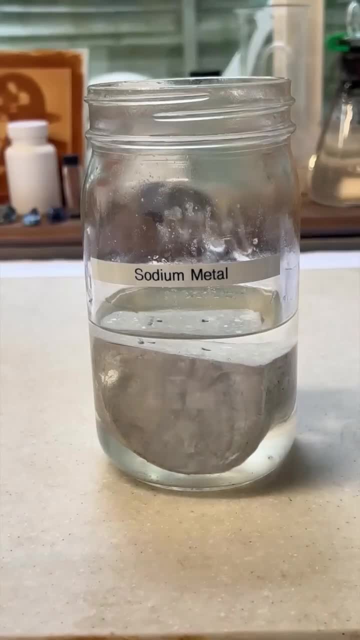 This is sodium metal. It's not like your normal metal. It has a few weird qualities. 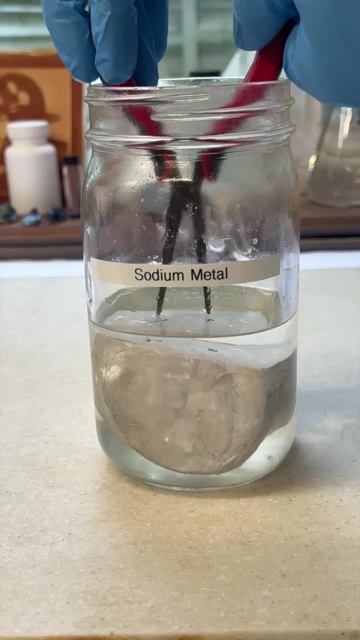 Firstly, it has to be stored underneath oil or it'll react with the air and moisture in that air.